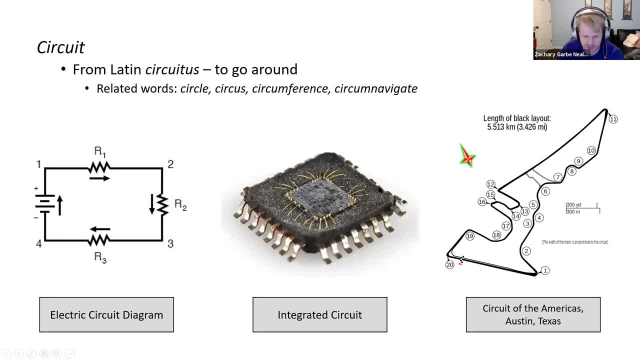 see, you know I'm sure many of you have seen like the full component, but I didn't know before seeing this how small they actually were on the inside, And most of it is much just packaging and the actual chip itself is much smaller than that. And then here's another example of a circuit that's been cut away and you can see the integrated circuit inside the microchip. And these are semi-conductive materials, diodes and transistors on that microchip. And these are semi-conductive materials, diodes and transistors on that microchip. And these are. 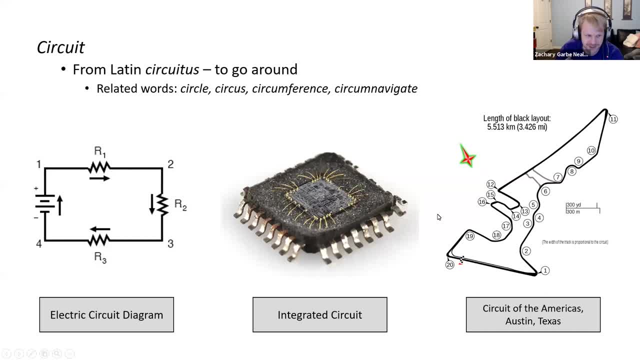 circuit of Americas is a race course. So just to go with fit with the definition of circuit, it means, you know, to go around. there's many other ways we can use the word circuit, not just for electronics. but there's a another type of circuit not related to electronics. 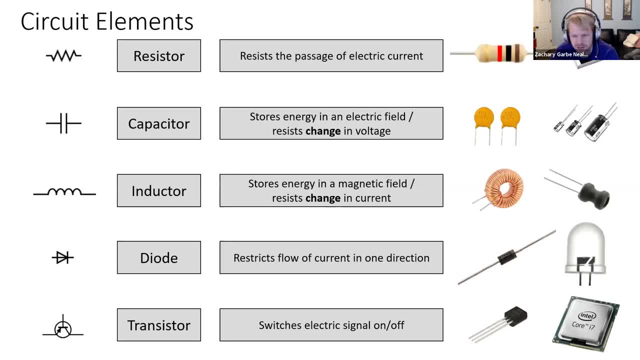 So let's go over some common circuit elements. So there are many different types of elements that go in the circuit, but these are just some of the most common ones And we'll deal with some of them today. Most common, probably the most common one, is the circuit of the circuit. 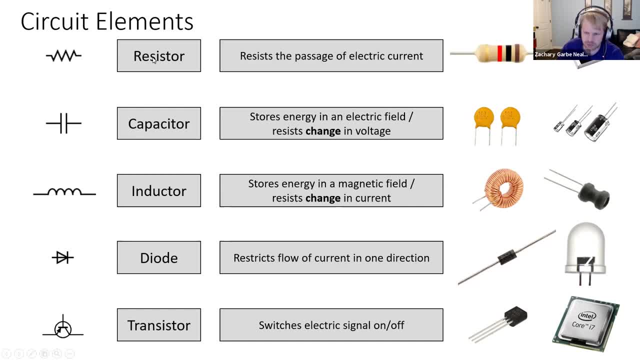 Most common probably is: the resistor is a passive element. the resistor will resist the flow of an electric current. Okay, so many resistors kind of look like this that you're familiar with and they have these different bands, different colors and the different colors and the different. 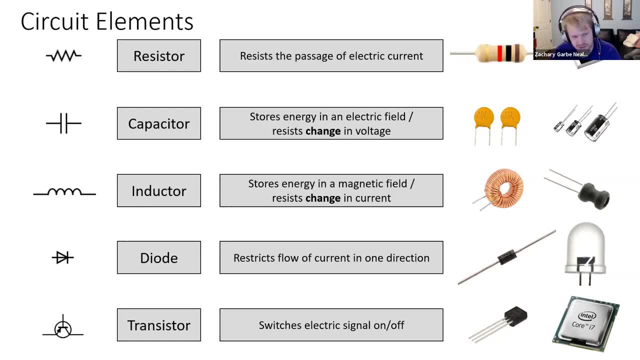 bands. they indicate the resist, the resistance of the resistor, And there's a chart that you can find that they can tell you which colors and which bands will will tell, will tell you the value For for. for myself I'm colorblind, So it's very difficult to actually see like differentiate. 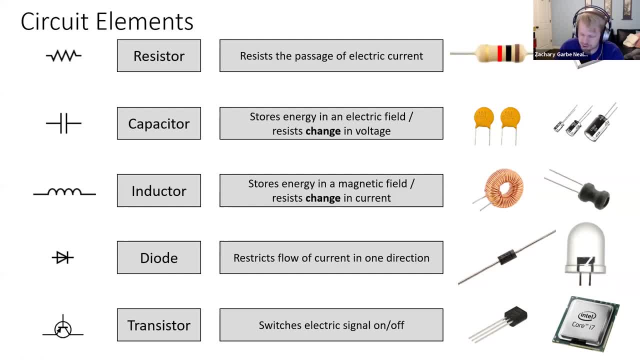 between red and green, I think, for I've heard for electrical engineers, the people that are colorblind have a fairly difficult time because a lot of electrical engineering deals with these color coordinated systems And there's other types of resistors. These are like surface mount. 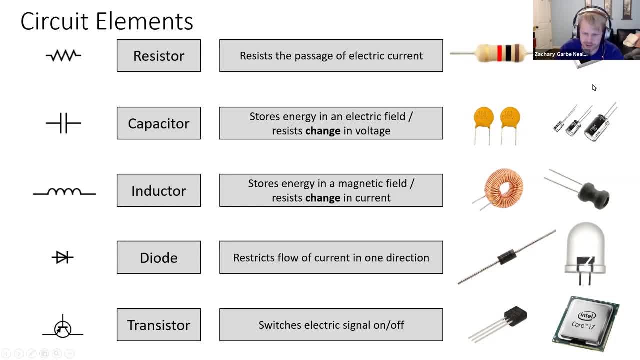 resistors are smaller profile that you can put on like a circuit board or solder on. Next element is a capacitor. So a capacitor stores energy in an electric field. It also, once a electric field has been built up in the capacitor, it will resist a change in voltage. So, for example, if you had a 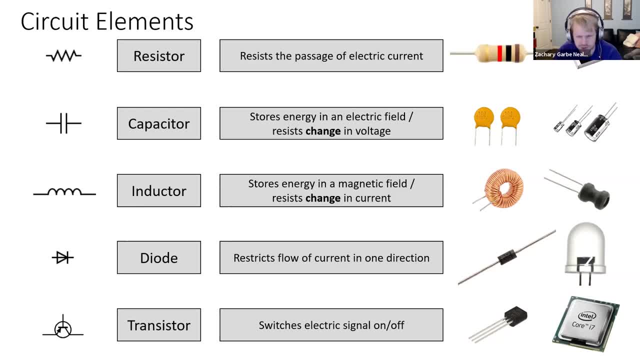 circuit with a capacitor in it and it's been charged up and let's say, you switch the circuit off or you break the circuit, the capacitor will try to maintain that voltage by discharging its, its energy, for a bit of time. So that's, that's a capacitor, Also important to point out. 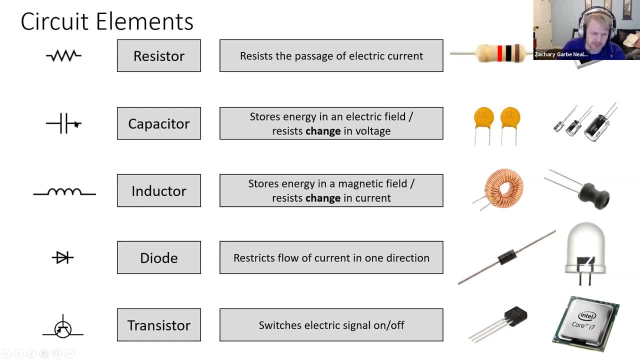 that current cannot flow through a capacitor once it's been charged. So it's a, it's a break in the line. you could say: except for AC current you can pass an alternating current between a capacitor, but not not a direct current. An inductor is just a wire that has a lot of coils. Inductors store energy. 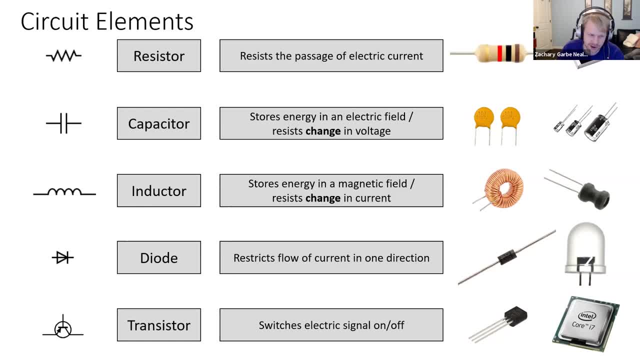 in the form of magnetic field And they similar to capacitor they. but instead of storing electric field they store magnetic field And they resist the change in current. So if we had a circuit running at a certain current and then we break the circuit and cut the current off, the inductor will try to supplement that lost current. 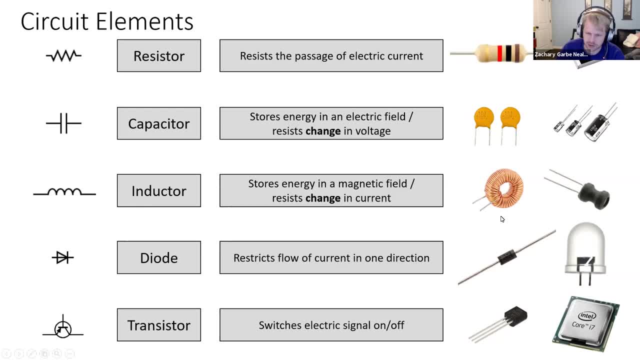 by discharging its energy, its stored energy. So they look like these wrapped coils, usually wrapped around a, I believe, a ferromagnetic material making the solenoid, and they can come in different shapes. Oh, I forgot to mention the capacitors. there's different types of capacitors, So these are: 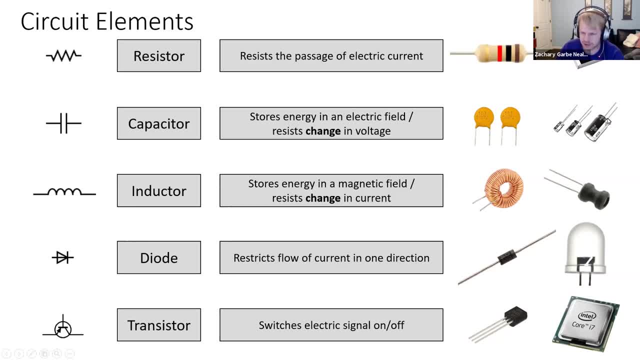 like ceramic capacitors, and these are electrolytic capacitors, where the electrolytic capacitors usually are polarized. So there'll be one side that has to be the negative side, Because these, these are inside the these capacitors. there's like a electrochemical reaction that's taking place And it 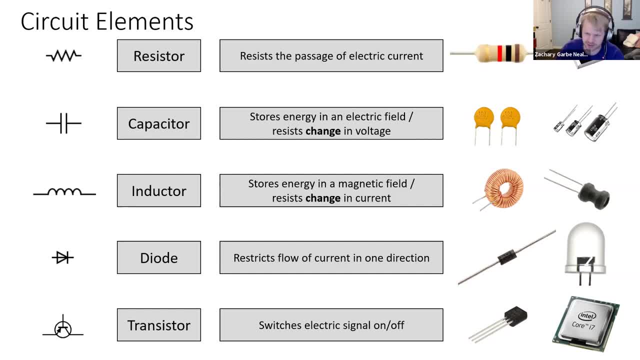 can only be in a certain positive, either positive potential or negative potential, that it can't be the reverse potential. It's just just similar to like a battery: you can't can't just flip the battery, turn it around and it's going to putting a negative voltage across the battery. would would ruin it. 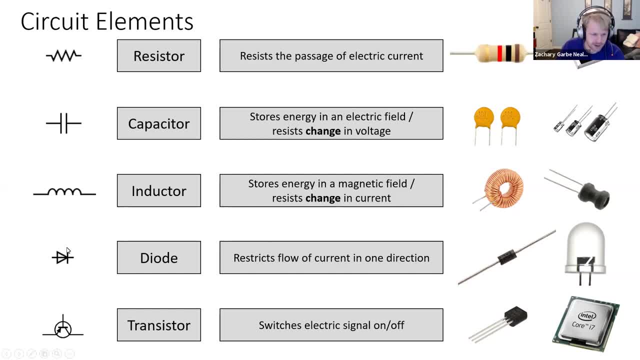 Same with these capacitors, And then a diode. a diode, diodes and transistors are semi-conductive devices. So a diode is actually a combination of two semiconductors, an n-type and a p-type semiconductor, and its function is to allow current to flow in one direction through the circuit. 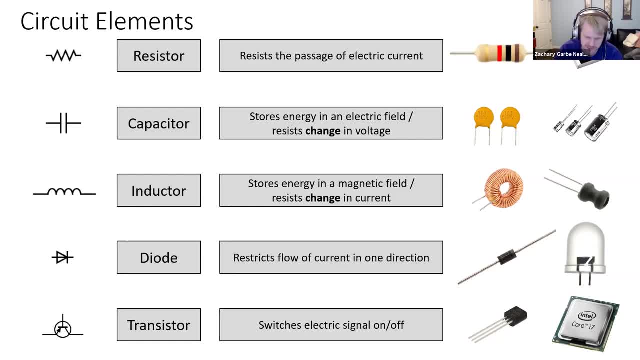 but it does not allow current to flow in the other direction, So it's going to be a negative voltage and it's going to be a negative voltage across the battery and it's going to be a negative voltage opposite direction. So it's kind of like a a valve, a check valve, that just allows flow in one. 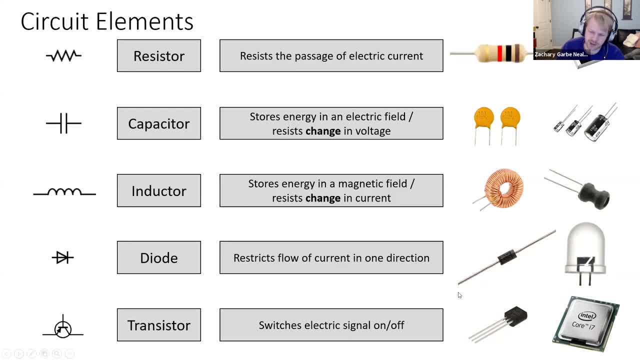 direction but not the other. So there's, you know, different types of diodes And in our labs the next week we will be looking at the characteristics of a diode. LED, a light emitting diode, is a type of diode And I'm sure you've you've experienced from our previous 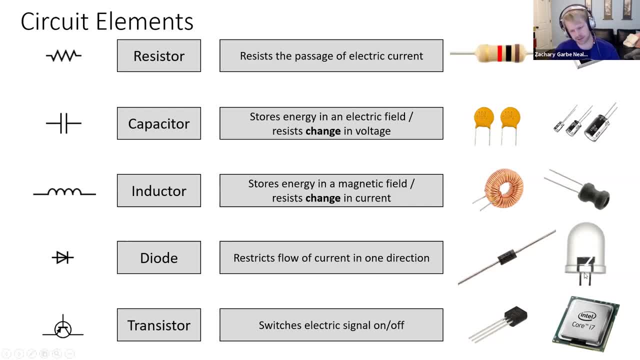 quarters when we work with LEDs, that the, the, the current can only flow in one direction. You cannot. you have to make sure the LED is in the right orientation, Otherwise it won't light up, because it's a diode. And then transistors again is another semi-conductive material. 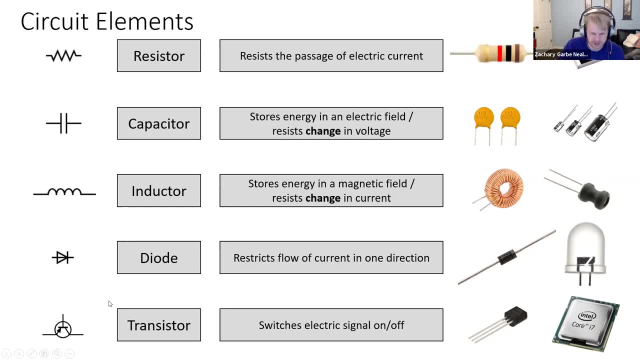 It's a combination of either a n-type, p-type material. We will be looking at a transistor. However, now that I remember, we're not actually looking- well, you'll see- but we're looking at the material inside the transistor, So we're not actually looking at the material inside the 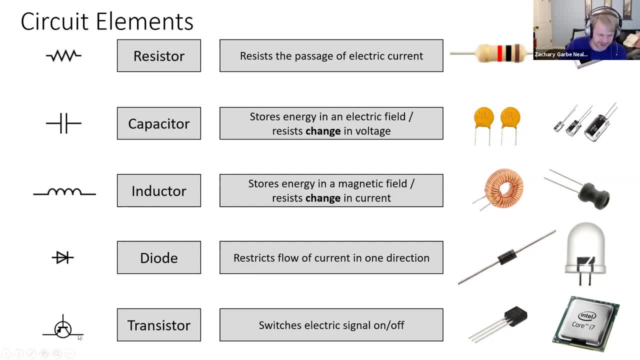 transistor and not like actual transistor itself. We're just looking at the transistor material And in any case transistors act as a switch, so they can turn a signal on or off. And this is the basis for all computing, because if you can have a switch that gives an on or off, 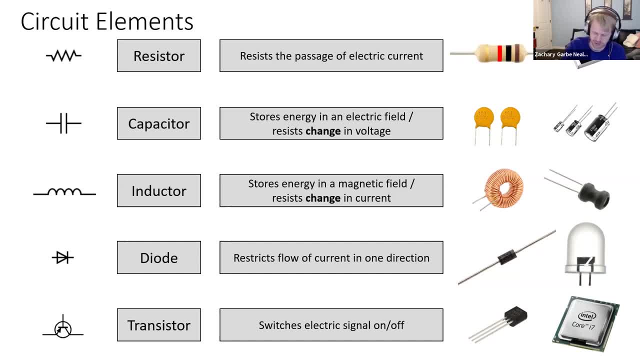 signal, then you can do all computation and base two math, And so all computers rely on transistors in order to make those computations. Before the invention of transistors we had something called vacuum tubes, And it worked in a similar way that it would deliver. 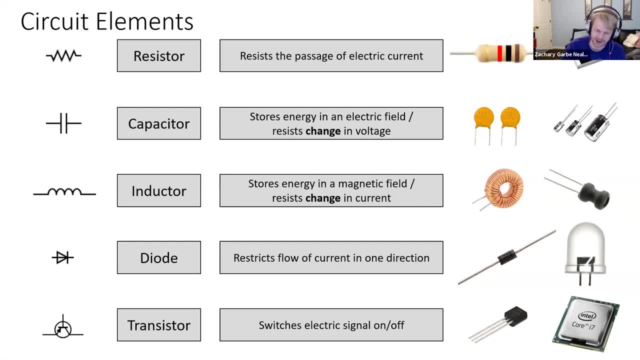 an on or off value. but they weren't compact, They were much bigger. It required a coil that would heat up this environment and emit electrons in one direction And then so it would allow the current kind of flow in one direction, not the other, so like a diode, Anyways. so since the 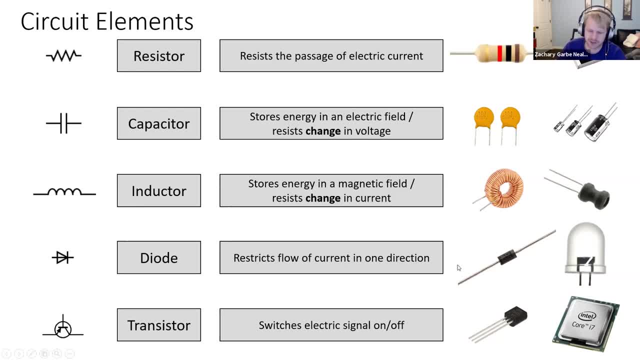 invention of the transistor, we can miniaturize these components, And so we're not actually going to do that, We're going to do a lot more, And an example of that miniaturization is in a computer chip. So this is an example of an Intel computer chip, a CPU, a central processing. 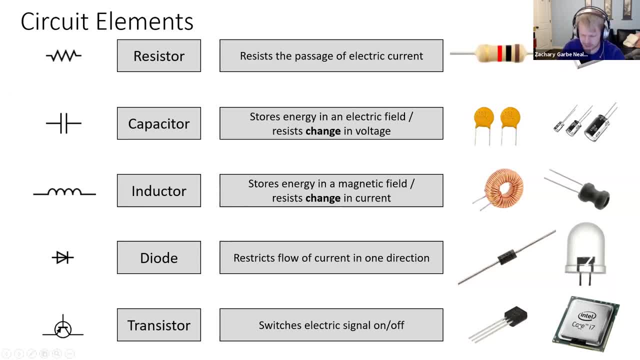 unit. So in all your computers and all your cell phones and everything that does computation will have a chip like this that does those computations, And inside the chip there are many transistors. Now I asked the morning class and I'll ask you guys too, oops, oops, sorry. How many transistors? do you have in your computer? And I'll ask you guys too, oops, oops, sorry. How many transistors do you have in your computer? And I'll ask you guys too, oops, oops, sorry, How many transistors do. 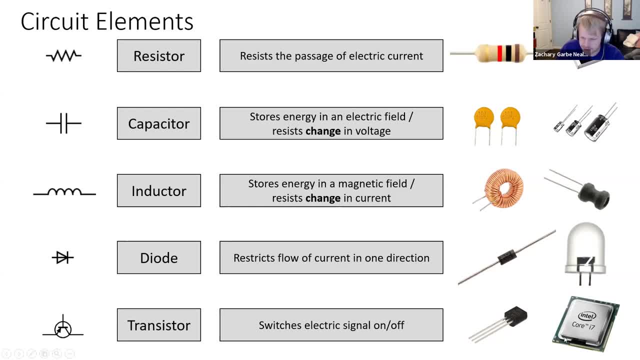 you think are inside one of these computer chips. So here's an example of just one transistor, but how many do you think are able to be put into your computer chip? or a ballpark estimate, How many do you think- And I have my computer- Say again: 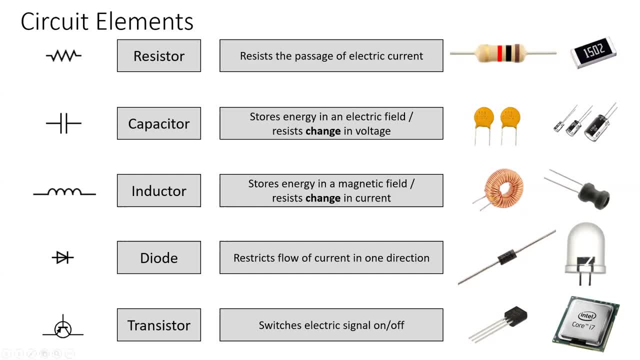 At least 10?, At least 10.. Yeah, yeah, I'd say that's correct. So, John, you say a billion, and, yeah, that's correct. There are billions of transistors inside your computer chips, And so, for example, I took the computer, the CPU chip that's in my computer that I'm using now. It's an. 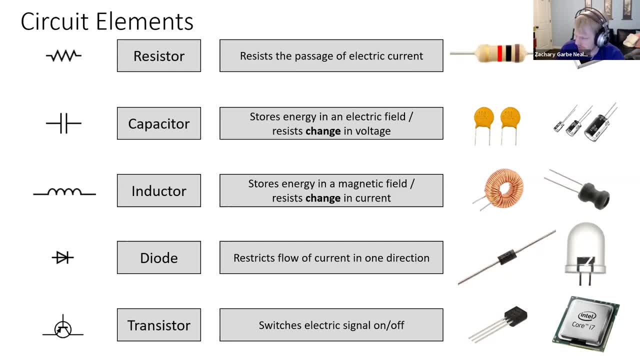 eight-year-old chip I got in 2012.. It's an Intel i5-3570 and so on, Anyway. so I looked it up and it has 2.1 billion transistors inside the chip, So that means it can make a. 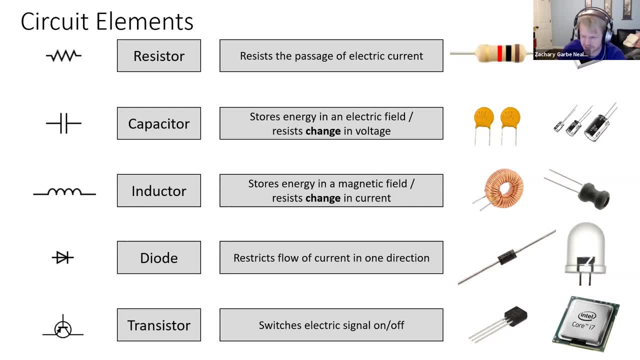 you know, the more transistors you have, the more processes you can have, and that increases the speed of the computation. And the transistor that's inside my chip. the size of the transistor is 22 nanometers And I think now today it's even smaller. It's like 11 or so nanometers. 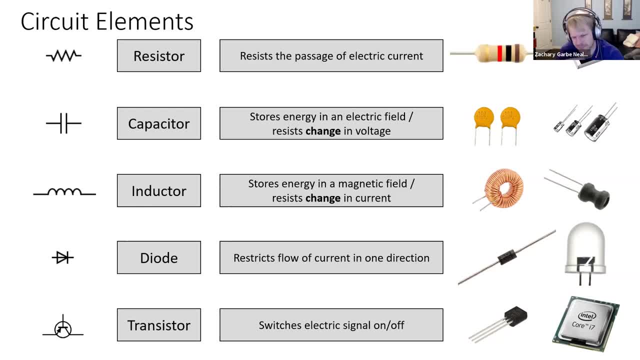 And so you know that fits that law. I forget what that law was called. If someone knows the law of the universe, it's called the law of the universe, So it's like you know what I'm talking about. they can blurt it out where, every year, the size of the transistor 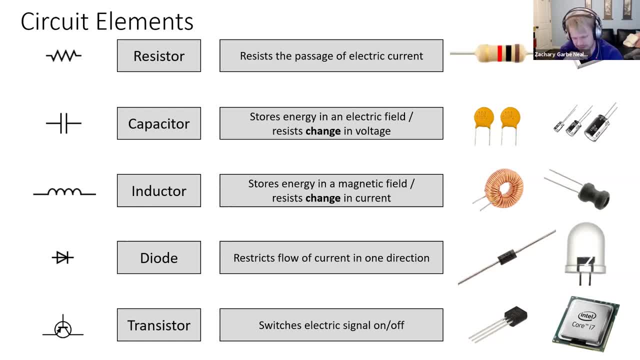 decreases. Moore's law, thank you, Yeah, Moore's law, So something, and I forget exactly what it was- but like every so often or every year, the size of the transistor decreases a certain amount and it fits some trend right Now. that's been true up until, I believe, recently, And the 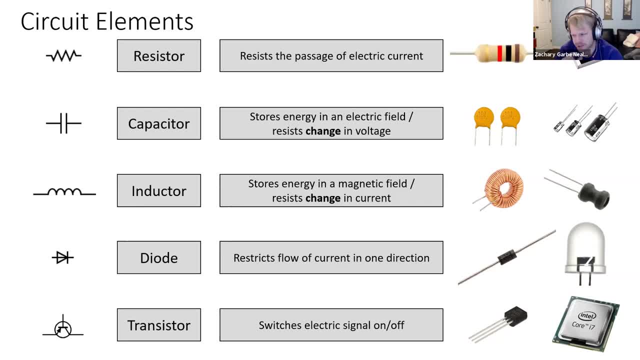 problem is there's a limit on how small we can actually make a transistor, And you guys know why. Why is there a limit How small we can make the transistor? I can think of actually two. Is it because of tunneling? 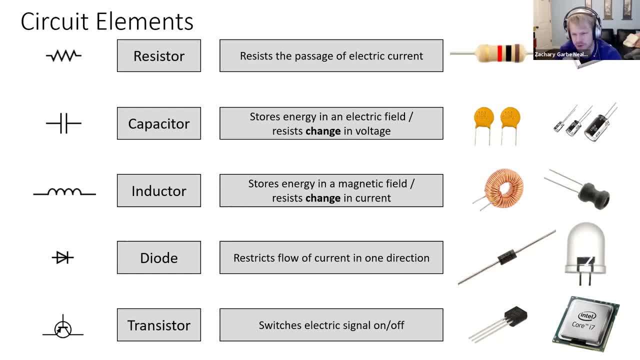 Yeah, One reason is tunneling, That's correct. So if you make something too small, you're you know. the purpose of the transistor is to stop current or stop voltage. yeah, stop current and then turn it on, right, It's a switch. But if you make it too small, you'll have electron tunneling. 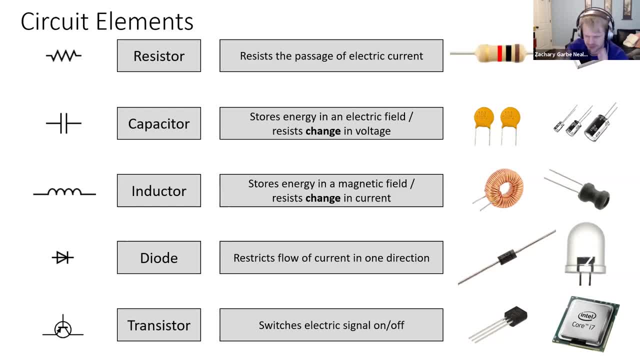 and it'll just go through without any- you know- switch involved. The other problem is the smaller you make these materials. remember, transistors are made of doped semiconductors, N-type and P-type doped silicon, And the order of doping is like one part per million or one. 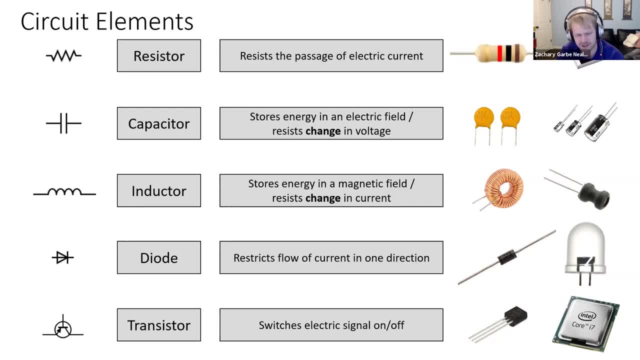 part per billion. It's a very small amount of dopant that's added to the material. And the smaller you make the material, the more crucial is the accuracy of the dopant right. So if you're making it really small, you only have like a million atoms in your transistor. 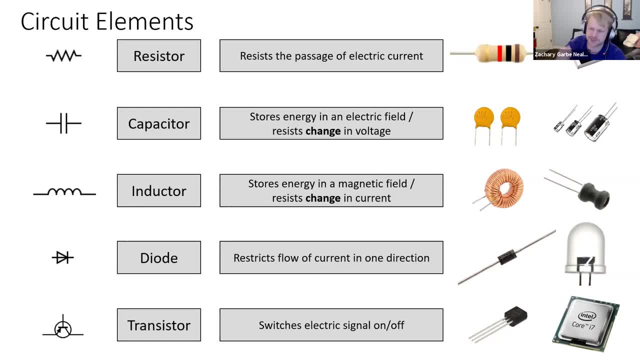 And so you can only put in one, you can only substitute one or put in one dopant, And so it's easy to you know mess that up. So on a smaller scale, All right, let's move on. So talk about. 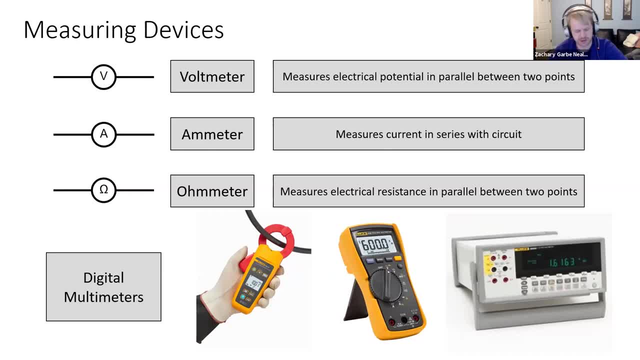 some measuring devices that are commonly used and will be used in our labs. So we have the volt meter measures, electrical potential between two points and in parallel to those points. So we'll talk a bit more about that. The ammeter measures, the current. 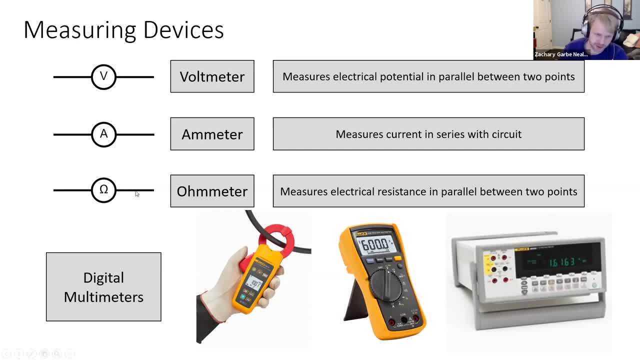 That's in series with a circuit. So a volt meter is in parallel, ammeter is in series, excuse me- And the ohmmeter measures electrical resistance, again in parallel. Well, actually, I mean really, ohmmeter would be really in series, but you shouldn't be using. 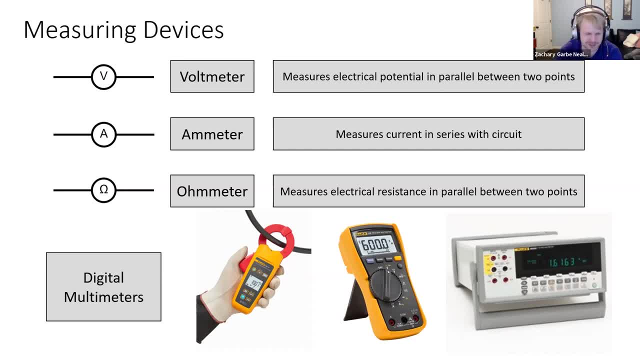 the ohmmeter as part of a circuit. It doesn't, I'll talk about later. But so these three things, they are three different instruments, right, There's three different mechanisms that in these instruments that would allow for these measurements. And you know, historically, 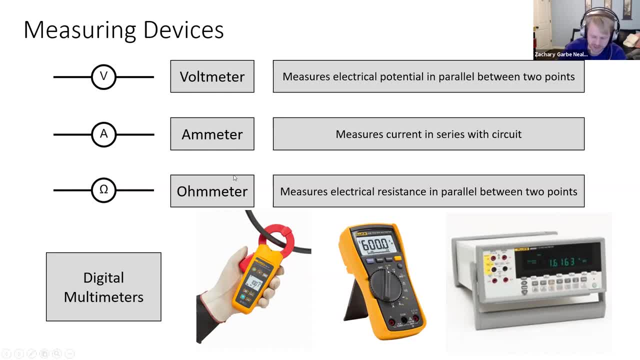 before digital processes, these were all like analog and they would have to have these three different. you would have three separate instruments for this. But now we have digital multimeters. I guess there's also analog multimeters, but digital multimeters that. 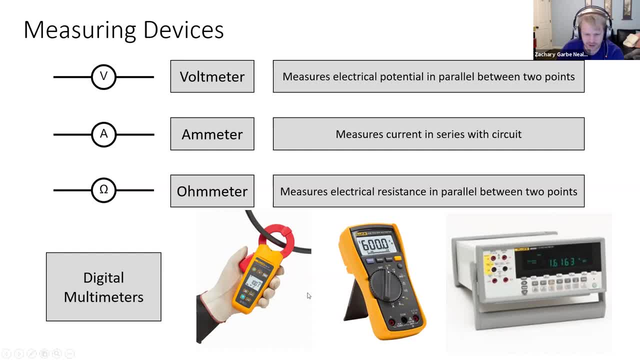 incorporate all three of these and many other things inside of them. So these are examples of some digital multimeters. So they can measure current, they can measure voltage, resistance and they can measure other things. Some of them measure temperature or light or capacitance, and 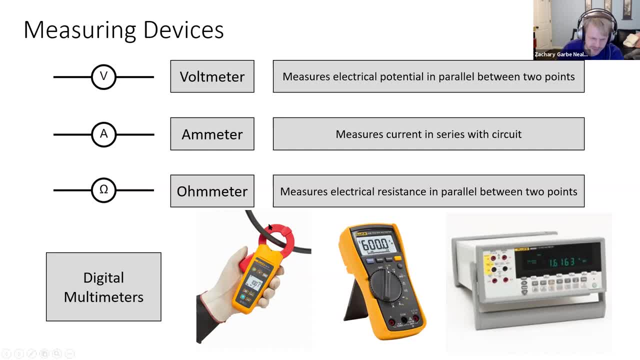 some other things. So you know, here's an example of like a hand clip-on one where if you clip it around a wire that has a current, I think, I believe through induction you can measure like the current or the voltage, which is quite handy for electrical engineer If you want to probe. 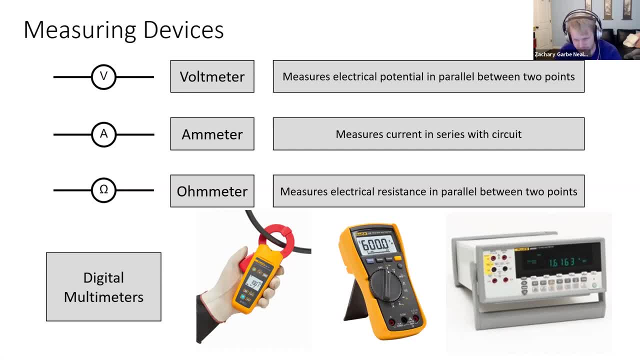 something and you don't want to make contact with the actual wire itself or have to find contact points to probe it. And then there's also, you know, desktop versions that are more sensitive, And so some of our labs will be using the desktop version for a four probe Kelvin clip measurement, And these are all made by the Fluke. 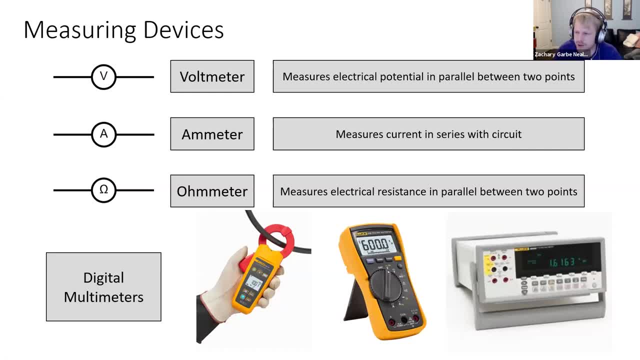 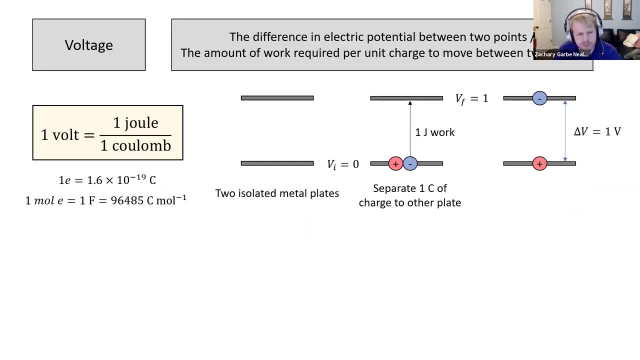 brand. Fluke is a very well-known brand, a very high quality brand of, and a rather expensive brand of, multimeters. So here's some definitions that we'll go over, And most of this you know, you should already know through like a freshman or sophomore physics classes. 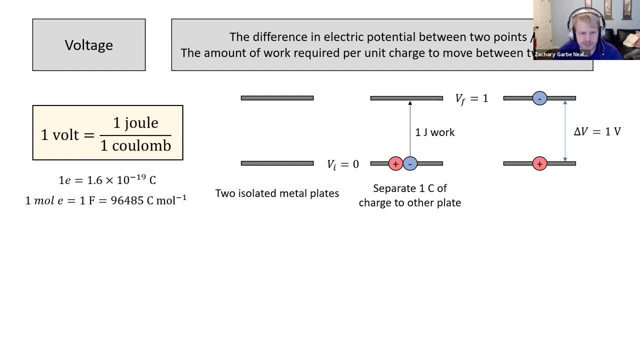 but just as a review to get you guys ready for next week's labs. So voltage is the deference in electric potential between two points. In other words, you know, it's also equated as the amount of work required to move one coulomb, excuse me, one unit of charge between two points. The units: 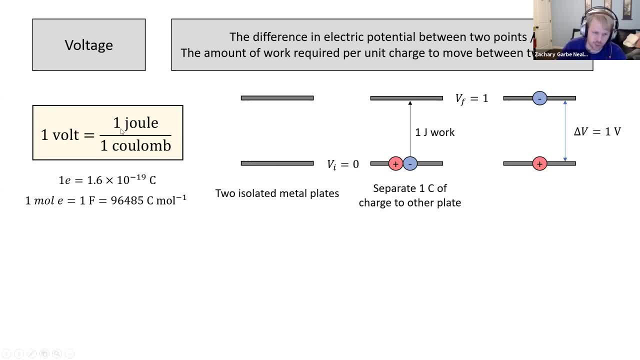 of voltage is the volt And that's equivalent, like I said, is one joule of work per coulomb of charge And if you remember, you know if you have an elementary charge which would be like a proton or an electron or a. 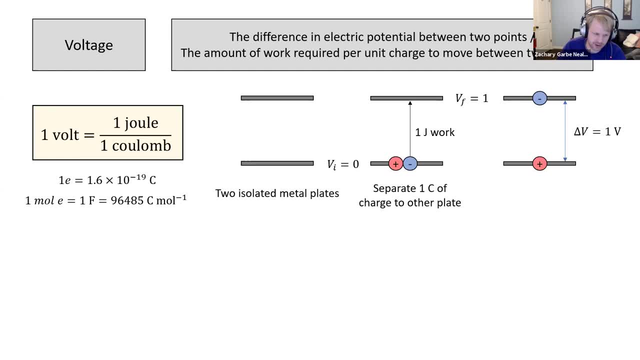 monovalent cation or anion. I have an elementary charge of one and that is equivalent to 1.6 and 10 to the negative 19 coulombs, And one mole of that elementary charge, so one mole of ions. 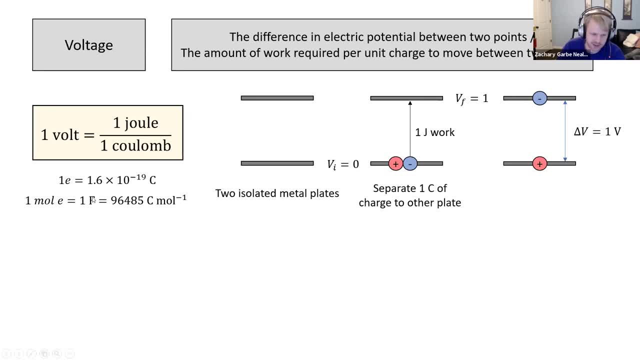 for example, monovalent ions is equal to one. this is F for a Faraday. One Faraday is a constant 166,000 coulombs per mole And it's important to distinguish. this we'll be talking about. 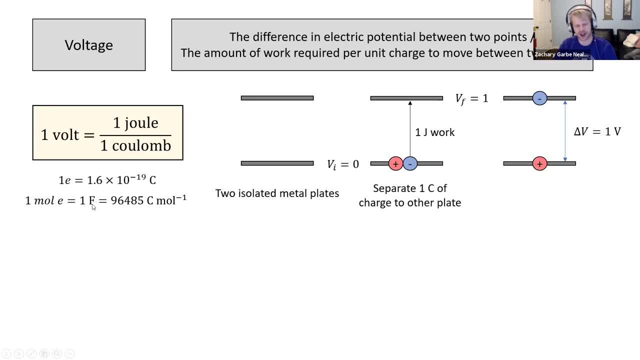 capacitance. later, Capacitance has units of Farad, which is different than this constant which is Faraday. Okay, so here I kind of give an example of one volt of potential difference. So if you take two isolated metal plates and they're conductive plates, I guess they don't necessarily need to. 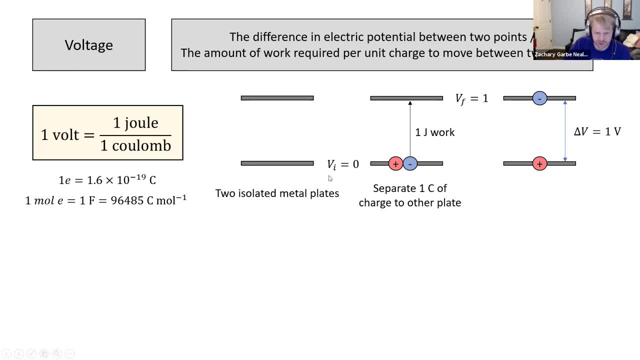 be conductive. but there are two isolated plates and by themselves they have a voltage of zero. And we were to take one of these plates, but we would not go to the other input and we would only go to this one. So when you take one of these plates, you have a voltage of zero and you have a voltage of one. so 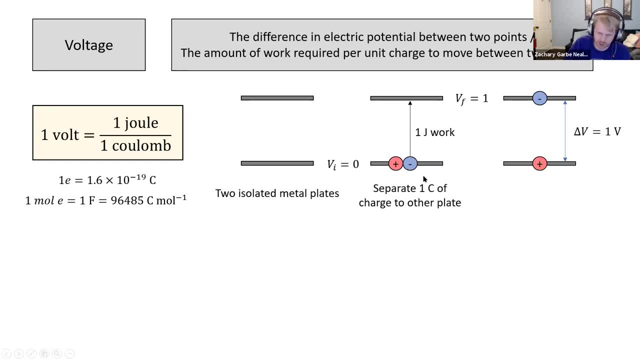 one unit of charge or, excuse me, in this example, one coulomb of charge, and we were to move it to the other plate, or rather separate it from its, its neutral state on one plate, and let's suppose that took one joule of work. if that takes one joule of work to move one coulomb of charge, then the 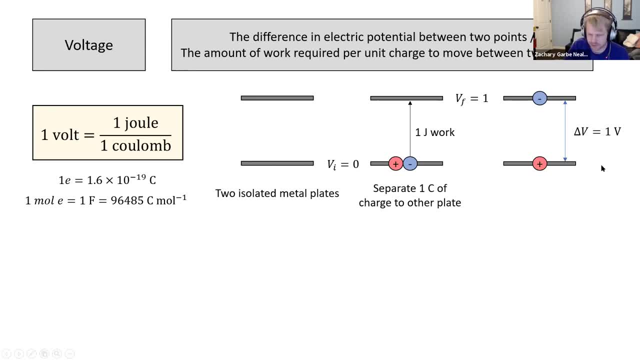 potential difference between those two plates is one volt. it doesn't matter how close the plates are. if it took one joule of work to move it, it's going to be one- a potential difference of one volt between those two plates. so you know what. what could be doing that work to move that charge. 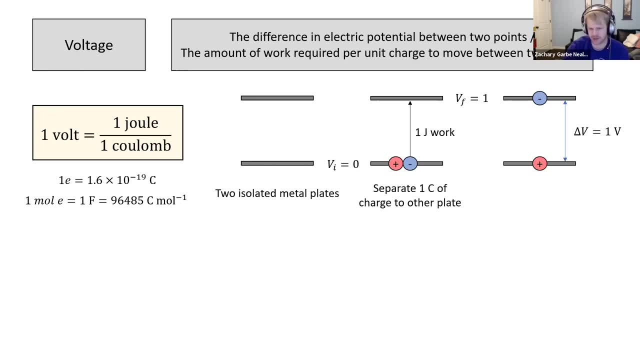 you know it could be a electrochemical cell or like a battery, could be what moves, or like has that potential difference to separate that charge. so an analogy that's often used with voltage and other definitions is a water system. so imagine if you have a water tank. 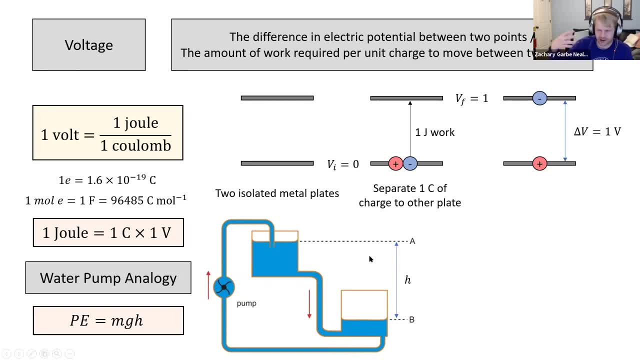 two water tanks that are connected and one water tank is at a higher elevation than the other, kind of like a dam and a reservoir of water right there's a potential energy for the water at the higher level to flow to the lower level right, so that potential energy is analogous to the change. 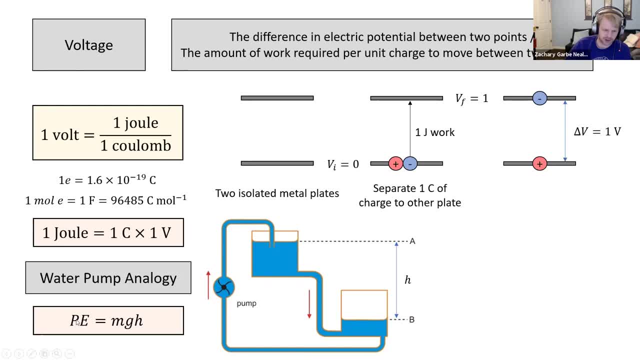 in potential voltage. that is. so here I have to demonstrate: potential energy is equal to the mass times, the gravitational acceleration times, the height, and I rearranged this equation so we say one joule of work or one joule of energy is equal to one coulomb times one volt. okay, so in this 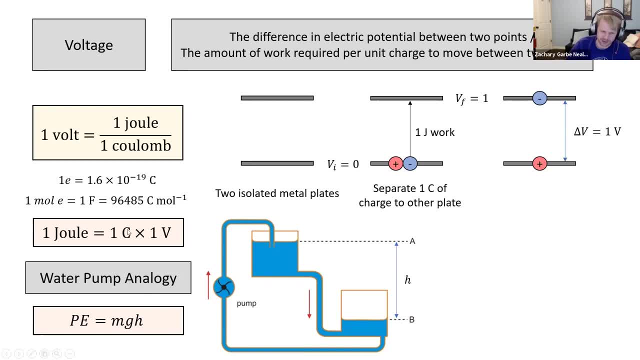 analogy, you could think of mass times, acceleration equivalent like to coulombs, and then voltage is analogous to the height of the system. okay, and then in this, this example, we have a pump that's that take those inputs the work. and then, in this example, we have a pump that's that take those inputs the work, and then 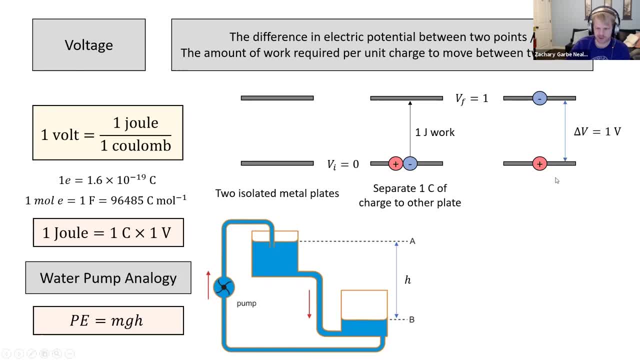 the work to move the water back to the top of the system. that which could be analogous to, say, a battery in a circuit that could, you know, put some charge at a higher potential. okay, so that is voltage. now let's look at current. so current is the net flow of electric charge. 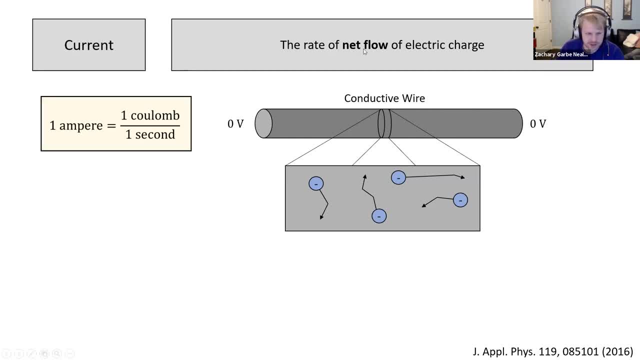 and I want to emphasize that it's net flow and not just just, not just the speed or not just the, the movement of charge itself, but the net flux of of charge. it has the units of ampere. that one ampere or one amp is equal to one coulomb of charge per second. okay, so in this example we have a wire. 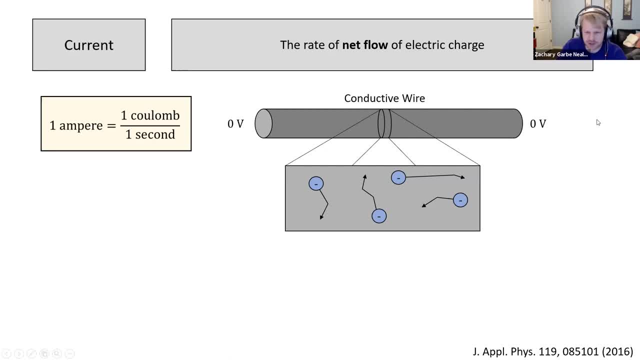 a conductive metal wire and there's zero voltage difference, there's zero potential difference between the two sides. so in that case, you know what is the the current? well, the current is going to be zero because there's zero potential difference between the two sides. so in that case, 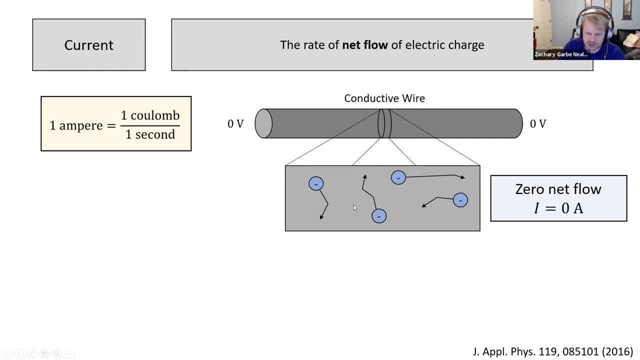 there's zero net flow in of charge in the material. however, it's still important to to realize that the electrons themselves are still moving. the free electrons, that is, the conductive electrons, are still moving fairly rapidly within the material and and with maybe random motion when they collide. 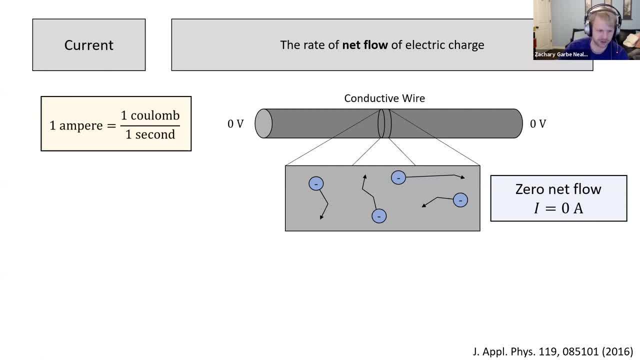 with, you know, other atoms, they will deflect their, their trajectory and that collision, the distance they move until collision, is called the mean free path, or rather the, the average distance these electrons or particles travel before colliding is called the mean free path. and for I found a paper that calculated different elements. 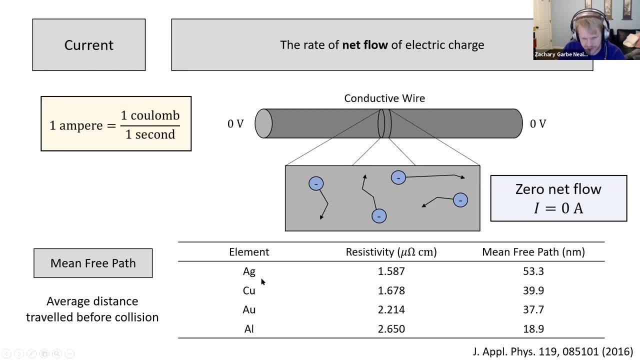 and their mean free paths. and so we, we look at silver, for example. silver has the electrons in silver have a mean free path of 53 nanometers, which is quite large if you think about it, because we, we can make nanoparticles of silver. you know around 10 nanometers and we can make nanoparticles. 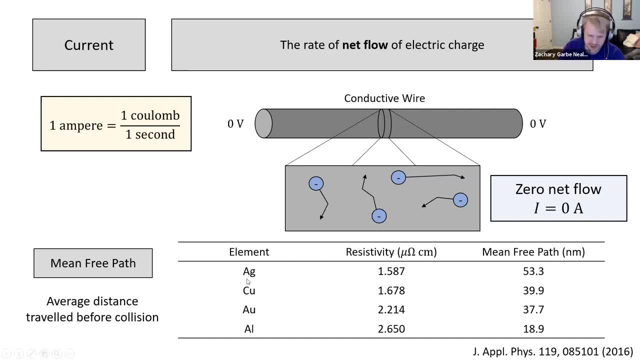 of 50 nanometers very easily, and so it's possible to make particles that have a dimension that's smaller than the mean free path, meaning that the electrons will not bump into any other atom. for 53 nanometers, which I think is is quite large distance, and it kind of gives you an idea of how. 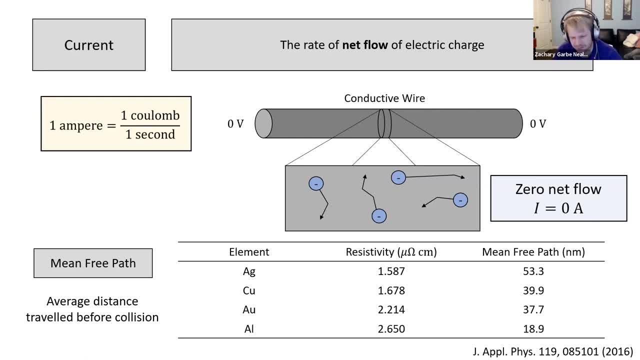 empty atoms really are right. remember a, you know, when we think of a atomic model of metal, we always think of the hard sphere model of metal. and we think of the hard sphere model of metal and we think of the hard sphere model of metal and you know that's, that's a good approximation to think. 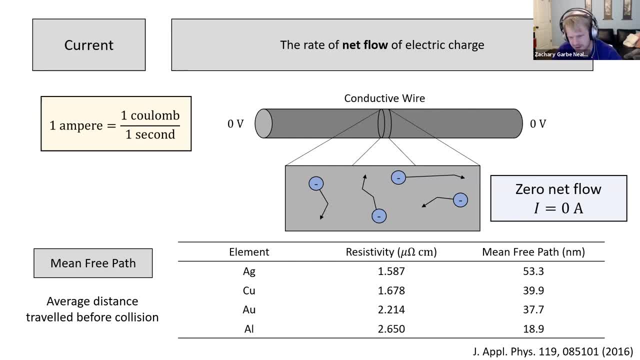 of bonding bond distances between atom centers. but you know, reality, that these electron clouds are mostly empty, and so electrons can zing through without any deflection at all. okay, so let's move on. so let's suppose that instead of zero volts, we we put a potential difference. 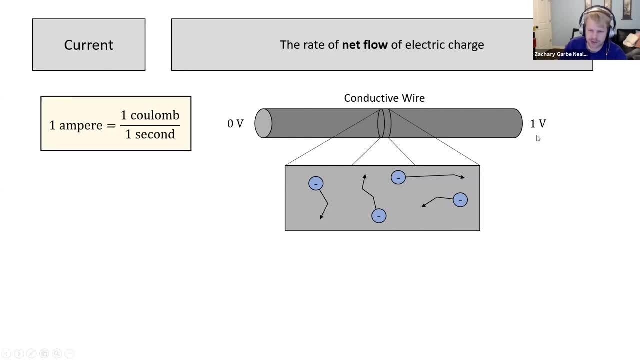 across these, the two ends of this wire, so we have a one volt potential difference, for example. then what is? you know? what would we expect to happen? and what would happen is that we would have a net flow of electrons. in this case, this is a positive potential and, by convention, 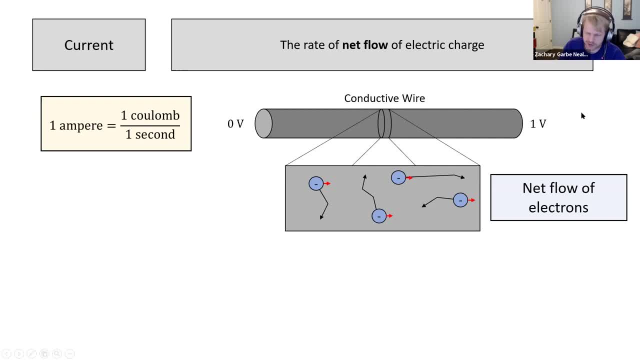 current flows from positive to negative potential, and I mean by convention. by definition, current is the movement of positive charge, but you know, realistically we think of the movement of electrons which are negative charge. so we're going to have a net flow of electrons and we're going to have a 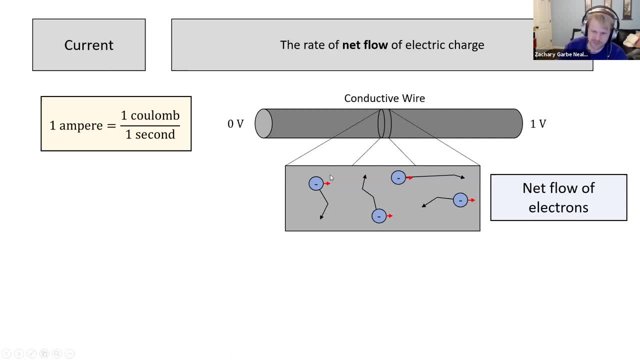 so the electrons will flow in the opposite direction of current. so that's why they're flowing to this higher potential, which is a lower potential for the electrons, but higher potential for protons or positive charge. okay, so one one question I have for you guys is: how fast? 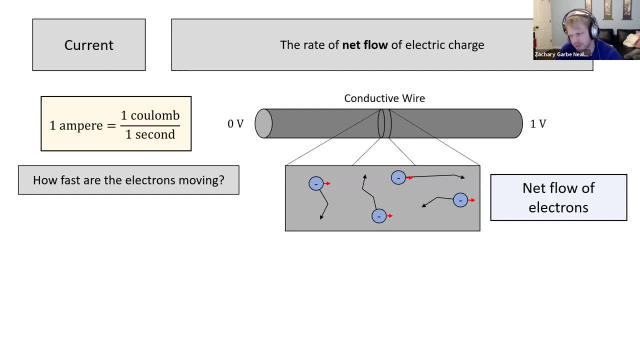 do you think these electrons are moving all right? so you say speed of sound in the object? um, hey, that that's a pretty good guess. um, however, I would say no, not quite. the speed of sound does relate to- uh, I'd say, mechanical motion. I think it's more. 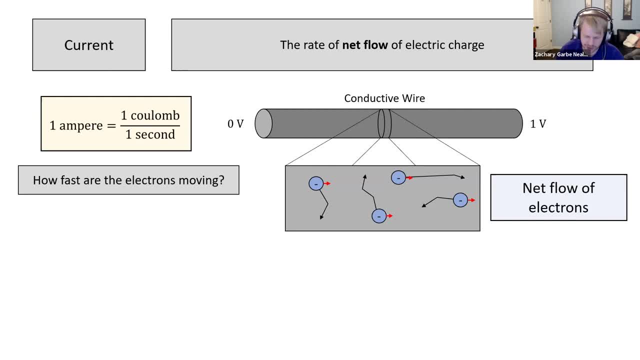 related to the mechanics, right, like if you, if you bump the material, the material can only uh be mechanically, um you know, sensitive as fast as the speed of sound, right, so that has to do with the bonding of vibration. you could say, yeah, so that uh a good, good guess, but not quite so. it's a bit of a trick question. 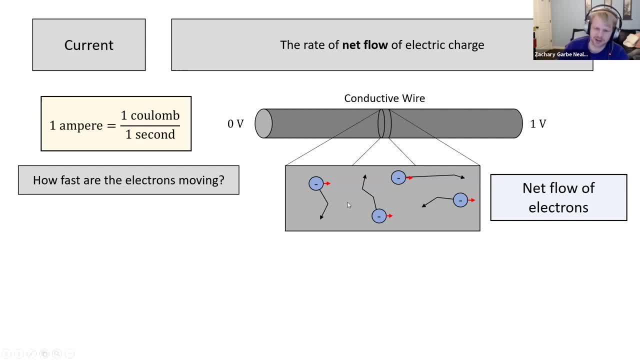 kind of, because you could think of this in two ways. one is, like I said, these electrons are moving in random directions all the time at very high speeds, and that speed is about a third of the speed of light, so around a hundred thousand meters per second, so very fairly quickly. however, uh, if we 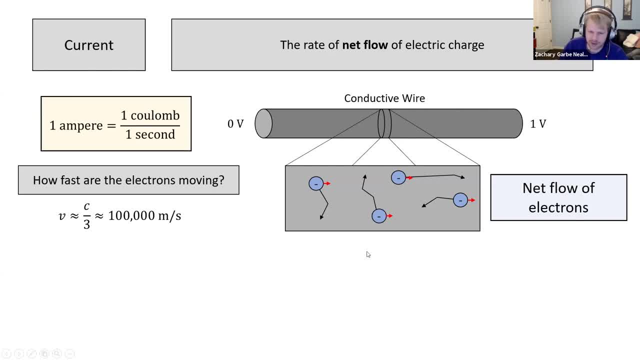 want to specify how fast is the, the net flow of electrons, you know, towards to this positive potential? uh, that's a bit, a bit slower. um, so if we were to draw an imaginary line here, uh, imaginary cross section in this wire, the question is: you know what's the net flow, the speed of the net flow? 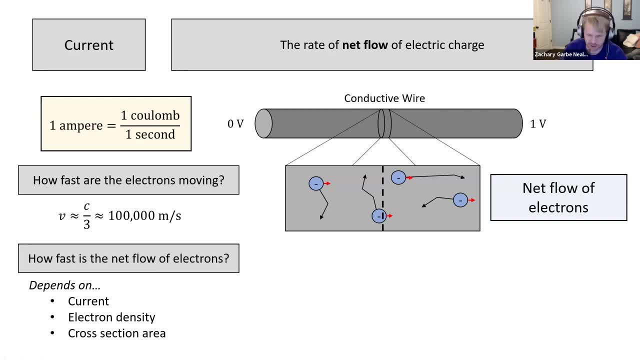 of electrons. you know it depends on several things, such as you know, of course, the current, because that that is the net flow of electrons, um electron density of the material, so how many electrons per volume inside the material, that's a material property- and then the cross-sectional area that 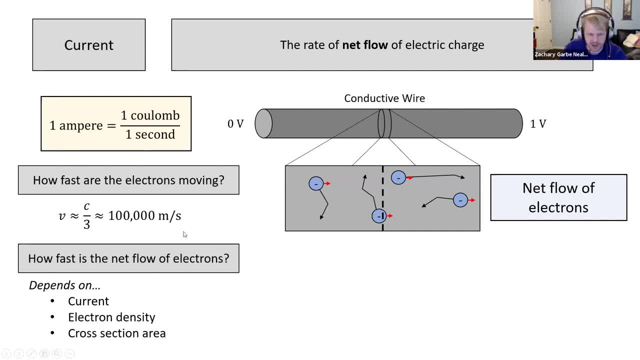 we're looking at. so my current is coulombs per second, but I guess my question is: you know how can we turn this into centimeters per second? okay, uh, so if we let's assume some things, let's assume that the current in this wire is one amp or one coulomb of charge per second flowing through this. 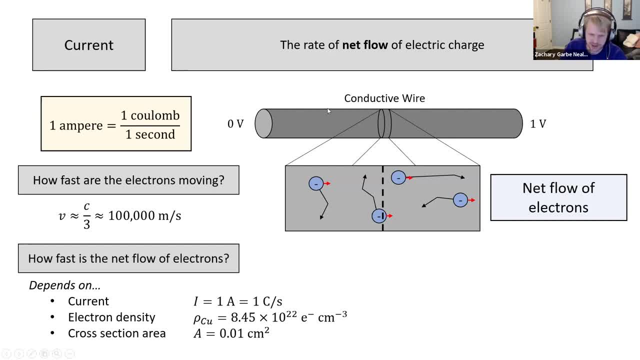 this cross section, the dense, the electron density- and let's say this is a copper wire of copper- is 8.45 times 10 to the 22 electrons per cubic- excuse me, centimeter, and the cross-sectional area is about 0.01 centimeters squared, that's. 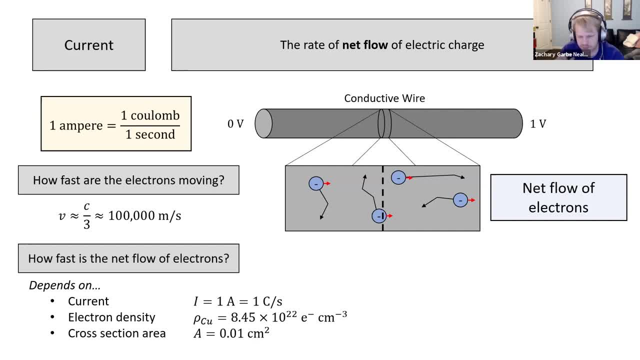 about. uh, that's a little bit bigger than a wire with one millimeter diameter. um, so we can. we can solve this to turn, you know, current, from coulombs in the sec per second into centimeters per second, um, using- and I always forget this and I asked the the morning, class this as: 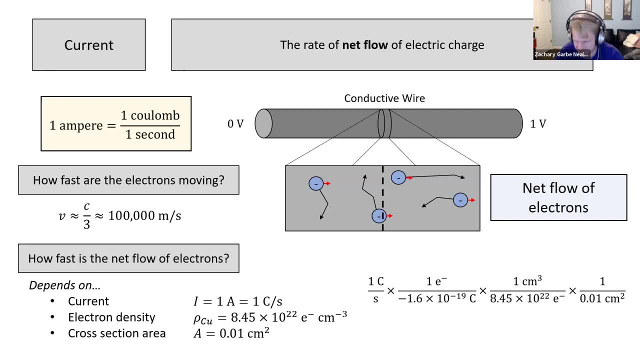 well, what is it called? uh, different. I always want to say differential analysis, but that's not right. what is this called a dimensional analysis? dimensional analysis, right? so we just we plot them in and we, we take off the the units until we get into centimeters per second. so we start with one amp coulombs per second there. 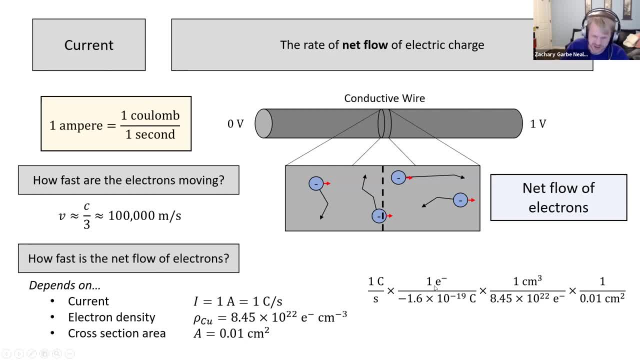 is a conversion here that hasn't been mentioned, but it was mentioned on the last slide. one electron has a elementary charge of a negative one point of 1.6 times 10 to the negative 19 coulomb, and that's a negative one point of 1.6 times 10 to the negative 19 coulomb, and that's a. 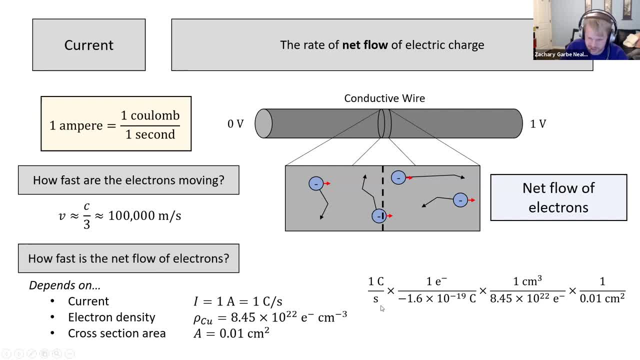 그래서 next we want to try to Roz Coulomb. so the ratio of lambs to electrons per second M's all right. so now we get rid of cool homes. we have electrons per second. now, passing, passing through this point, times the electron, inverse of electron. 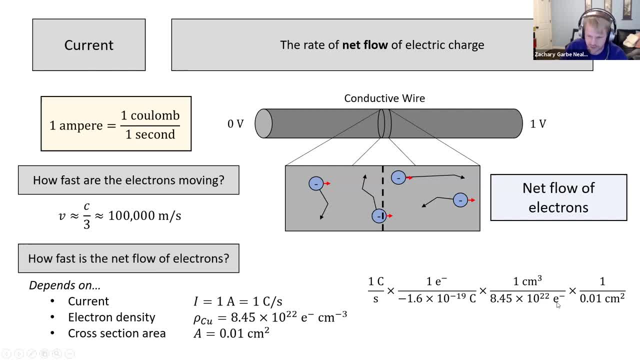 density. so now we got centimeters cubed per second and then divided by the cross-sectional areas that turns into centimeters per second. and so weekend for you times the electron inverse of the electron density. so now we got calculation. you end up with what's called the drift velocity of the net. 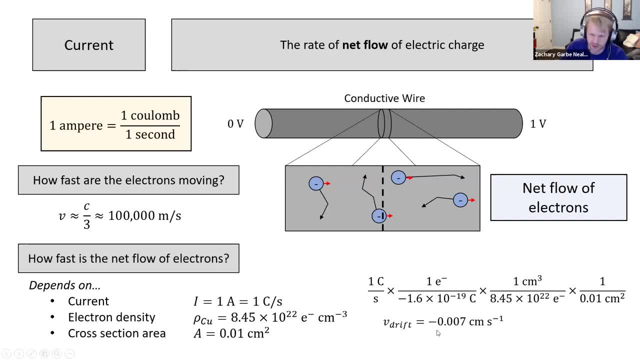 stolen deductions. that иде thatems. so much by this. yeah, light electron values of the net electron flow. and this comes out to be negative model. zero point zero, zero, seven centimeters per second. so that turns out to be objective vector velocity of the net electron flow to get to that upper index. Razorkar delloyer. 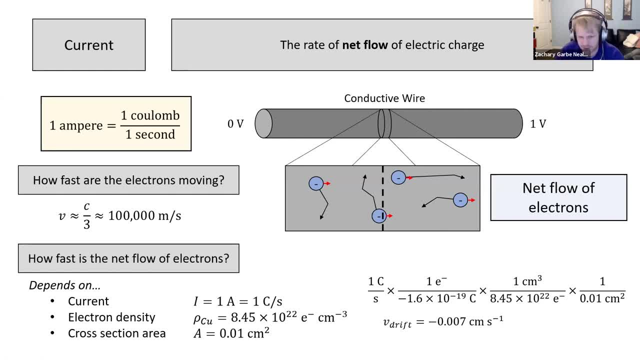 run appears is being same as without coverage. is being shown, Bayer, any relation to this if there's a constant Le international second? so so in reality, the net flow of electrons in a wire of this size and this material for one amp, which is a quite a bit of current, is very slow, very 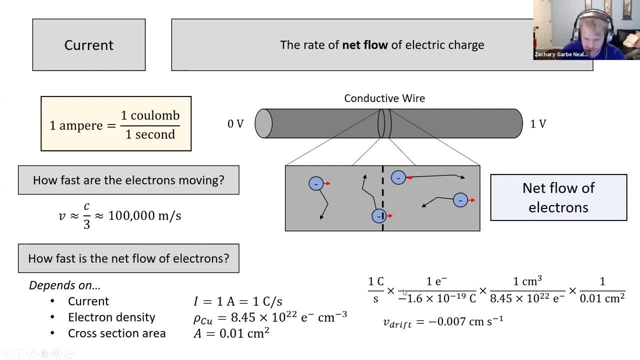 slow, especially relative to the actual electron speed. the reason why this is negative again is just by convention, these electrons flow in the opposite direction of the current- right current would be right to left, but in this case electron flow is to higher positive potential. okay, does that make sense? oh, 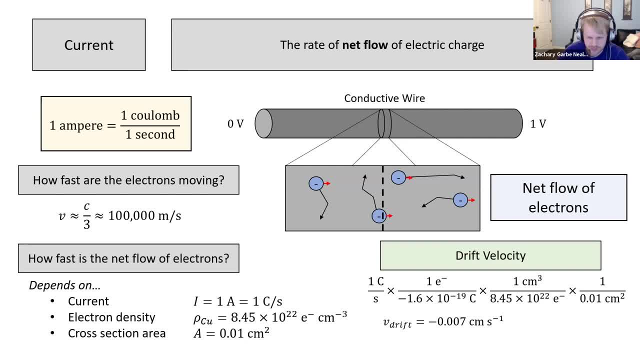 so still on this slide. so yeah, it's called drift velocity. the drift velocity is related to the, the charge mobility. the mobility of the electrical current is tied to the charge. its kind of like the big 자� to the electron mobility or, in p-type materials, might be the whole mobility, and so I'm sure you've 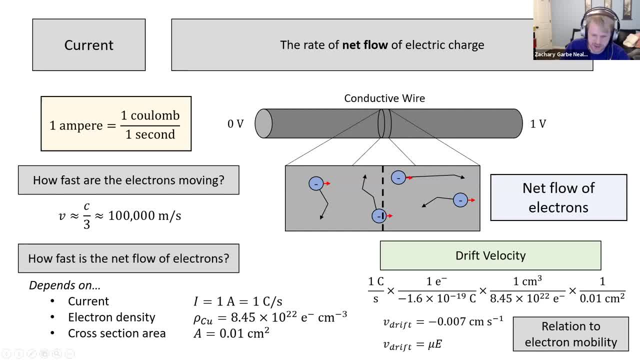 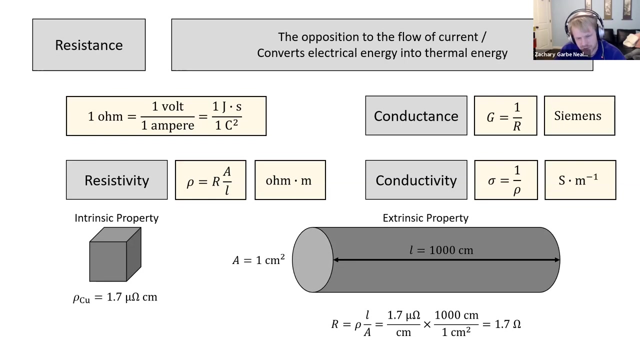 talked about this in your last quarters- class electronic properties. the mobility is a material property. so here drift velocity of these electrons equivalent to the electron mobility times the electric field. electric field is just the voltage divided by the distance that it's across. okay, okay. so let's look at resistance. resistance is the opposition to electron flow or current. 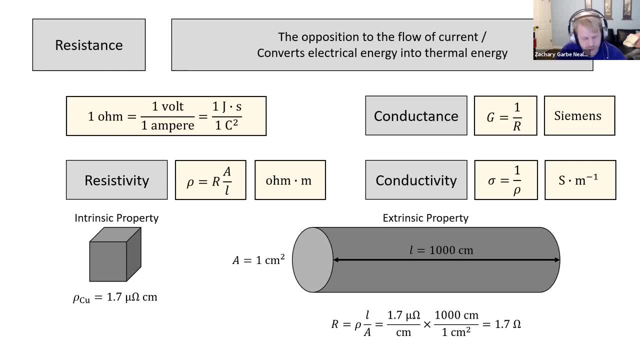 and also another way of looking at resistance. it converts electrical energy into thermal energy. all right, and I think you, you guys, did that in the your autumn quarter. you were looking at the power drawn from a light bulb. I guess you weren't really looking, but you calculated resistance and you could. you. 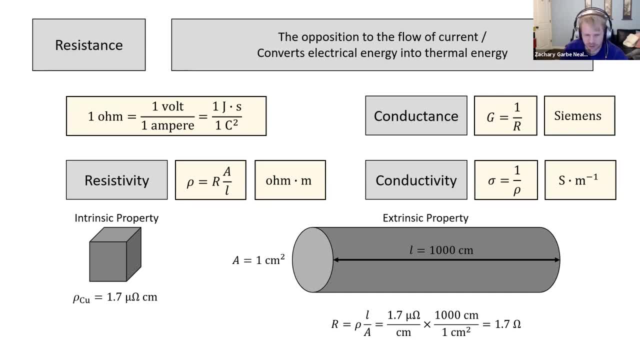 know power of the light bulb, or rather energy or watts joules per second is power is how much energy is being converted into thermal energy which also, from a consequence of that, gives off light. for a, for an incandescent light bulb. so resistance has a unit of ohms which is equivalent to, just by ohms laws, one volt per. 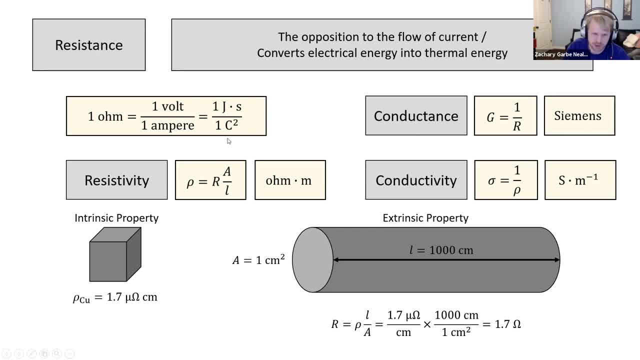 ampere, but it also has equivalent units of joules seconds per coulomb squared, because a volt is a joule per coulomb, an ampere is a coulomb per second. the inverse of resistance is conductance with, with a simple g, so just the inverse, the reciprocal of resistance, and it has units of siemens. 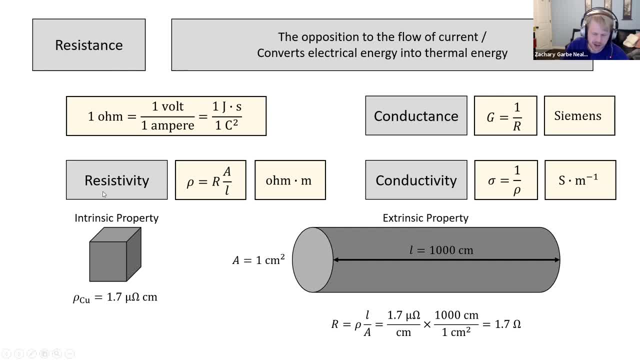 resistivity is a material property where resistance is not. resistance depends on the dimension of the material. resistivity is independent of the dimension or volume of the material. resistivity is rho, which is a bit confusing because in the last slide I used rho as electron density. but now 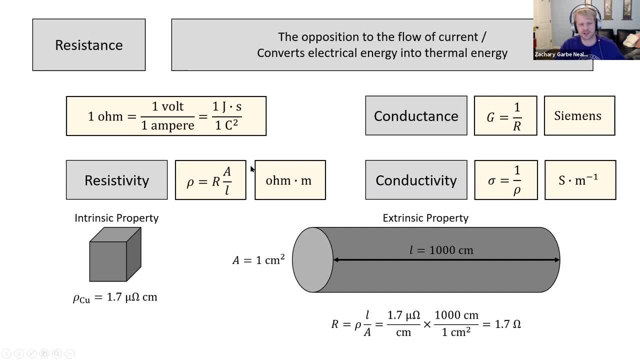 I'm using it, as resistivity is equal to the resistance times, the area of your object divided by the length of the object, and so it has units, ohm meters it's. it's important to take a note that these are kind of weird units. you know you're not going to be able to do that if you don't have. 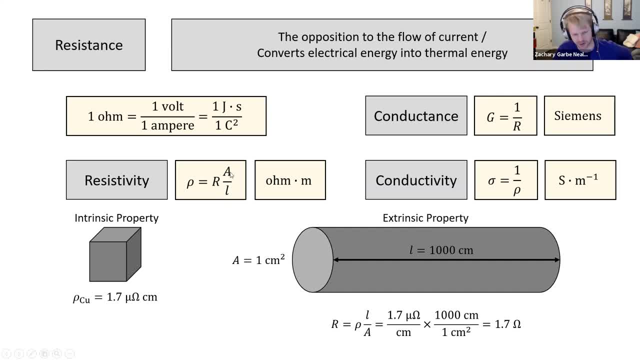 it has meters here, and that's because you're multiplying by area and dividing by length, so resistivity is an intrinsic property. all right, and resistance is an extrinsic property. so in this example I have a a wire of a length uh 10 meters. cross-sectional area is one centimeter squared, so 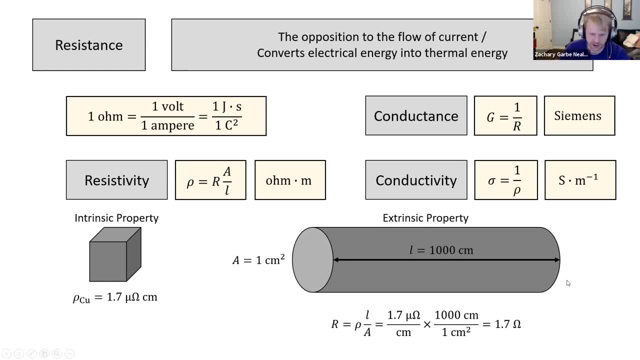 kind of a pretty, pretty big wire and uh. so if you wanted to calculate the resistance of that wire- and let's suppose it's copper, which has a resistivity of 1.7 micro ohms per, not per 1.7 micro ohm centimeters- then you can calculate the resistance of that. 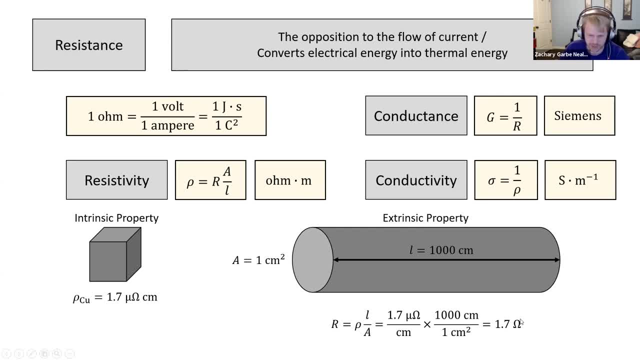 length of wire and so that comes out to 1.7 ohms using that equation. all right, so uh pretty, that's pretty low resistance, especially for such a long, a long wire. and you know that's why we use power. the power of the wire is so important because it's a very long wire and it's a very long wire. 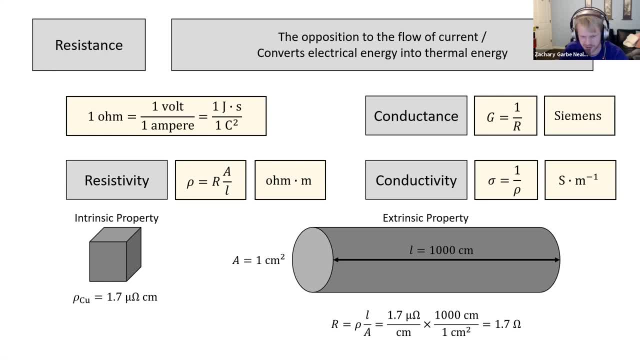 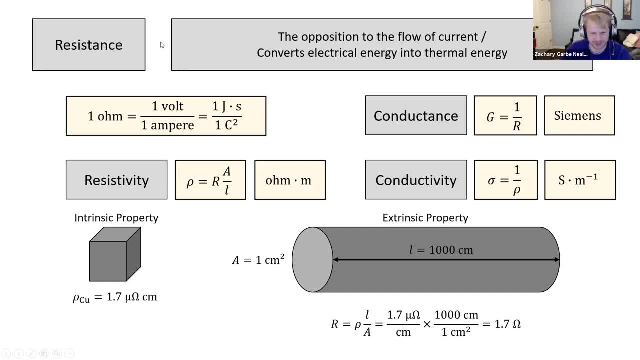 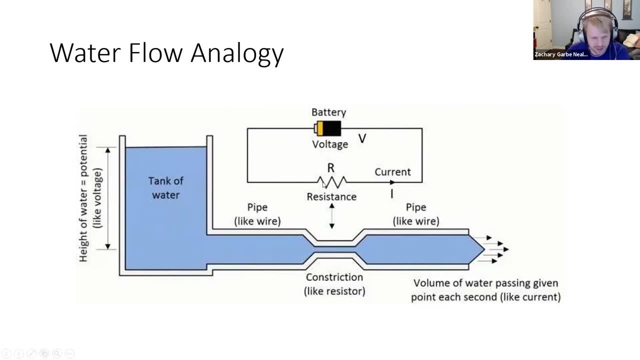 would be a superconductor that doesn't have any resistance, but that's a bit pricey, okay, okay, so back to the water analogy. um, so here we have an entire circuit, the battery, a resistor, the current through the circuit, and so, again, like i said, the, the voltage across the battery, is analogous to the height of the water. 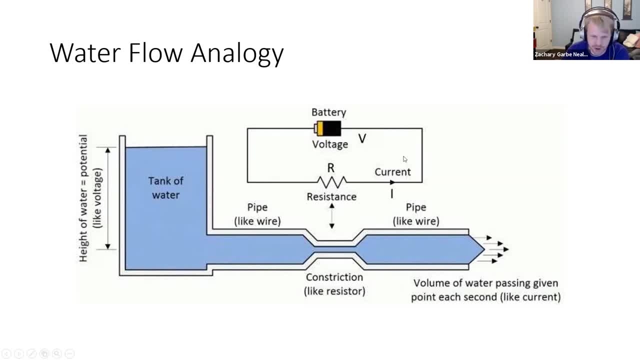 that has potential energy to flow. the current in the circuit is analogous to the flow of volume, so not not the speed of water, because, uh, the the current through the system, the current through the circuit needs to be the same. the current through the circuit needs to be the same. the current through the. 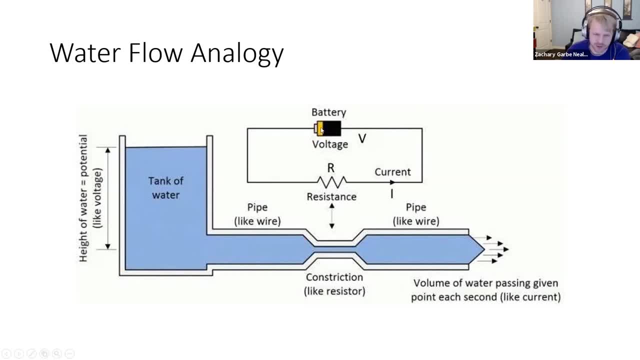 through the entire circuit. you know, whatever the number of charges per second out of the battery needs to be equal to the number of charges per second into the battery, even through the resistor. the current needs to be the same. So it's the same in this analogy, the flow of volume of water. 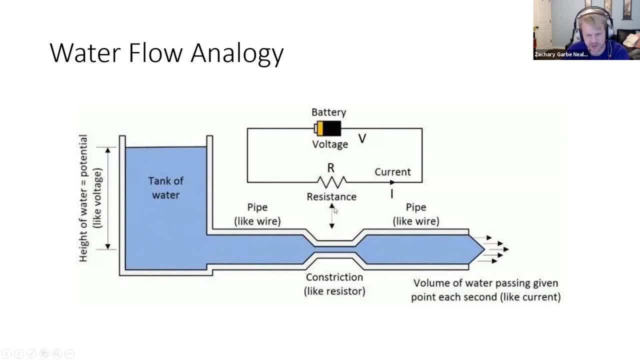 passing through this constriction, which acts like the resistor, needs to be the same. So that means that the speed of flow, the velocity of water in this constriction, must be faster in order to make the same amount of flow. So flow of water is like the current. this constriction is like 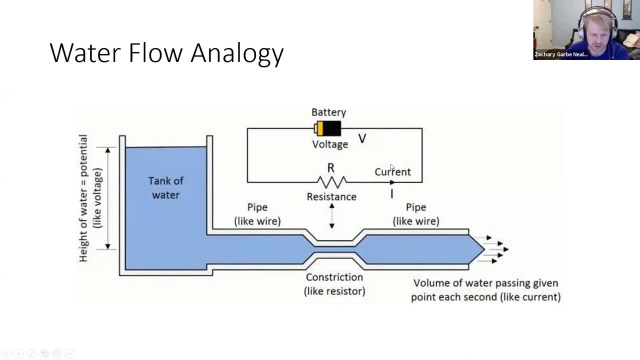 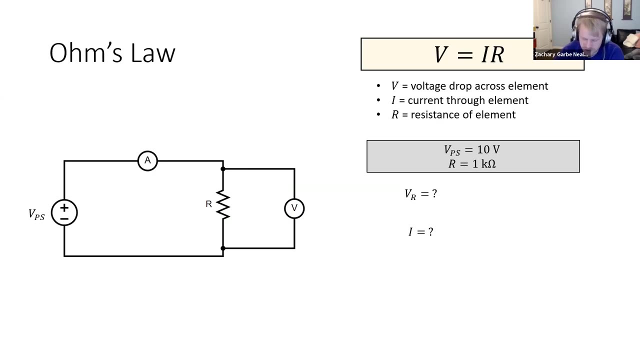 resistance, the height of the potential energy is like the voltage, And if we were to have a battery, it could be like a pump that pumps the water back to the top. So these three things are related by Ohm's law, Which is: voltage equals the current times, the resistance, And so here's an example of how you 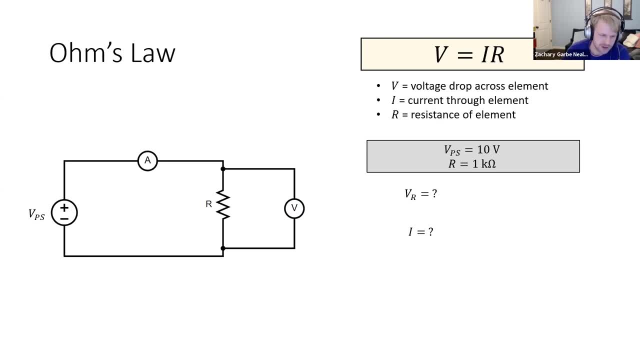 could use Ohm's law to calculate current in a circuit. So here's a simple circuit. we have a constant voltage power supply, For example, maybe like a battery, although batteries are not necessarily constant voltage, because the voltage depends on the current and most of it doesn't. 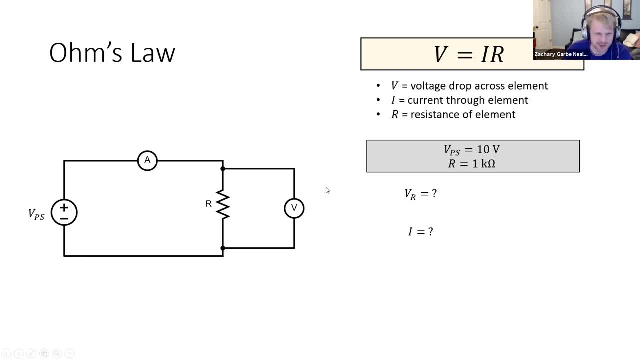 matter If the constant voltage power supply, we'll say it's at 10 volts. Here we have an ammeter to measure the current, We have a resistor in series with the circuit And, like I said, the voltmeter is in parallel to whatever element you 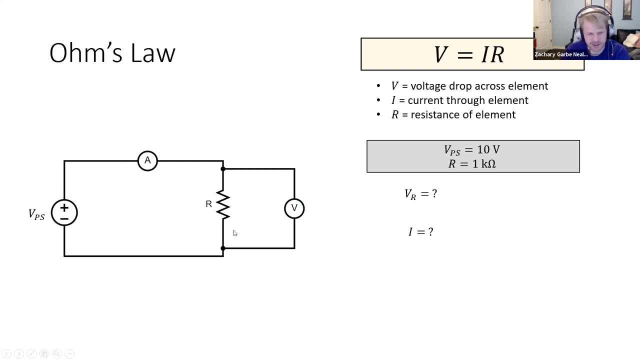 want to measure. Now, one assumption we have to make in these simple circuits is that the resistance of the wire is negligible, And we'll just say zero for now. that the resistance in the wire is negligible. The only resistance we care about is the resistance of the resistor which is put at one. 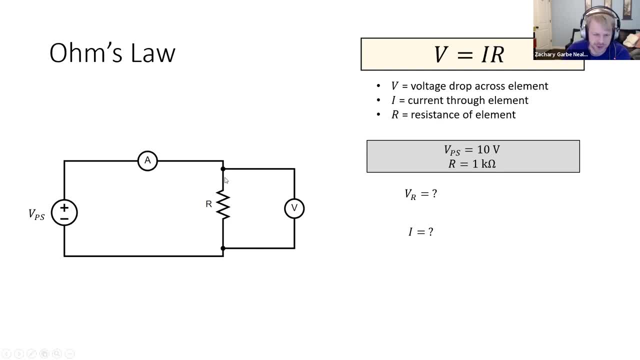 kilo ohms. So if we were to measure the voltage across this resistor, what would that voltage measure? What would this voltmeter measure? So that's a question for you guys, And this one's kinda easy to think about. what would that voltage? 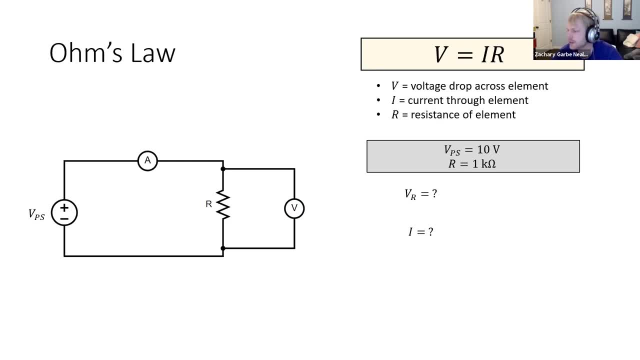 be. yeah, Aaron says 10 volts and that's correct. so because this is the only element in this circuit and you know, if you look at this, we have a probe of the voltage above the resistor and a probe below it. this would be exactly the same if we 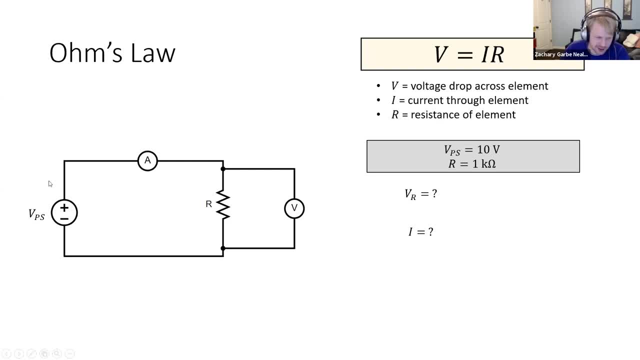 took this probe and put it over here and measure the voltage across the voltage source. it's the same thing as what we're doing right now, so we're just measuring the voltage of the voltage source- source basically. so the voltage drop, the voltage drop across the resistor, is equal to the voltage provided by the 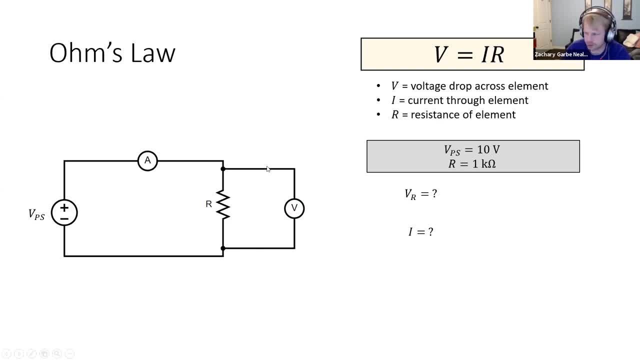 power supply, which would be 10 volts. so if that voltage is 10, then we can calculate the current using Ohm's law, and it's a bit simple so I'll just do it for you guys. so using Ohm's law we say the current across the resistor is equal. 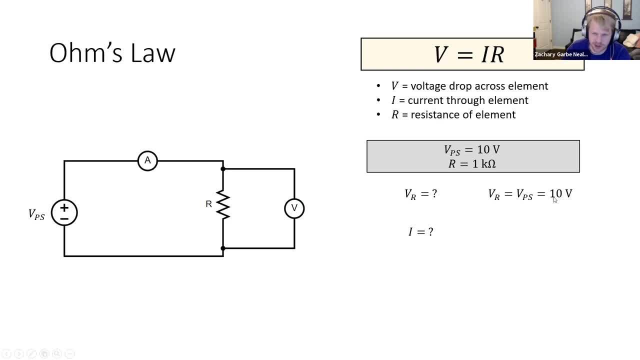 to the voltage of the voltage source and the voltage drop across the resistor is equal to the voltage drop across the resistor, which is 10 volts, divided by the resistance of the resistor, which is 1 kilo ohm, so 1000 ohms, so 10, divided by. 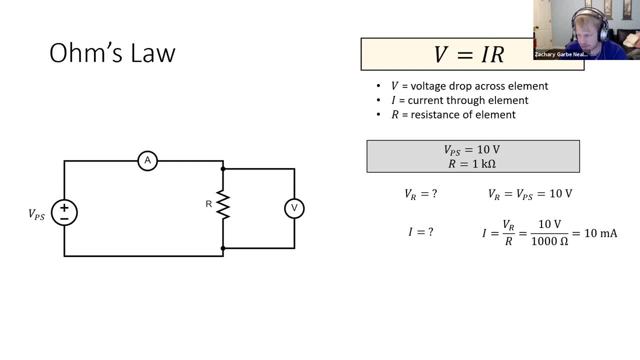 1000, that's 10 milliamps. so that's the amount of current that goes to the resistor. and remember, like I said, the current that comes out of the power supply must be equal to the current that goes into the power supply. you can't. 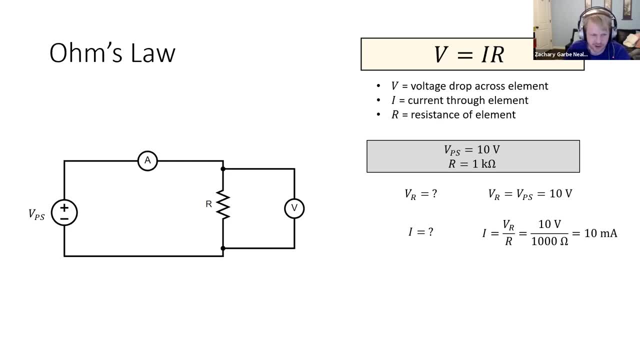 have an accumulation of charge anywhere in the circuit, you have to have equivalent or you have to have charge balance. that is so the number of coulombs per second out is equal to the number of coulombs per second in. so that must mean the current through the resistor is all and all the wires are all the same. so 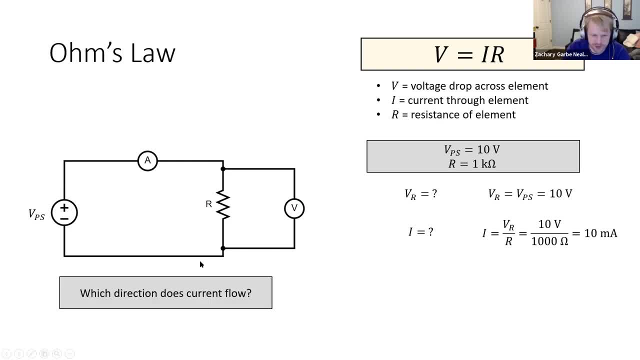 here's another question. I have a couple more questions for you guys. first one is: which direction does the current flow in this circuit? all right, we have. we have two options. it can flow in the clockwise direction or the counterclockwise direction. so if you're using a resistor, and you're using a resistor and you're 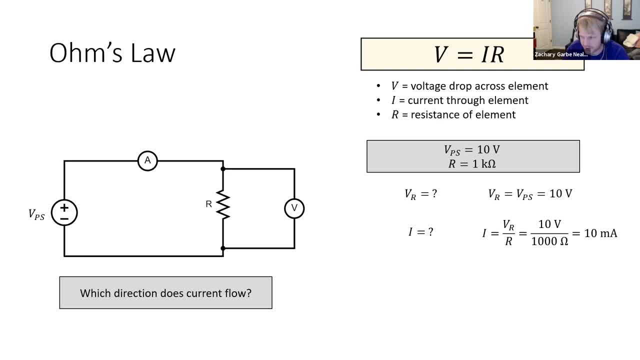 using a resistor for a single circuit. they have both counterclockwise and counterclockwise. now I'm using a resistor if you're running across this circuit- and you're just running through this circuit- I don't want you to be hot Opening. Tor Sü müs. 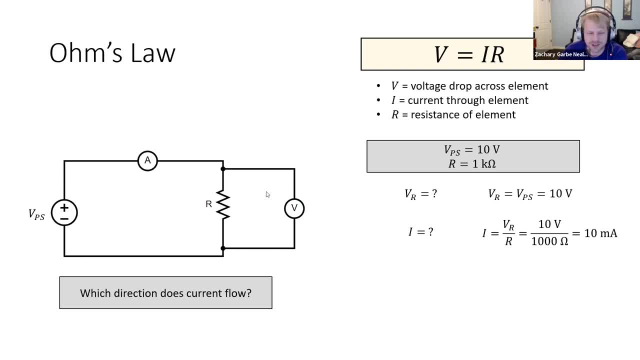 hey, into this next one. we have this. it's a book of wonderful knowledge, interesting. i'm gonna look counterclockwise. So, no, the answer is yes, It goes clockwise, right, Yeah, clockwise. So remember the current by definition, or I guess by yeah, the convention or definition is: 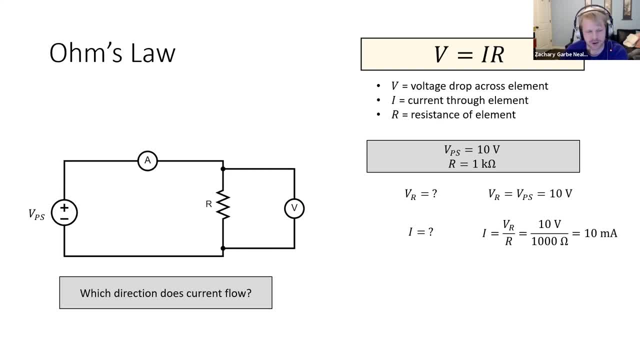 the flow of positive charge. So positive charge flows from the positive terminal of the power supply to the negative terminal of the power supply. So positive charge is flowing. oh, I have a picture. I think, Let me. the current is flowing in the clockwise direction, okay, Which means that. 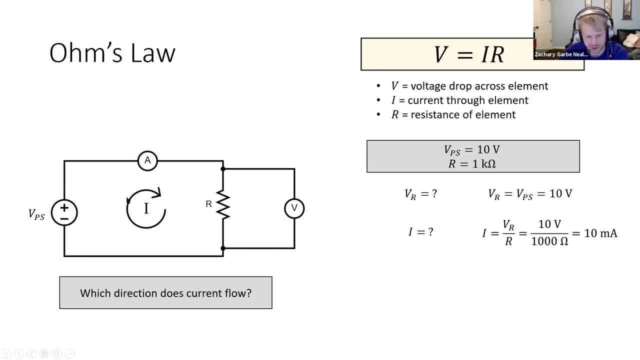 the electrons are flowing in the opposite direction, counterclockwise. So electrons come out of the negative terminal and they flow into the positive terminal. all right, How about? how about this? this little circuit right here? We have another loop here. The voltage is also connected there. Is there any current that goes through this voltmeter? 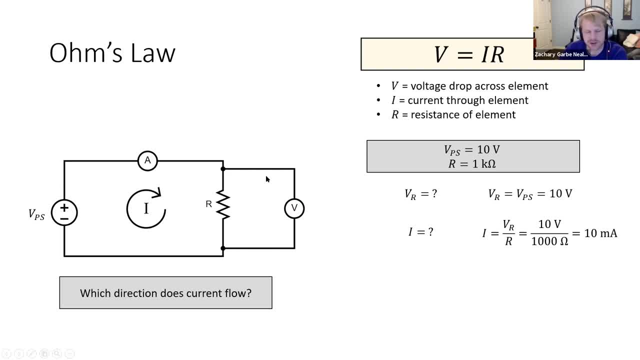 So there there, ideally, ideally, there's no current that flows to the voltmeter. Now, in reality, yeah there, there has to be a little bit of current in order for the voltmeter to measure. There has to be a little bit of current, And voltmeters are typically what. 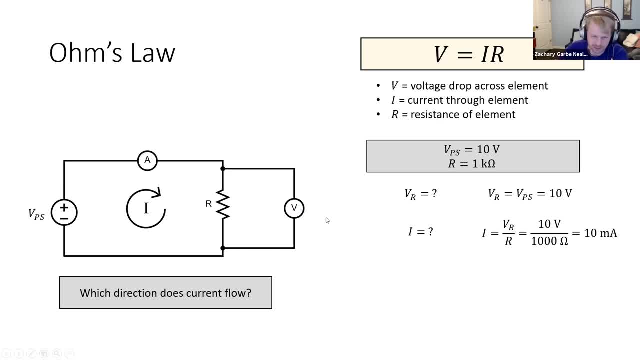 we call high impedance devices. So impedance related to resistance, it means that the resistance across the voltmeter is very high. It's like I think that for very cheap multimeters it's like 10 mega, milli-ohms, mega-ohms, 10 mega-ohms and then higher end, more accurate, precise. 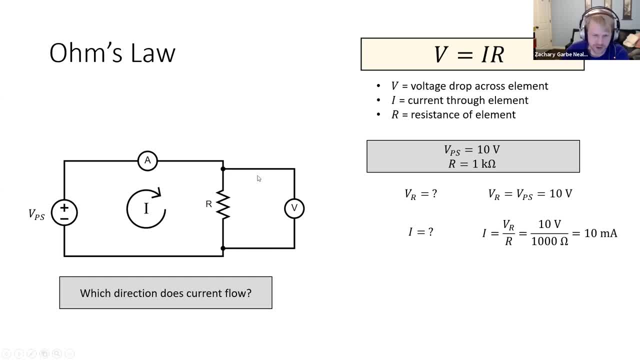 multimeters is like giga-ohms, So very, because the resistance is so high. it's like oh high in the voltmeter. very little current will go through this loop here, which will allow you to accurately measure the voltage across the resistor. Okay, Okay, One more question before. 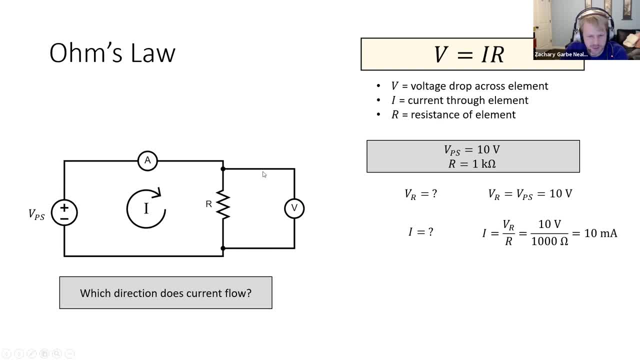 we move on, You know. let's say, instead of measuring the voltage across the resistor, let's say we measure the voltage across the ammeter. So we take these, these voltage points, these probes, and put it one before and one after the ammeter. or or to make it even, 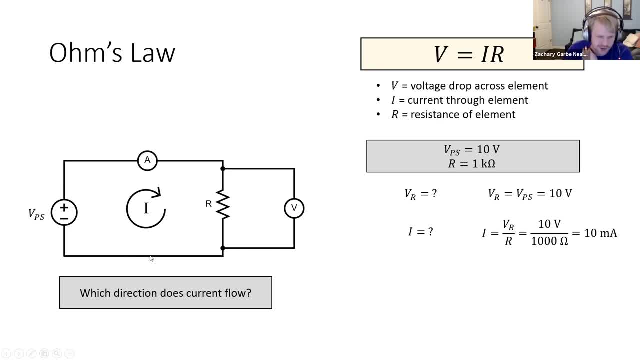 more simple. just say we measure it across two points of the wire down here. There's nothing between it, just one point there and one point there. Question is: what would we measure? What would the voltage measure if we just measured two points on this wire, Or or across the ammeter? 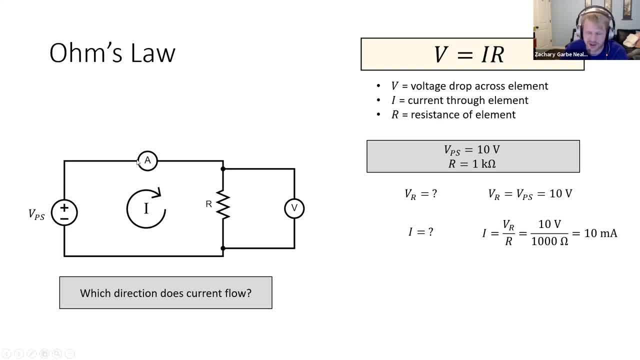 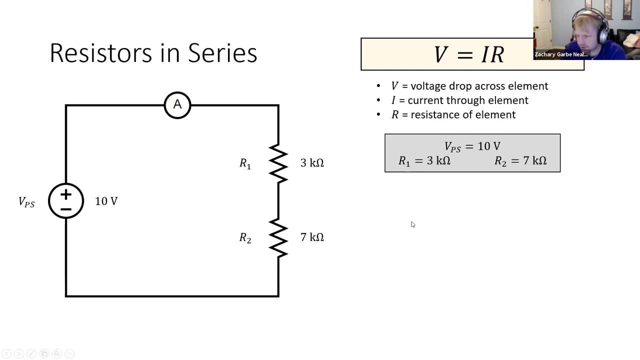 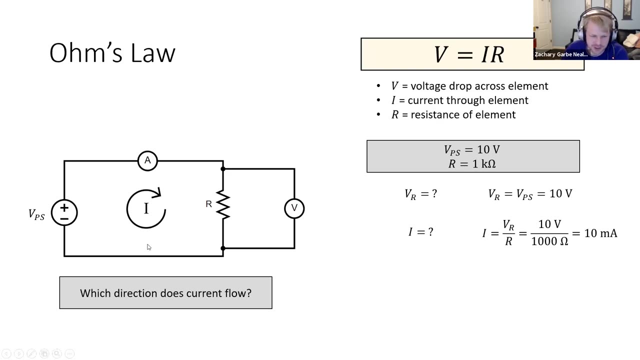 in an ideal situation, there's probably going to be some resistance to ammeter, but theoretically- Oh sorry, Yeah, So I see zero volts. That's right, So yeah, so there'd be zero volts in a theoretical situation. Like I said, we're assuming there's no resistance in these wires. 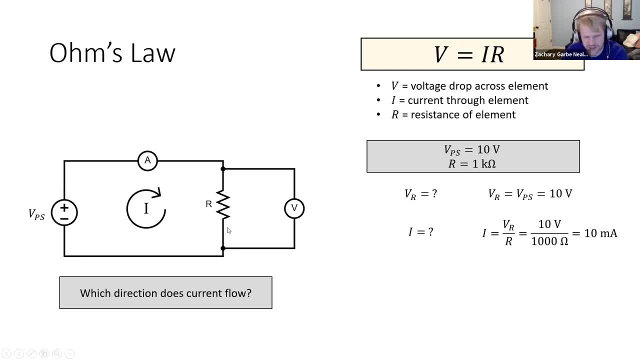 only in the resistor. Now I in reality there there is a little bit of resistance in the wires, And so if we were to measure two points between wires that have a certain amount of resistance, we would. and the current, we know the current. 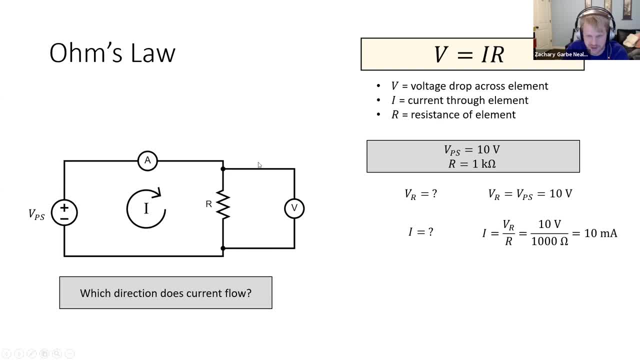 the current has to be the same. The current has to be 10 milliamps through the entire system. So then you could. you would expect a little bit of voltage, But, like I said, because resistance is so small and we're assuming it's zero, it should be zero volts. Okay, Let's move on. 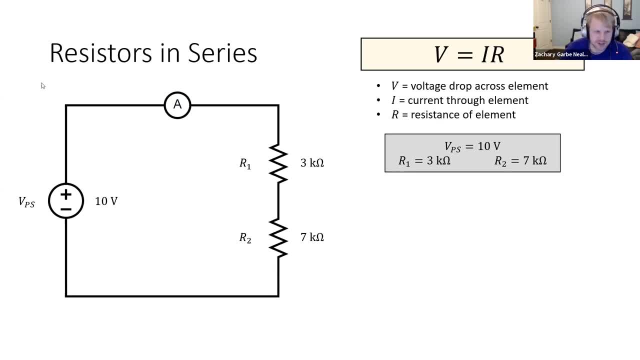 So let's look at two resistors, and these resistors are in series. All right, So they're one after another, they're in the same circuit and they're in the same loop. Okay, We can still use Ohm's law to calculate the current. So let's look at two resistors, and these resistors are in. 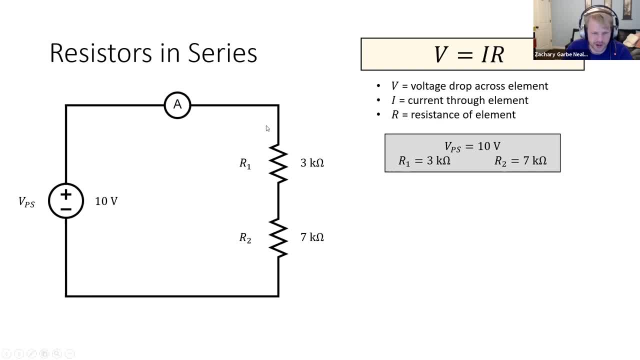 series. Okay. So let's look at two resistors, and these resistors are in series. Okay, We can still use Ohm's law to calculate the current through the system. The question is, what is the voltage drop across each of these resistors? All right, So when you have resistors in series multiple, 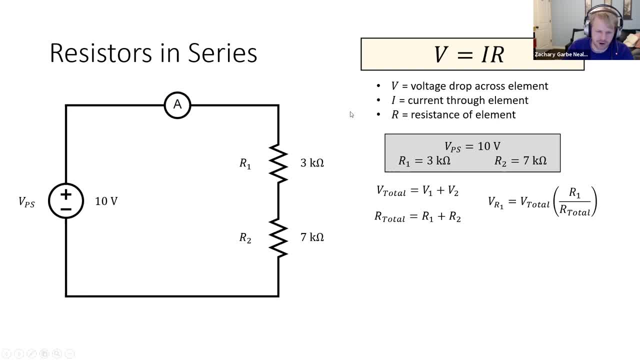 resistors. the voltage drop across all the resistors is, like we said, the same as the power supply. If we were to put the multimeter across both of these, it'd be just like putting the multimeter across the power supply. So there's 10 volts of potential from top to bottom of these. 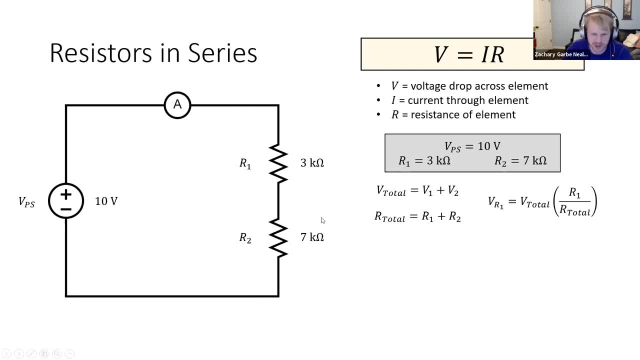 two resistors, And then we have the voltage drop across all the resistors, And then we have the voltage drop across all the resistors, And then we have the voltage drop across all the resistors, And then the total resistance is just the sum of these two resistors. If we were to, we could make a 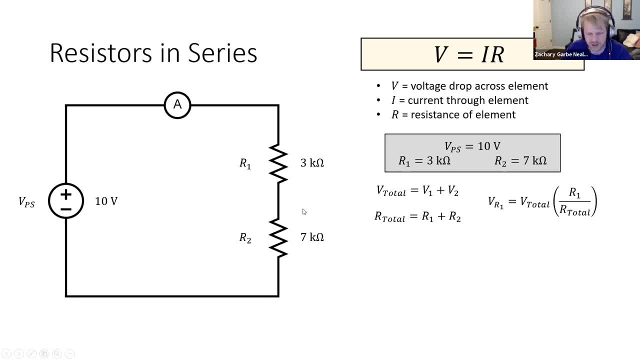 simplification and say these two resistors is equivalent to one 10 kilo ohm resistor. Okay, So if we know the voltage across both the resistors, let's see. And we know, we know the voltage across both resistors and we know the. 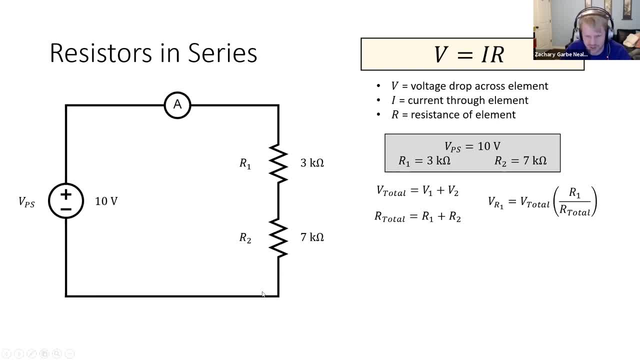 resistance of both resistors, the total resistance, which is 10 kilo ohms. then you can calculate using Ohm's law, the current through the entire system, right? So we have a total of 10 kilo ohms of resistance, a total of 10 volts. 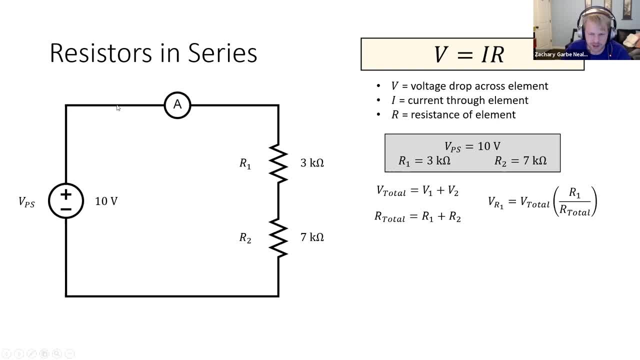 So, the same as before, the current through the system will be 10 milliamps. And now you know the current. the current in R1 is equal to the current in R2, which is the current provided by the voltage power supply. 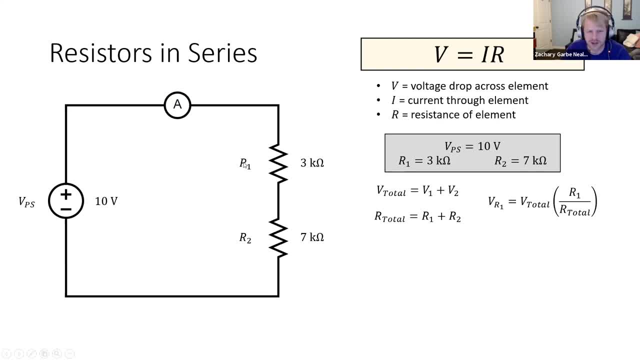 So then you can use Ohm's law again to calculate the voltage drop across each of these resistors, given the resistance, and the current Another. just the equation itself, to make it easy, is that the voltage drop across a single resistor in series is equal to the fraction of its resistance. 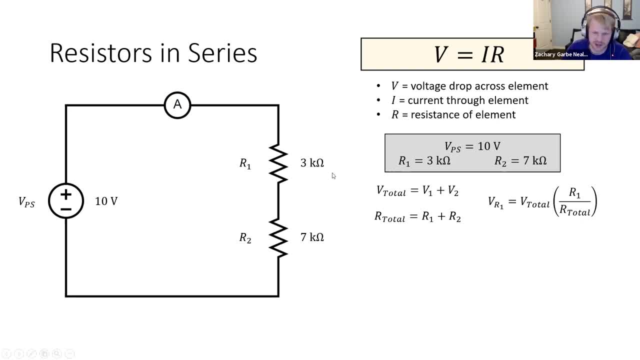 to the total resistance, all right. So in this case for the 3 kilo ohm resistor it'd be 10 volts times 3. dividable, It's 10 by 10, so 30% of 10, basically right. 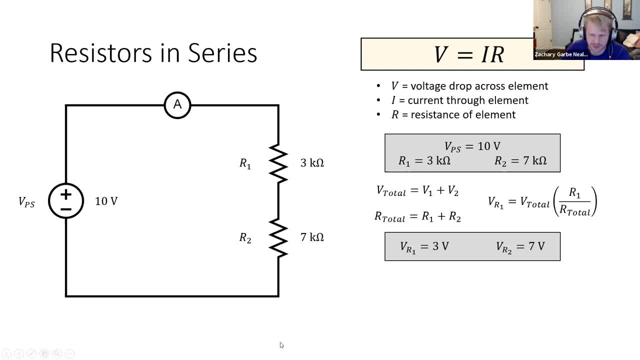 So this has 30% of the voltage drop, This has 70% of the voltage drop. okay, And it doesn't matter if you know R1 is first or R1 is second. okay, It'd still be 3 and 7.. 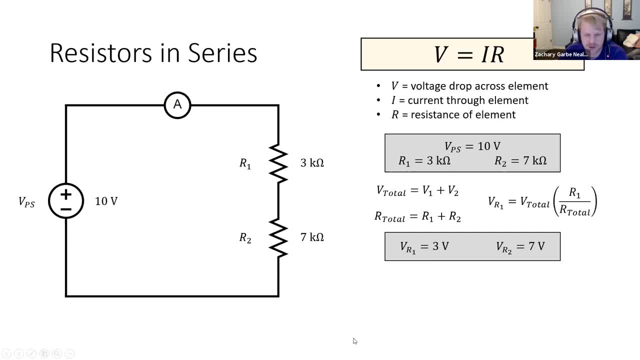 It depends on the ratio of the resistance between the two, or rather the fraction between the two. Okay, Yeah, again the current. you can look at the like I said. you could do it from the total resistance and the total voltage, or you can just. 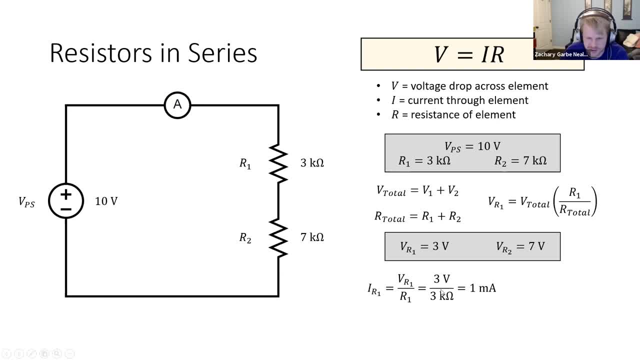 You can just look at the individual resistor and this calculation still works. you know, for 3 volts across 3 kilo ohms and you can use Ohm's law, and that equals 1 milliamp. Oh wait, did I say 1 milliamp? 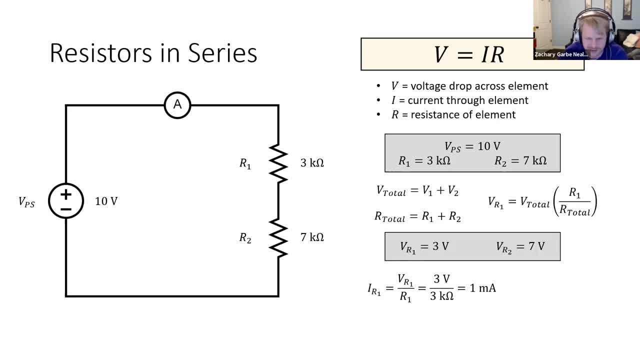 Okay, excuse me, I said 10 milliamps before but it's 1, because I forgot We have 10 kilo ohms. In the previous example it was only 1 kilo ohm. Okay, So basically overall, you need to remember that current, you know. 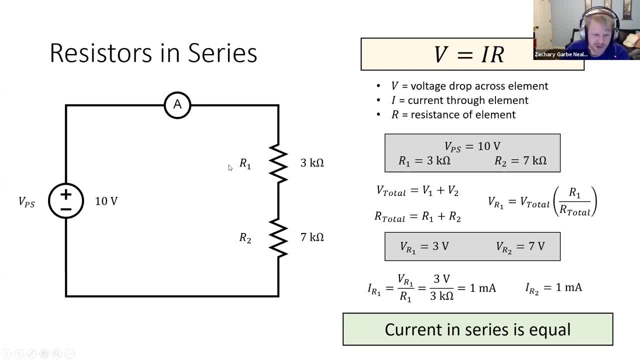 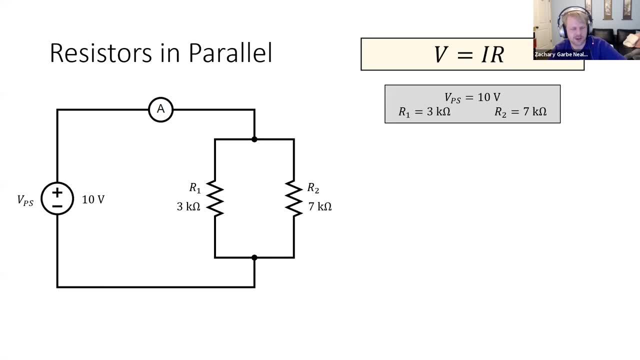 the current is going to be 10 kilo ohms. It's going to be 10 to the power of 1 milliamp. okay, So you need to remember that current through the entire system is equivalent to all elements in series. okay, 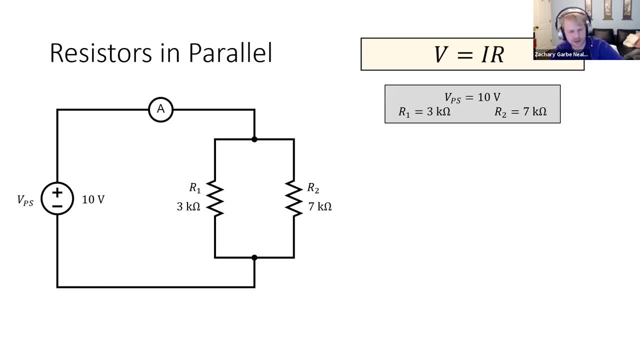 Let's look at another example. This is the last one. is the resistors in parallel? okay, So in this example again, we have a constant voltage supply of 10 volts, but what's different is that now there is a junction where the wire splits. okay, 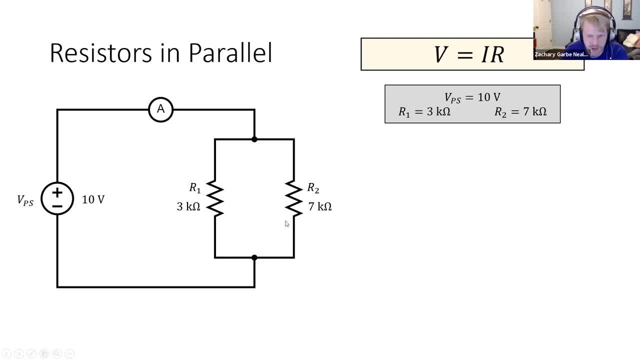 And so we have two resistors in parallel and then the wire splits. The wire has another junction where they combine again okay. And so the question again: what is the voltage across both the resistors and what is the current across both resistors? 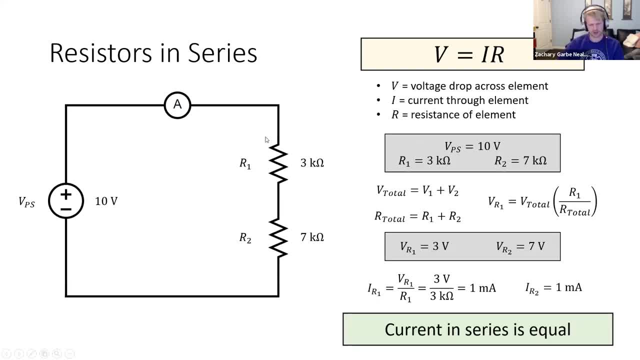 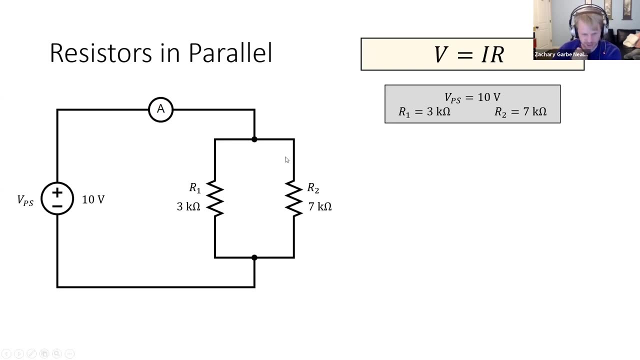 So in the previous case, in series, we said the current in series is equal. right, The current is constant through the entire circuit. but what's different is the voltage? In parallel it's the opposite. The voltage across these two junctions is equal, or in other words, the voltage. 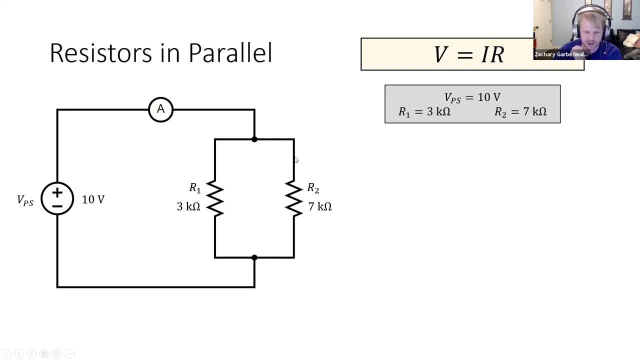 across R1 is equal to the voltage drop across R2, but what is different is the current, And remember I said whatever current goes in in this case, whatever current splits needs to be equal to the current that gets combined at this junction. okay. 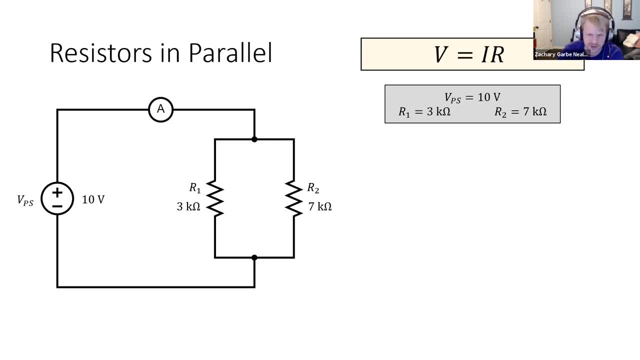 You can't have accumulation or depletion of current anywhere in this circuit. So, like I said, the voltage difference between these two junctions or across each of these resistors is 10 volts, which is given by the power supply. Now we want to calculate the current I1 and I2, through each of these resistors. 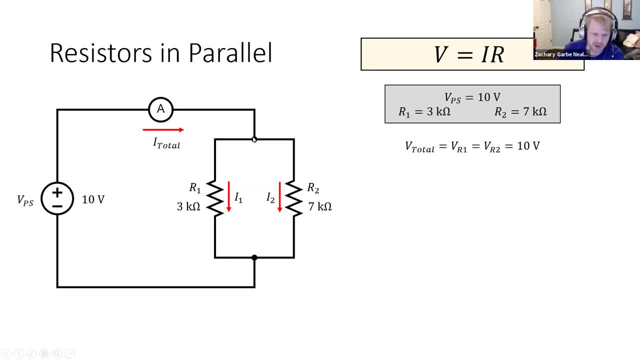 and then also the total current. So remember I said the total current in has to be equal to these two currents. So I total is equal to I1 plus I2.. We know the voltage across each resistor, We know the resistance. We can use Ohm's law to calculate I1 and I2 individually. 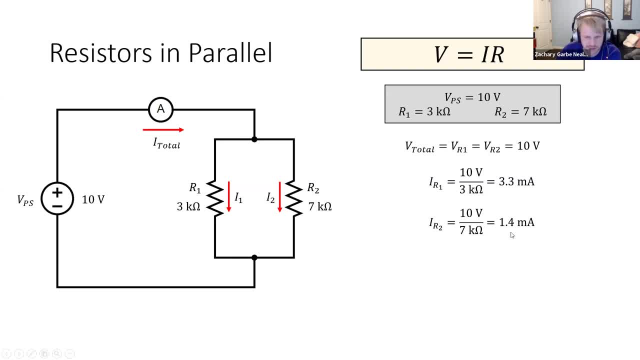 So Ohm's law gives us I1- 3.3.. Okay, So I1, 3.3 milliamps, I2, 1.4 milliamps, and then the total current given by the power supply or supplied by the power supply is the sum of those two currents: 4.7 milliamps. 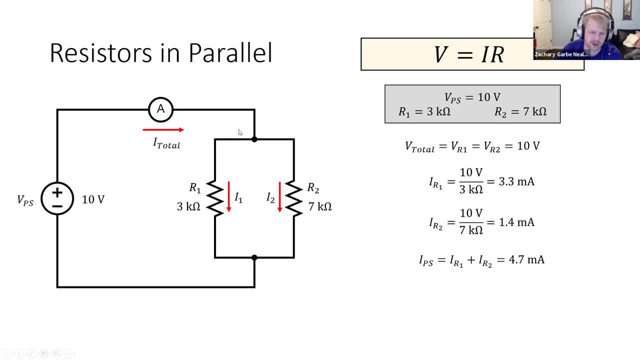 Okay, The other way you could do it. there's an equation to calculate the equivalent resistance. If we were to combine these two and make it a simplification, that total resistance- the reciprocal- is equal to the resistance, The reciprocal sum. 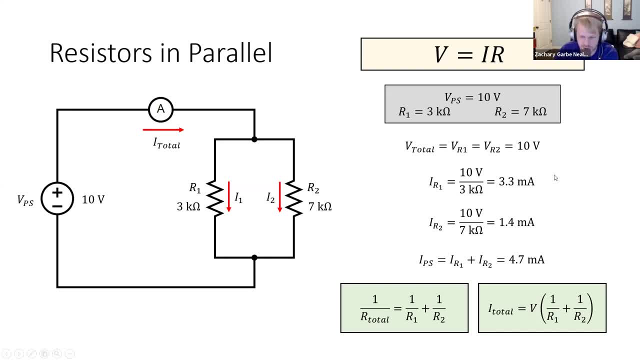 And then the total current. you can plug this into Ohm's law again to get the total current is another way of doing it. Okay, So that was. we were looking at circuits in series, circuits in parallel, to measure current and voltage across resistors using Ohm's law. 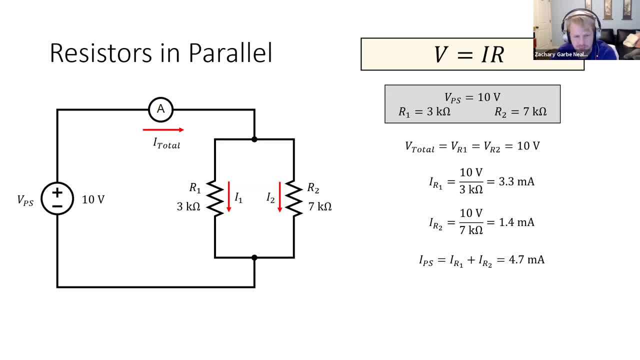 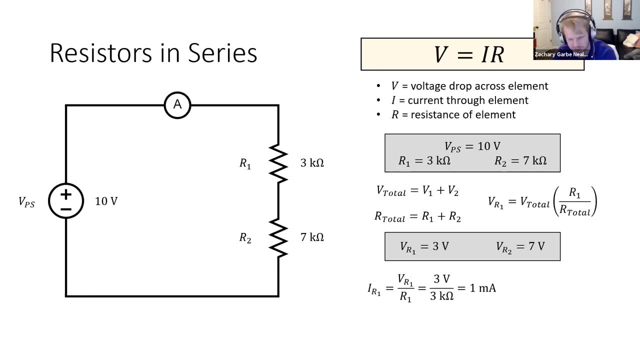 So in lab next week you will need to be able to measure the voltage and current and convert it to current, But it will only be For resistors in series. there won't be any parallel work and it'll be very simple. 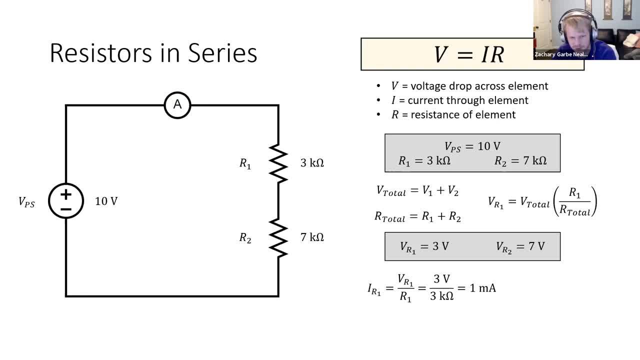 Just like this. you'll have at most two elements. You'll have a resistor and a diode. The experiment will be measuring voltage across a resistor. You'll have to calculate current or something like that. right, So not too complicated at all. 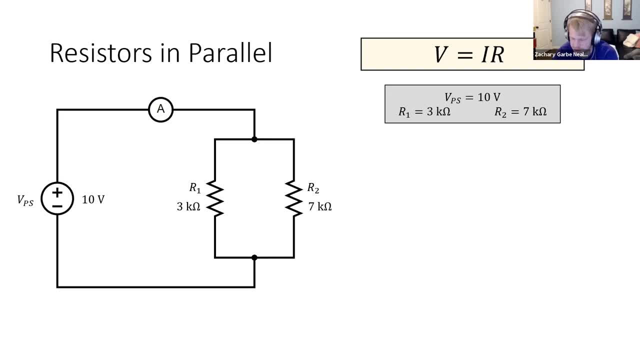 There's a class in electrical engineering. Some of you might have taken it. It's electrical engineering 215.. Okay, Okay, So I believe it's the introduction to electrical engineering. I took it when I was an undergraduate and it was, in my opinion, a difficult class. 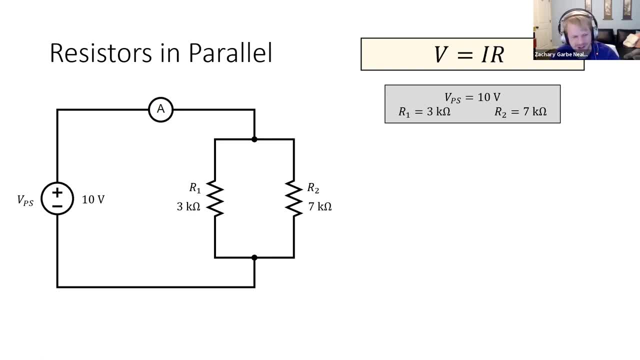 I think it's a weed-out class for electrical engineering students, but I ended up switching to pass-fail because I was afraid I wasn't going to get a good grade. Actually, I did kind of okay, but because I switched to pass-fail, it meant I had to take 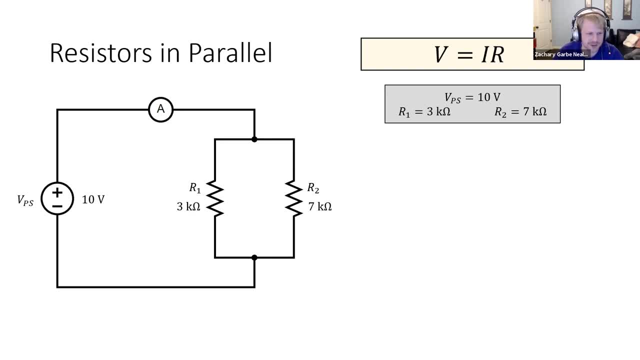 an additional elective to meet my requirements. Okay, So that's available If you're interested in this sort of thing. electrical engineering- there's that class. I would recommend it if you're interested. Like I said, it was kind of difficult. 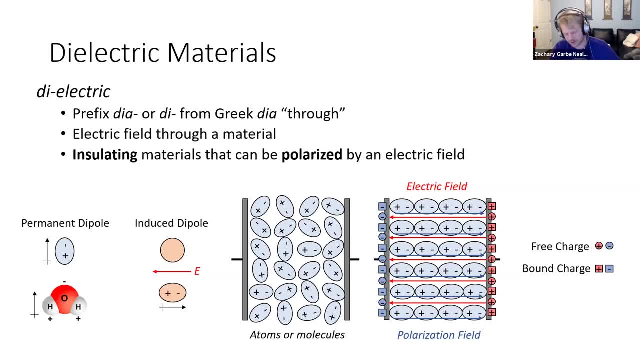 Okay, So now I would like to talk about dielectric materials to wrap this lecture up. We won't be talking, We won't be investigating it in labs, So I want to kind of introduce you to this class of materials. There is a class, senior-level elective class, MSE 452, taught by Dr Chow, which goes into: 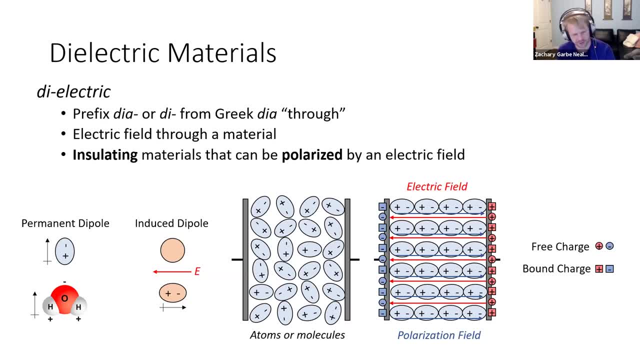 much more detail with dielectric materials and piezoelectric, ferroelectric and also ferromagnetic materials. So if you're interested in this type of thing, I encourage you to enroll in that class. It's during winter quarter, So dielectric materials- let's look at the root of the word. 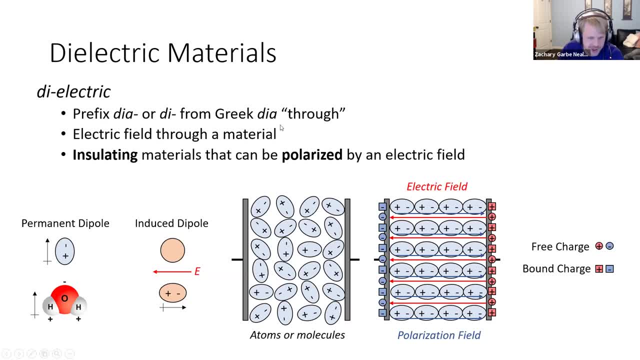 So this time the prefix dia or di is Greek meaning through, So literally it means electricity through a material, But it's kind of not quite electricity. What it should be is electric field, because dielectric materials are insulating materials, So electrons are not going to be passing through these materials. 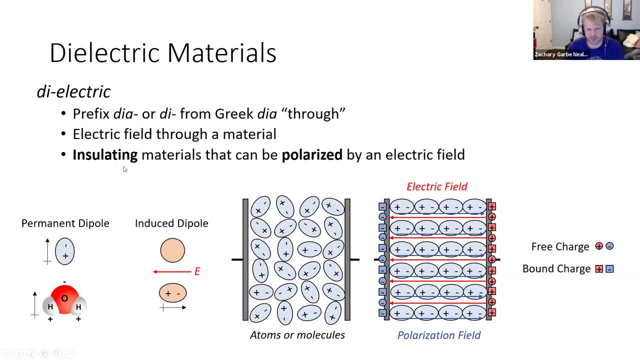 These dielectric materials are insulating materials that are able to be polarized by an electric field. So polarization. there's two different types. I show here a permanent dipole, For example, like water molecule has a permanent dipole. There's an electronegativity difference and one side is more negative than the other side. 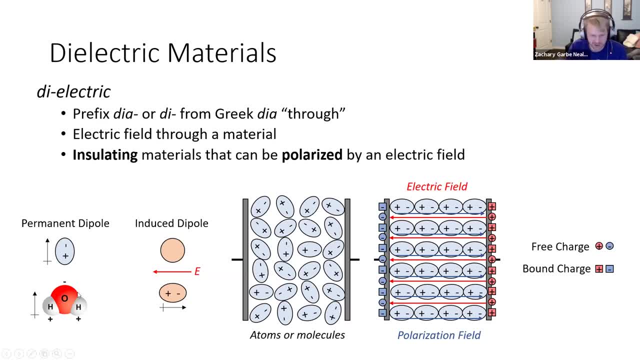 So it can align it. The molecule can align itself with an electric field And then there's an induced dipole. So you can have just a neutral atom with an electron cloud, and if you put an electric field across that atom, the electron cloud will be insulating. 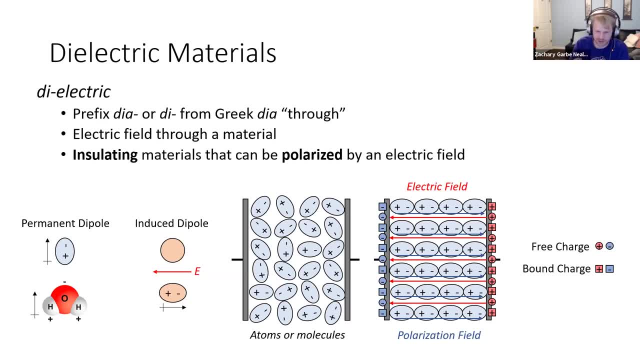 So you can have a neutral atom with an electron cloud and if you put an electric field across that atom, the electron cloud will be insulating. So this will distort And you'll have a side where the nucleus is and a side where there's more density of electron. 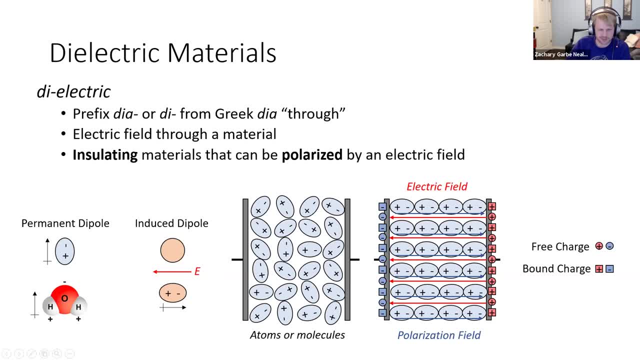 clouds. So that's an induced dipole. So in this example here you have two parallel plates and you have a material between the plates, atoms or molecules. In this example they're just, for example, like water molecules and you can apply an. 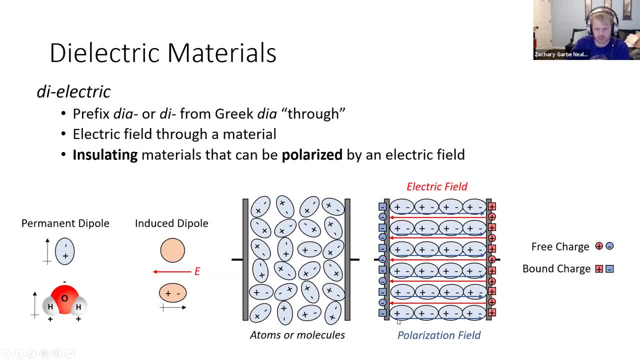 electric field between the two plates and that will polarize the material. So this material is considered the dielectric material, All right, And that will induce what's called a polarization field inside the dielectric and that will accumulate additional charges to the surface. 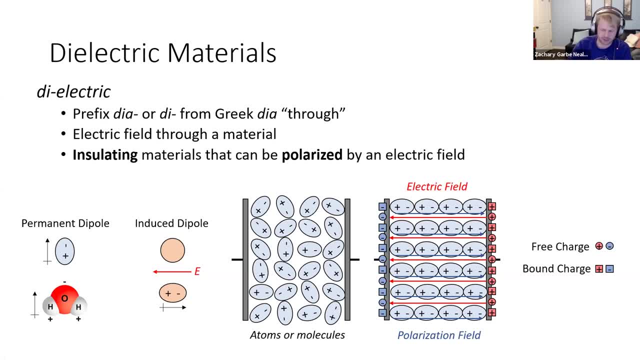 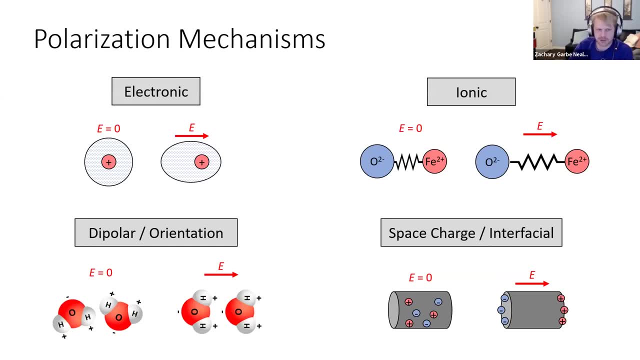 So this is like the basis of a capacitor, is kind of like what I'm showing you right here. So there are four different types of polarization mechanisms in materials. The one I already described is electronic polarization, where you have an atom with an electron cloud. 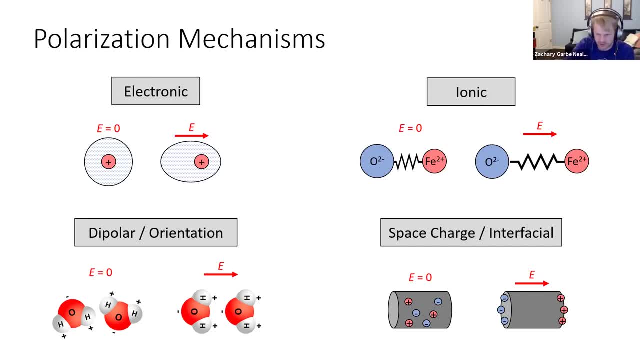 You apply electric field and the proton kind of is attracted to the. is this the right side? Yeah, yeah, the electric field is always positive to negative. So the proton is the nucleus is attracted to, like the negative side of the electric field, and the electrons are pulled to the negative, the positive side. 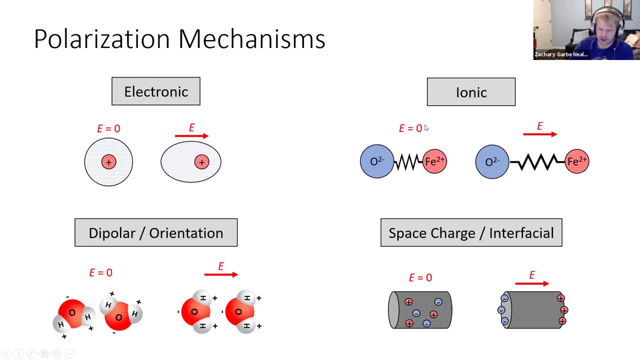 Electronic. and then there's ionic polarization. So ionic, it happens in all ionic solids, For example. this example is iron oxide, FeO, iron 2 plus and oxygen 2 minus, And at rest they have a equilibrium bond distance right. 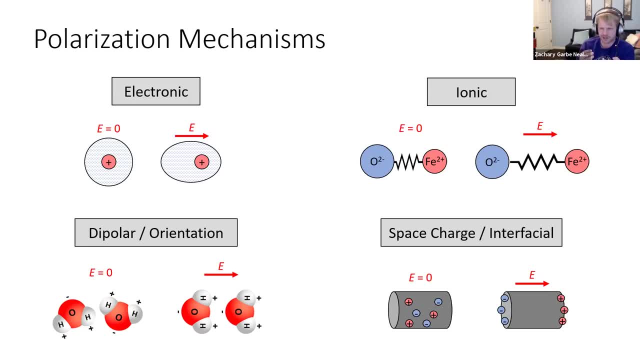 They're a distance at their lowest energy, And if you apply an electric field across the material, then it'll pull the cation, the positive ion, towards the negative side of the electric field and then the anion, the oxygen, towards the other side. 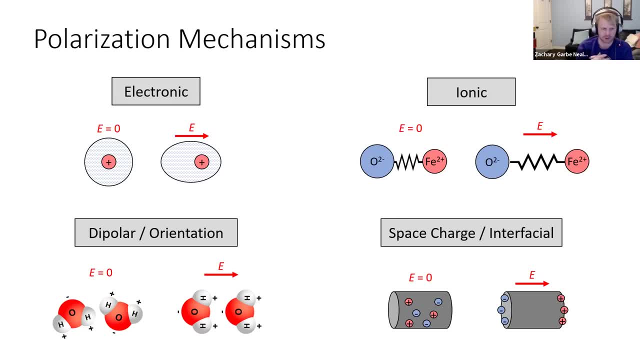 And so you're changing the bond distance, and that's another form of polarization, And then also dipolar, or also called orientation, and I already mentioned this. What if I, A molecule that has a permanent dipole, can orient itself with an electric field? 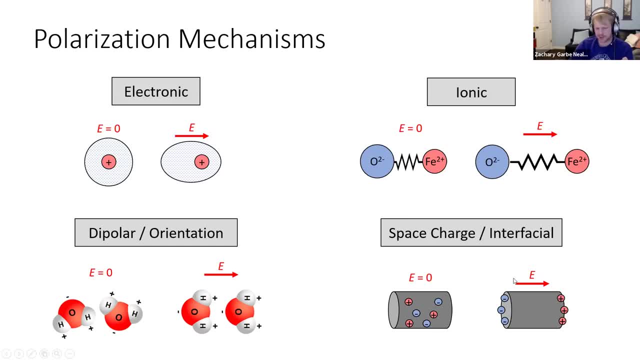 And then last is space charge or interfacial. So this is individual charges in the material that are mobile and they can move or be separated to different sides. So in this example you have a metallic material where you have surface charge on the material and at rest they're equally distributed. 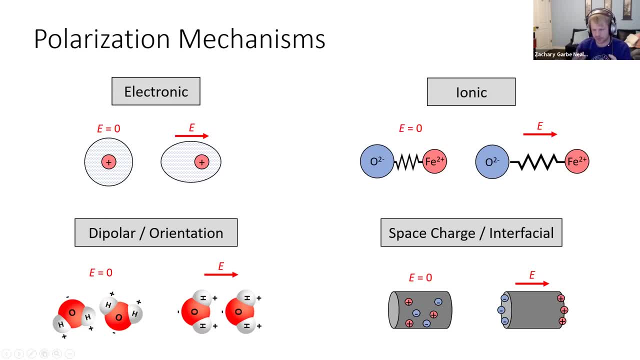 And then, if you apply an electric field, then you'll have a dipolar. And then, if you apply an electric field, then you'll have a dipolar. And then, if you apply an electric field, then you'll have an accumulation of negative charge on one side and positive charge on the other side, just on the surface. 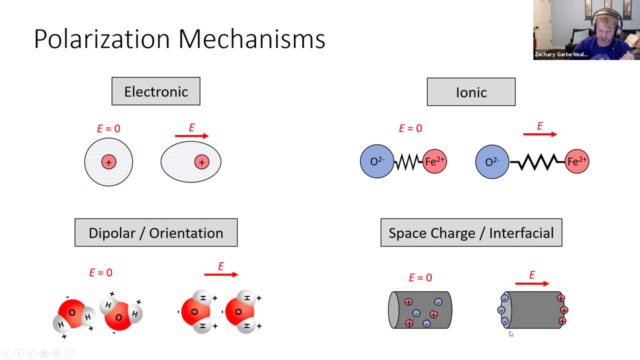 But it doesn't have to be electrons in a conductive material for space charge. It could also be ions like an electrolyte could also undergo space charge polarization, And I think a good example of this, I believe, is electrophoresis, which is used in biology. 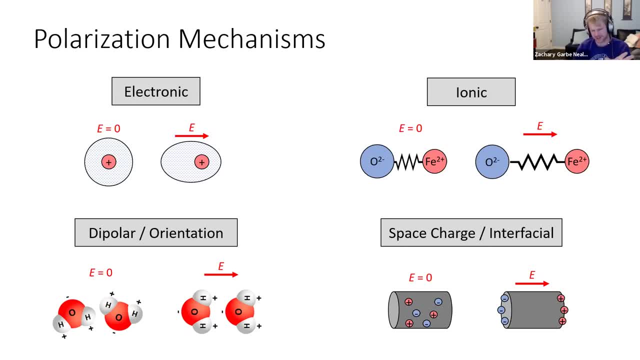 So I'm not too familiar with it. But my understanding is: you know, if you want to separate DNA based on its chain length, you can use gel electrophoresis, where you have like this gel and you have your DNA samples, and I guess they have different dyes or whatever. 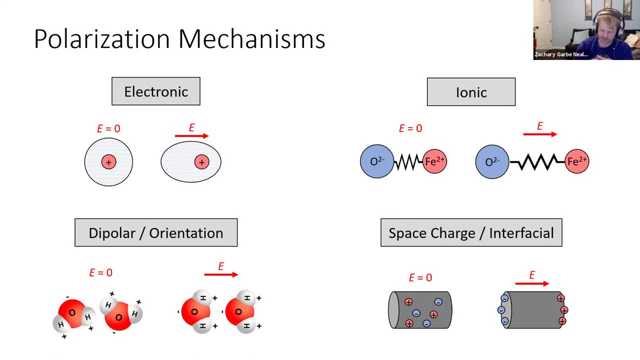 And you have an electric field and these molecules are charged, so they'll be attracted to the electric field and so they'll travel towards the electric field And depending on the size of the molecule, they will travel a certain distance. or, you know, the larger the molecule, the slower it travels. 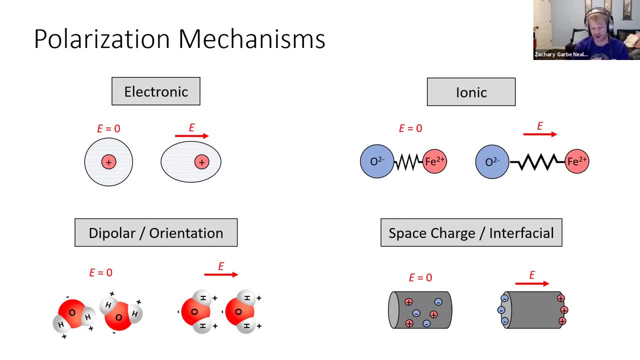 Right. So that's an example of the space charge. polarization is that you're having these ions that are attracted to one side of the gel And based on that you could- based on the distance it travels, you could tell something about the DNA. 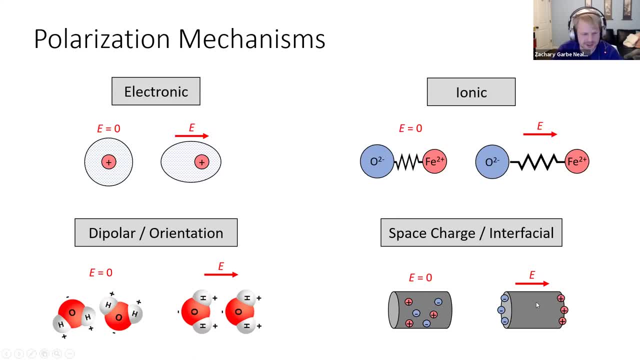 I'm not too sure I'm as familiar with that subject. So that's space charge, electronic ionic dipolar. So you can think of, try to think of some materials that exhibit these different polarization mechanisms And some many materials. 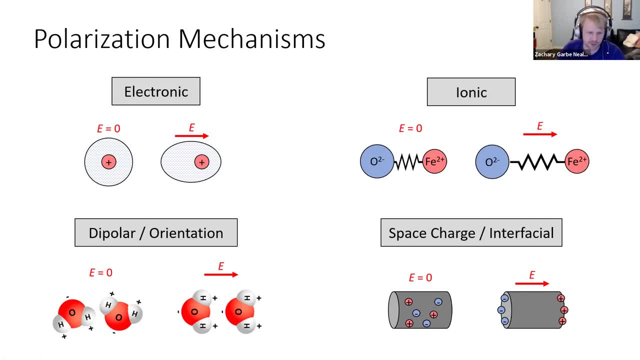 Will exhibit multiple polarization mechanisms, For example, water it has. its biggest mechanism is the dipolar mechanism, but it also has ionic polarization, right? I mean you would many people consider oxygen and hydrogen a covalent bond, which is correct, but you still have a positive charge and a mostly negative charge. 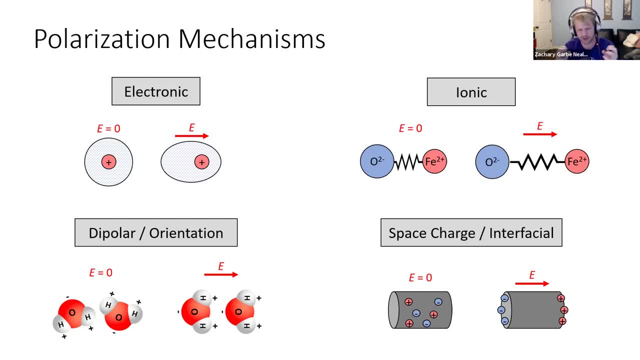 And so you could consider that the bond length, the bond length of oxygen and hydrogen, will also change in an electric field, not just the molecule itself, but also the bond length, And that will contribute. It won't be the dominant contribution, but it will definitely contribute. 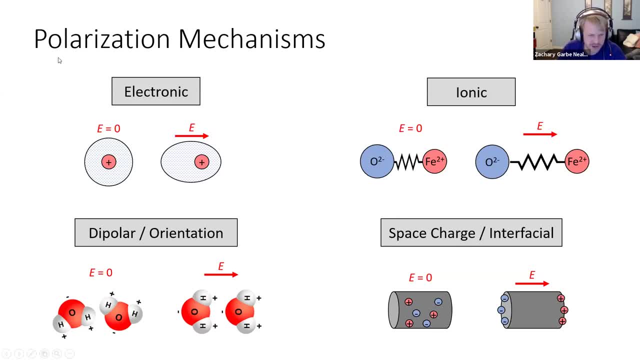 So can anyone think of a material? Well, let me, let me first say that all materials, all materials that contain electrons, have electronic polarization. right, It's guaranteed. If you, if you have atoms and you have electrons, you're going to have electronic polarization. 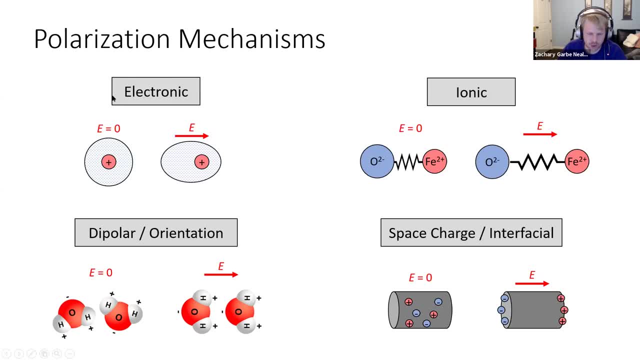 But can you, can anyone think of a material, A material that only has electronic polarization and none of the other polarization mechanisms? I'll give a couple hints. One: one material is a pure element, is one material. So, Jordan, you say material or atom? 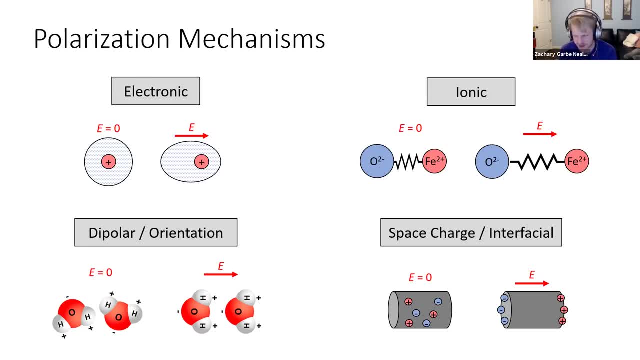 Yeah, it could be. a pure element is definitely. there's some examples of that, And then there's also some molecules that are examples, some fairly very common molecules: Hydrogen, So hydrogen gas, H2, for example. Yeah, that would exhibit only electronic because there's no, there's no electrical negativity difference between the two molecules of a hydrogen. 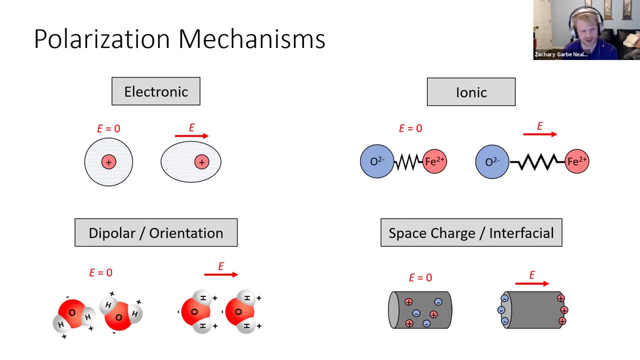 I was also thinking Nitrogen gas is the more common one, So you only have electronic. Another example would be the, the non-metal elements like silicon or germanium, that don't have any free electrons And so they don't have any ionic polarization. 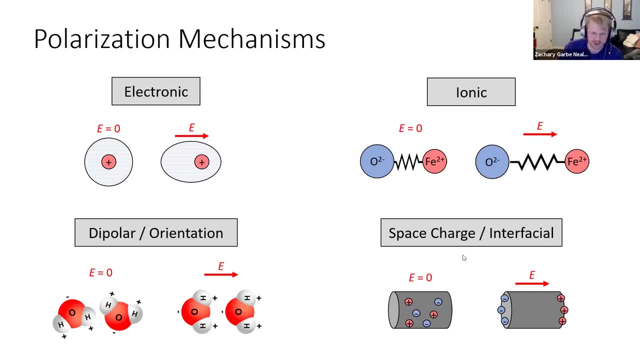 They don't have. ideally they don't have any space charge. polarization: no dipolar, They only have electronic. But if you had a metal like any of the metals that do have conductive electrons, then they would also have a space charge. 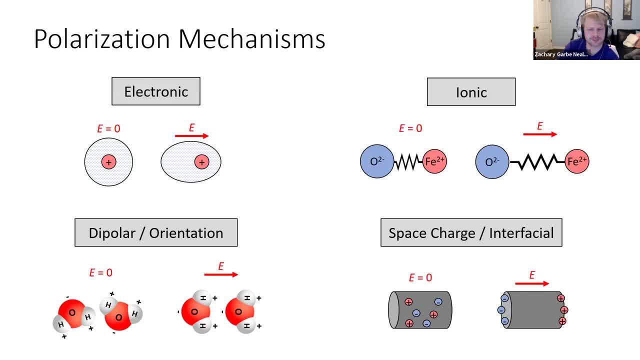 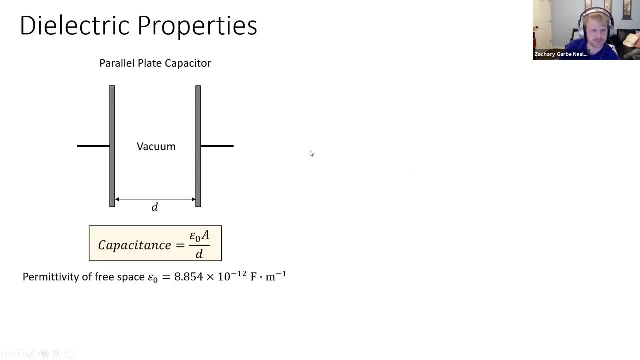 space charge, polarization. Okay, so let's move on to. so here's an example of a some dielectric properties. In this example we have a capacitor. This is a parallel plate capacitor and it's an ideal capacitor where there's just a vacuum in between two plates, Excuse me. So the capacitance. 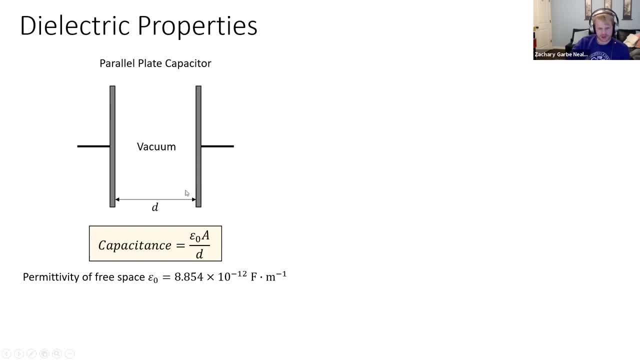 of these two parallel plates is a function of the area of the, the area of the plate divided by the distance of the plate, and there's a constant involved called the permittivity of free space. This epsilon naught is permittivity of free space It has. in this case, the f is a farad, not faraday. 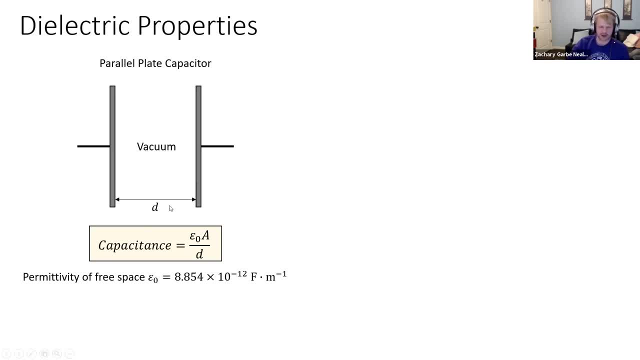 It's farads per meter is the unit, of capacitance is the farad. So it doesn't matter. capacitance doesn't depend on the voltage that you apply. Capacitance is a proper, a device property of this, of the capacitor. It doesn't depend on the voltage. So if we increase the area of these plates, 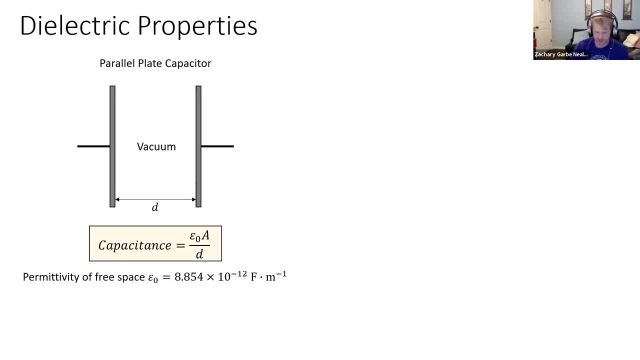 you're increasing the capacitance, or if you decrease the distance between the plates, you increase the capacitance. All right, and capacitance, if we apply electric potential between the two plates and we generate electric field between the two plates, then we start. 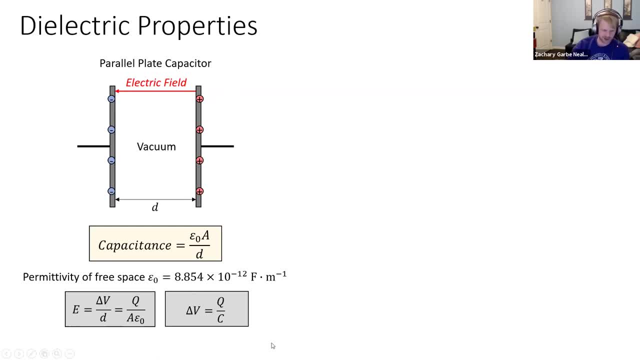 accumulating a certain amount of charge on the plate. All right, and so that's when voltage does come into account. So the the voltage for a given voltage across the plates, you'll accumulate a certain amount of charge on those plates, and that is related to the capacitance. So if you have a 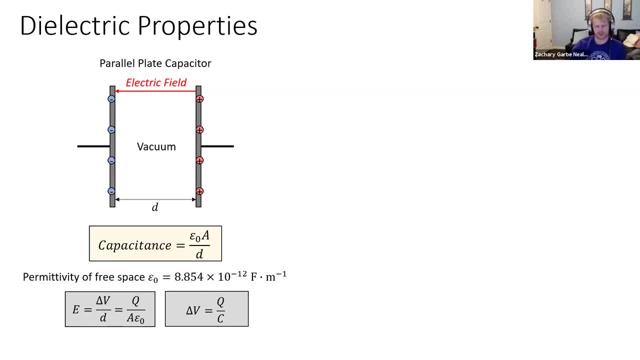 capacitor with higher capacitance for a given voltage, you'll have more charge on the plate. Okay, So now let's say we take the same parallel plate configuration and we insert a material, a material that's insulating. So this is our dielectric material. It's an insulating material and we apply the electric 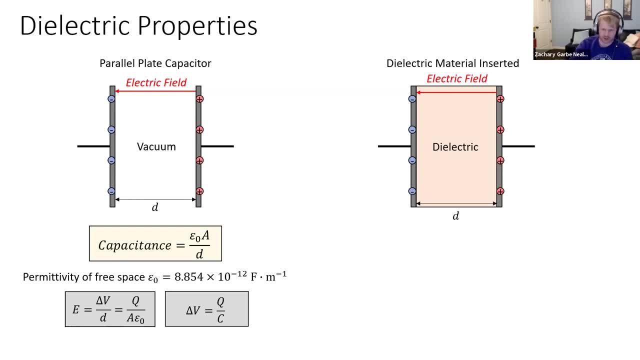 field across the plate. again, If it's a dielectric material, it becomes polarized and, like I said before, it creates this polarization field in the opposite direction. All right, and this brings more charge to the surface. So we have two types of charges at the surface. So just by inserting a 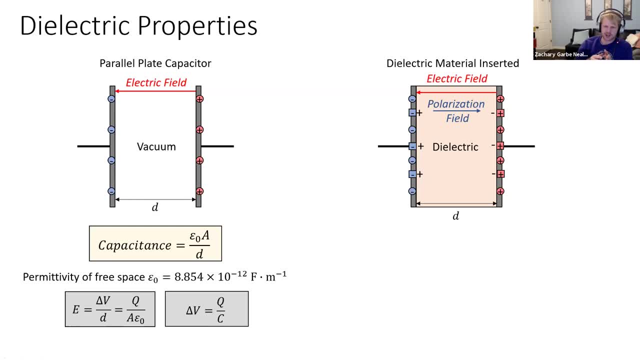 material, a dielectric material. between the two plates we generate a certain amount of charge. So for a given voltage between these two plates, we're increasing Q, We're increasing the amount of charge at the surface. So for a given voltage, for the same voltage across the plates, with a. 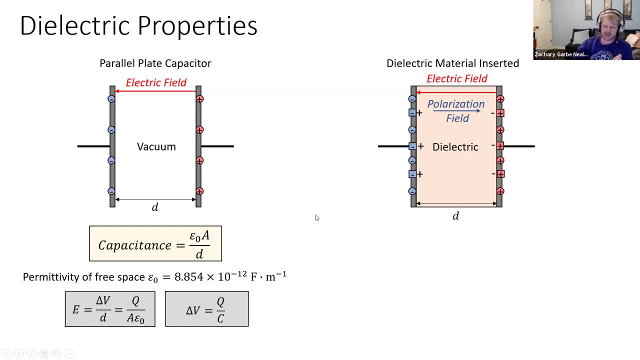 dielectric, we have more charge, which also means the capacity of this capacitor. excuse me, not capacity. I always I mix these up. You need to differentiate capacity from capacitance. The capacitance of this dielectric, of this capacitor, is higher when we, if we, just put a material in. 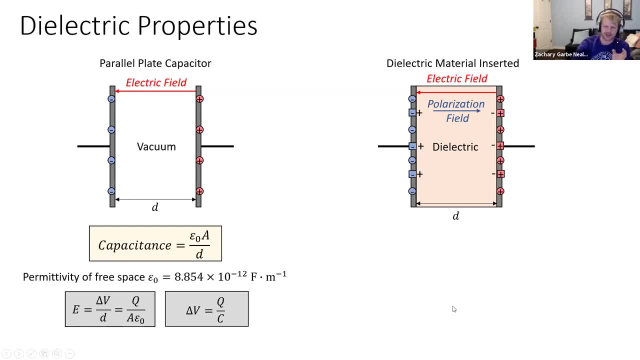 between the two plates compared to vacuum. Okay. and the amount of the amount or the increase in capacity, capacitance due to the dielectric, or I should say rather, the ratio of the capacitance with the dielectric compared to the capacitance without the dielectric is known as the dielectric. 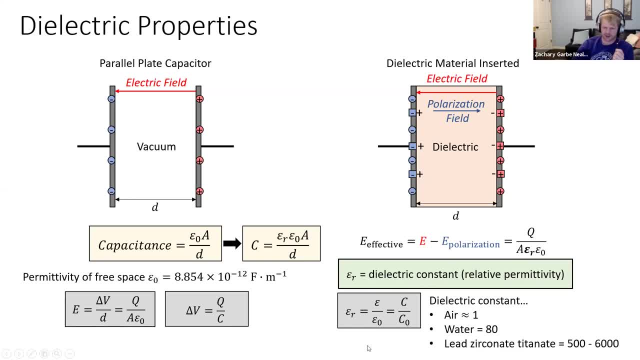 constant. So here's the ratio of capacitance with and without the dielectric. So that ratio is the dielectric constant, also known as a relative permittivity. Okay, and here's some examples of dielectric constant of different materials. For air, air is about one, By definition, vacuum is one. 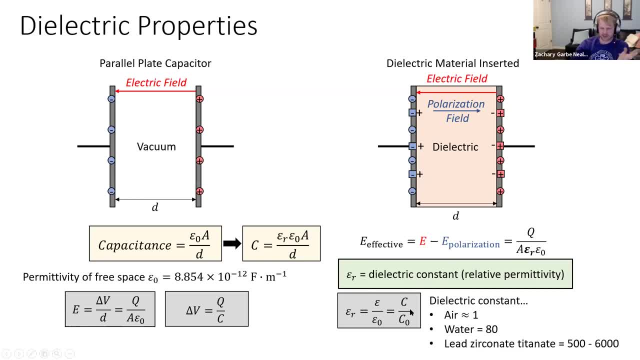 because the you know it would be C naught over. C naught would just be one. Air is more or less. we've got the same permittivity as vacuum, So it's about one. Water, on the other hand, is a bit. 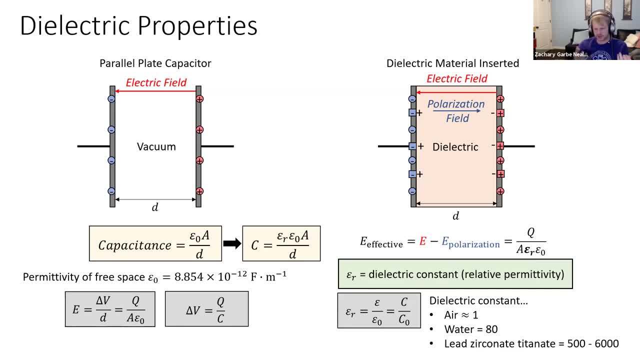 as we know, is a very polar molecule And so it has a much higher dielectric constant of 80. So just by adding water in you're going to increase the capacitance- yeah, capacitance- of your capacitor by 80 times. And then other ionic materials like lead. 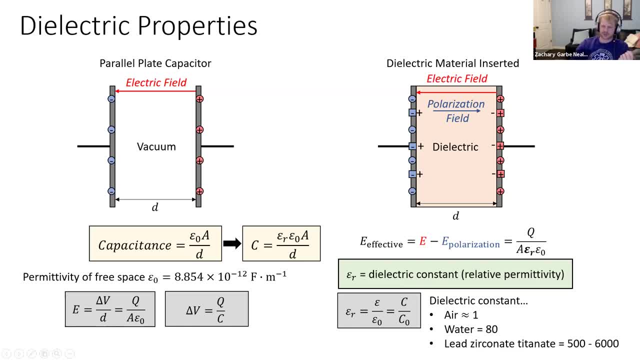 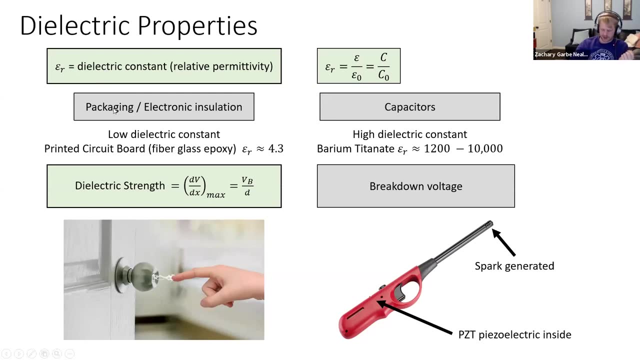 zirconate titanate, or PZT, has much higher dielectric constant- 500 to 6,000, depending on other factors. So some different applications dealing with the dielectric constant. One application of these dielectric materials is packaging or like electronic insulation. 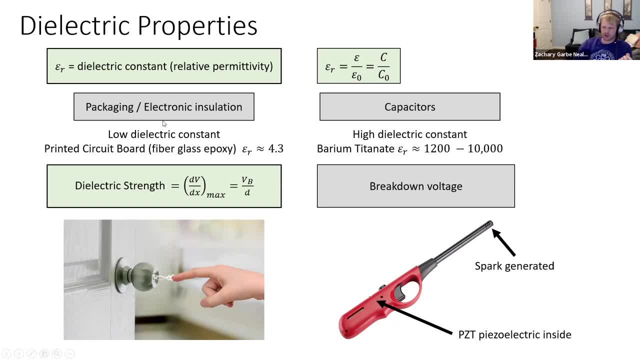 So for these type of materials you want to have a material that has a low dielectric constant, because if you want to isolate two like electric wires, or two electric lines, you know, say you have an integrated circuit and you have two voltage lines and you want to isolate them. 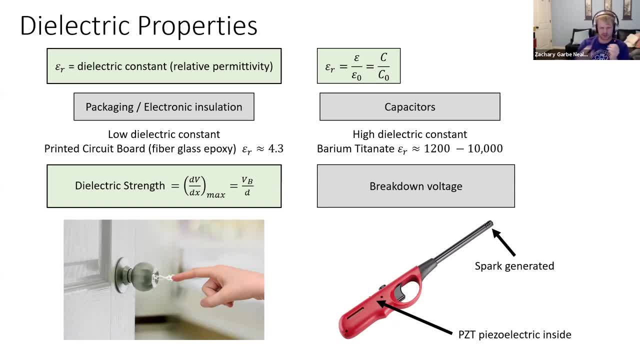 you don't want the charge difference to affect the voltage, So you want to have a low dielectric material, a low dielectric constant. So an example of that is printed circuit board PCB, which is made of a fiberglass composite epoxy and it has a relatively low dielectric constant, around four. On the other hand, for applications 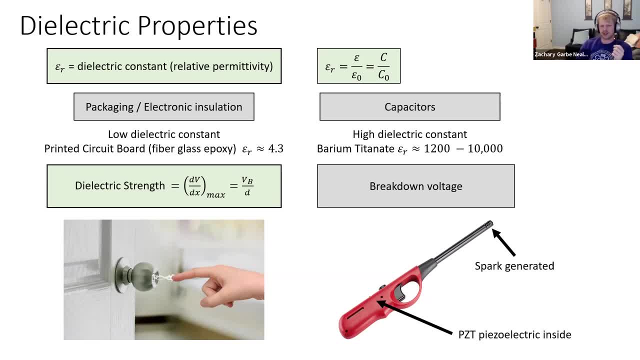 like capacitors, you want to have a high dielectric constant because you want to increase the amount of charge which would be capacitive T, the amount of charge that's accumulated on those surfaces of the capacitor. So an example of a capacitor material with high 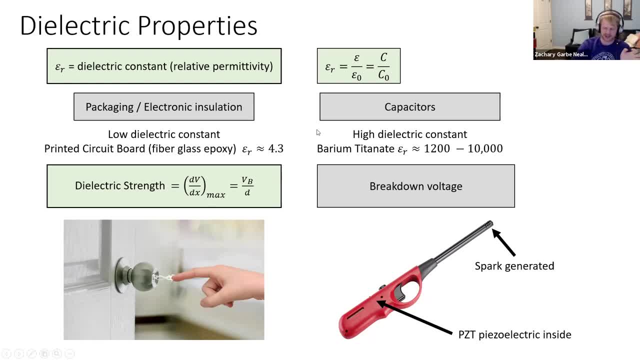 dielectric constant, which is a high dielectric constant, is a high dielectric constant. dielectric constant is barium titanate, very similar to that last material: lead zirconate titanate. The same crystal structure is the perovskite crystal structure. 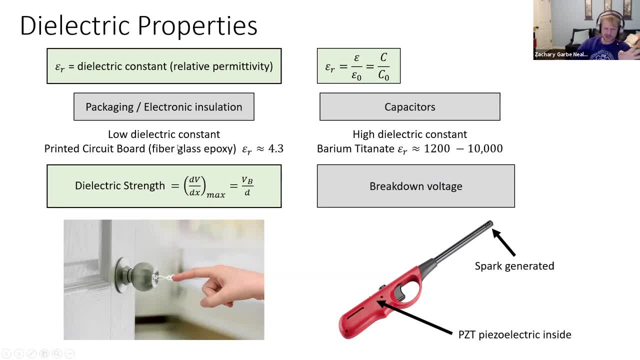 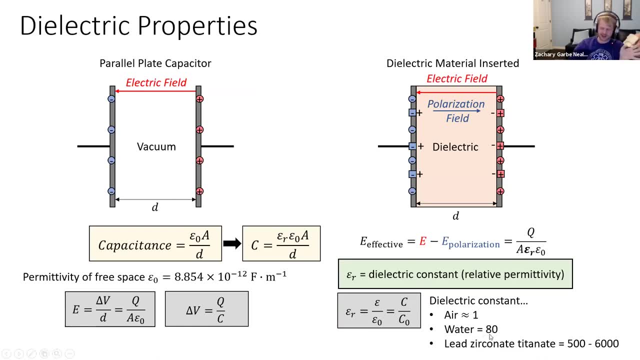 It has a very high dielectric constant. So this is I believe, and I could be wrong, but I believe this is why water is not good for electronics, right, You know, you always know you shouldn't- you shouldn't mix up water with electric circuits, right? But water itself is not. it's an insulating. 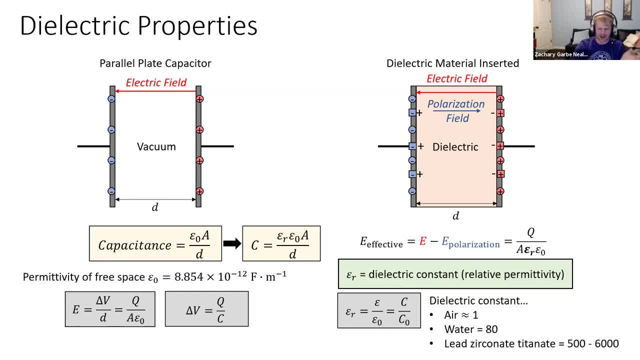 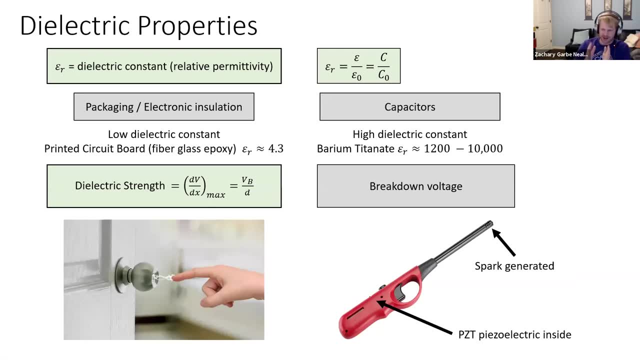 material right. It doesn't conduct electricity very well. It has very high resistance, but because it's polar it has a fairly high dielectric constant, So it acts as a capacitor, like if you're just to put a capacitor between two wires in your circuit. you know that's probably. 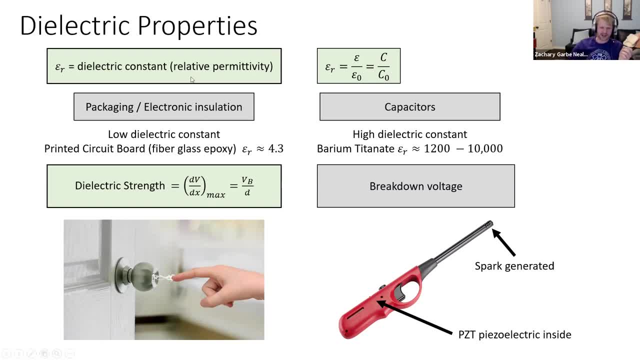 not going to be good for your circuit if you just insert a capacitor, right. So I think that's why water is not a good material. besides other reasons, There's other reasons like if the voltage is high enough, you can break down the water and that causes corrosion and all that. But anyways. 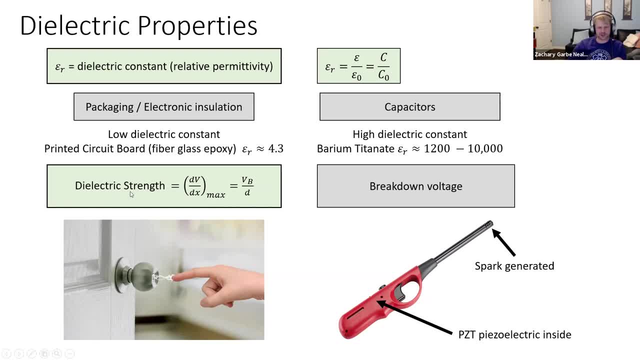 another dielectric property is called dielectric strength. Dielectric strength is the highest voltage you can go for a given distance before you start stripping the electrons out of the material in what you have what's called dielectric breakdown. okay, So imagine you had your parallel. 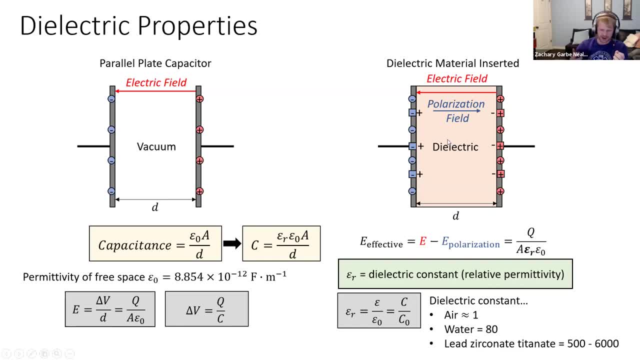 plate capacitor and you increase the voltage very, very high. you, eventually you're going to reach a voltage at this given distance where the electrons are just going to be stripped from the material and you're essentially, essentially you're ionizing the material and your the 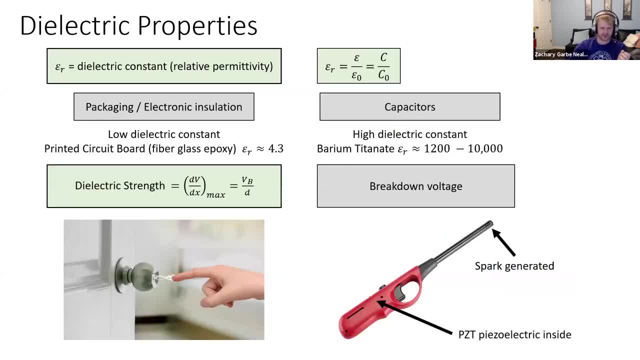 electrons are flowing freely through material like a conductor, So that's dielectric strength. So an example I always like to give is: you know, if you're at your home and you're walking around, you touch the doorknob of a door and you get a spark and you get a shock right. So that's the 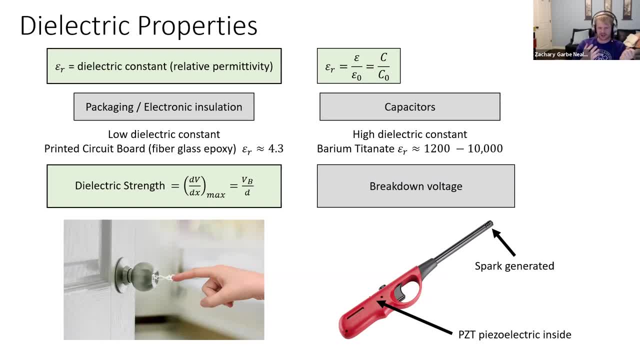 dielectric breakdown of air. right, Your electrons are jumping from your body to the doorknob, or the opposite doorknob to the body, not sure. And it's going, it's traveling through the air. So the electrons in the molecules of air, they're ionizing and they're becoming electrically conductive. So 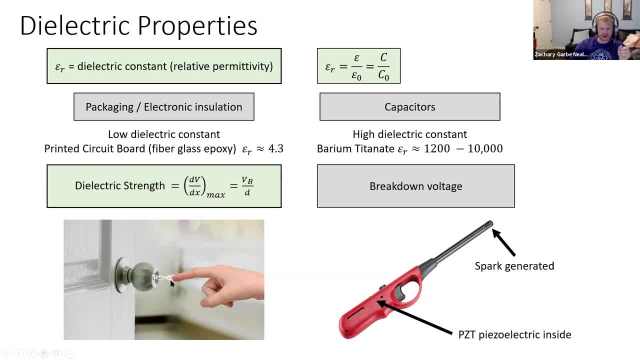 my question is for you guys: how high of a voltage or electric potential difference between you and the doorknob do you think it is for dielectric breakdown to occur? And so, of course, it depends. you know what's this breakdown? voltage is what I'm asking you guys. It depends on the distance. 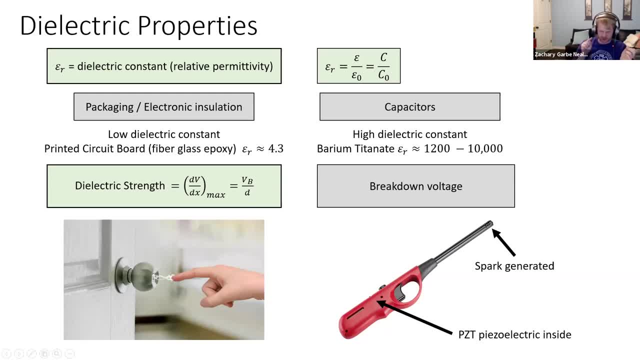 you are. So let's assume you have, you get a spark at one millimeter. You have a spark gap of one millimeter. It's kind of small right. So you make a spark. How? any ideas how high that voltage any? 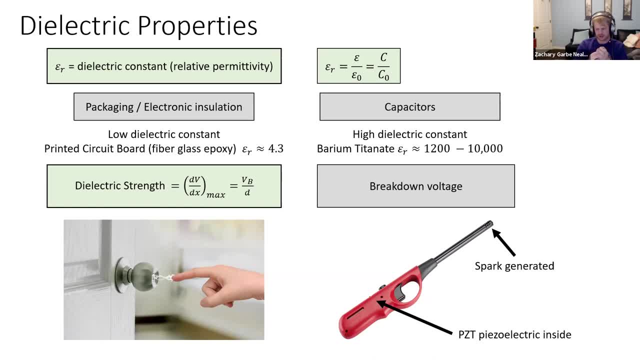 guesses what kind of voltage we're talking about. You know ballpark, ballpark figures Very good. So is it? is it 10 volts? Is it under 10 volts? That under 100 volts? All right. Over 10 volts, 10 volts, All right. All right, I'll move on. So it's, it's quite. 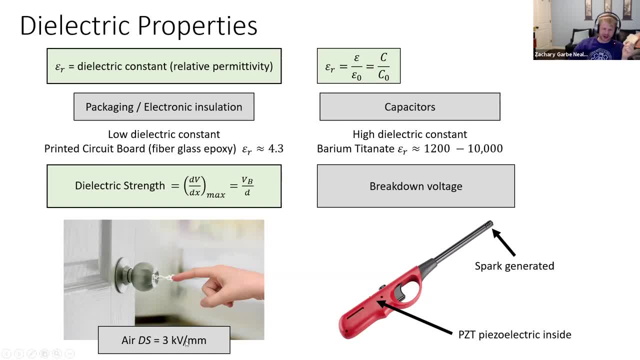 fascinating. The dielectric strength of air is three kilovolts per millimeter. So if you touch the doorknob and there's a spark between you and the doorknob that's one millimeter, The voltage between you and the doorknob is three kilovolts, 3000 volts, So very high, And 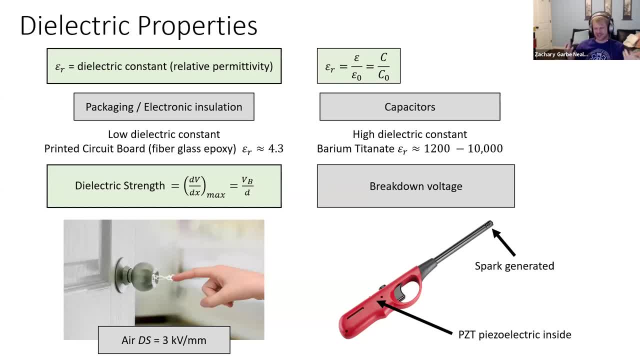 that makes sense because air, air is a- you know it's insulating material right. It takes a lot of potential to strip an electron away from a material right. So 3000 volts per millimeter for air to break down. Okay, So another engineering application of dielectric breakdown. 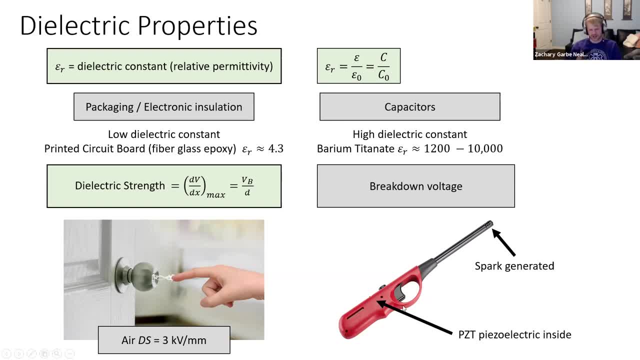 and dielectric materials is like a lighter, a gas lighter like this. So you know, when you click the lighter there's a material inside the lighter that generates a potential high enough to make a spark at the tip to ignite the fuel. And so, again, you know if you have one millimeter spark. 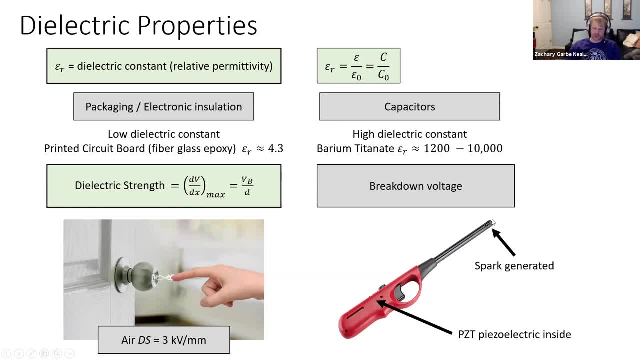 you're generating thousands of volts potential. And so there's a device, there's a material inside this, this starter, and it's not. it's not like there's no battery, right, There's just a material that's by itself, it's passive. 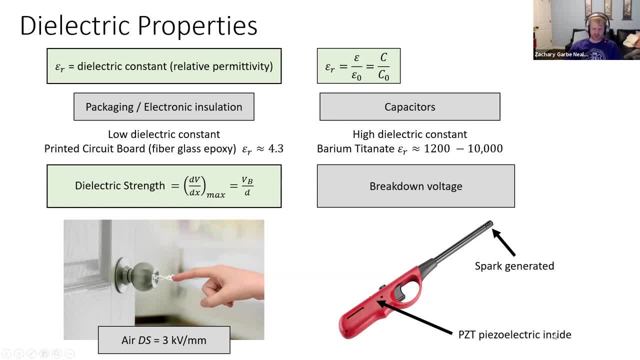 And that material is called a piezoelectric material, And we'll talk about that And specifically, I believe the piezo. I could be wrong, though. I think it's PZT, but I could. I could be wrong. Actually it might be quartz, So we'll move on. So piezoelectrics and also. 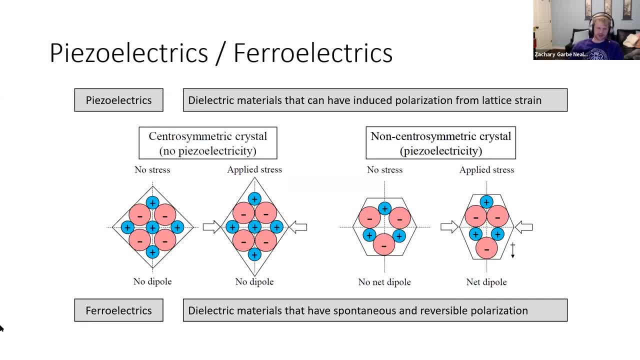 ferroelectrics are dielectric materials, And so what's special about piezoelectrics is that if we apply a strength or a strain or a stress on the material, if we squeeze the material, we distort the crystal structure in such a way that we induce a polarization in the crystal, Or in other words, 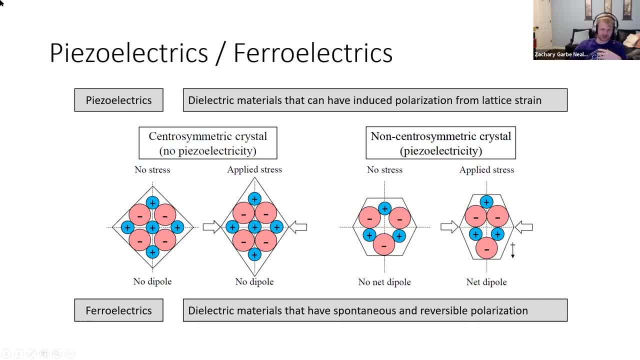 we're generating an electric field across the crystal. Okay, There's a. there's a requirement: in order for a material, in order for a crystal to be piezoelectric, to have piezoelectric properties, it has to have the following symmetry: It has to be non-sensual. 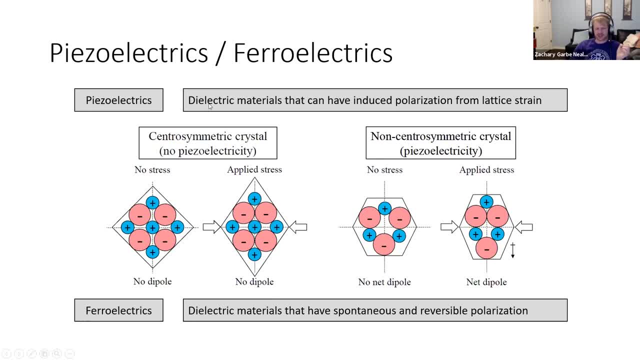 it has to have non-centrosymmetric symmetry, Where centrosymmetric symmetry means that the crystal has an inversion center. Inversion center is a type of symmetry where if we took one point on the crystal, like the unit cell, and we were to draw a line through the center into the opposite, 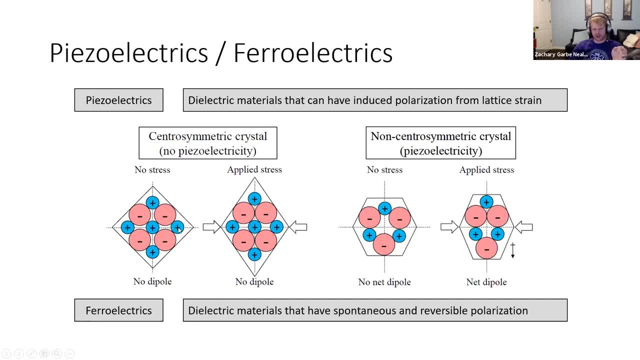 side the exact opposite. does the point on the opposite side? is it the same as the point that you started with? If it's the same, then it's the opposite side. So if we took one point on the same, it means you have an inversion center, And if it has an inversion center, it means you. 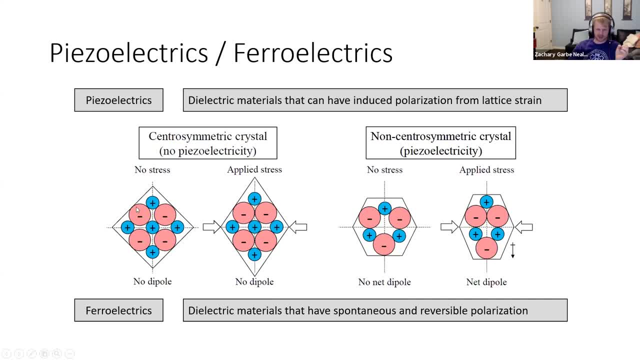 have centrosymmetric symmetry. So in this example I just demonstrate. you know you take a point here- you go through the center, you end up on the exact opposite side. it's exactly the same ion, for example. So it's centrosymmetric In a non-centrosymmetric crystal symmetry. 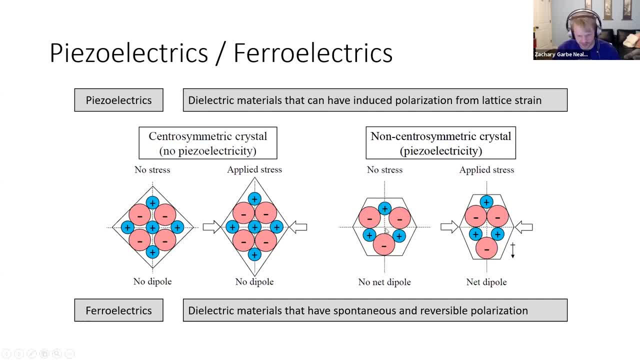 if you take a point, you go through the center of the unit cell, go to the opposite side, and it's not the same like in this example here it's non-centrosymmetric. And so how does that? how does that give us piezoelectricity? Well, in a centrosymmetric crystal, if we apply a stress. 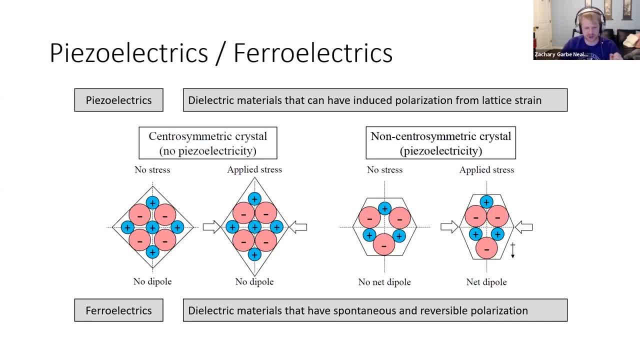 we distort, we distort the crystal. and if we distort it there's no net change in the dipoles. right, There's dipoles between the anions and cations, but they're all. they all cancel out, right? But in non-centrosymmetric crystal, if you apply a stress and we distort the crystal, 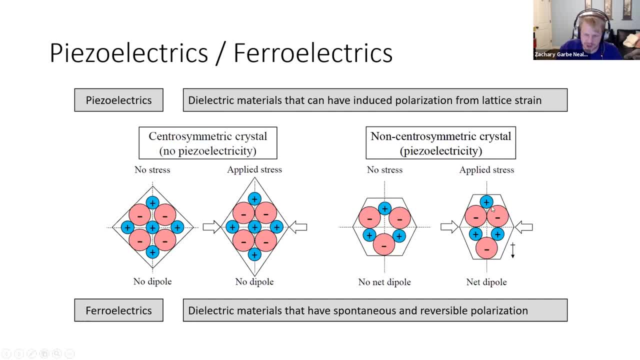 one side of the crystal is going to have a net accumulation of positive charge and the other side might have a net accumulation of negative charge, and that's going to induce a dipole or polarization. all right, So in piezoelectric, 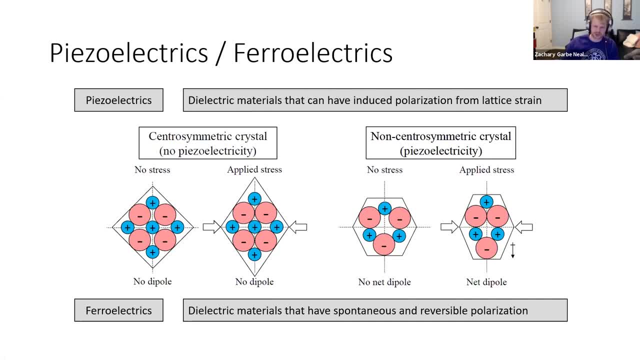 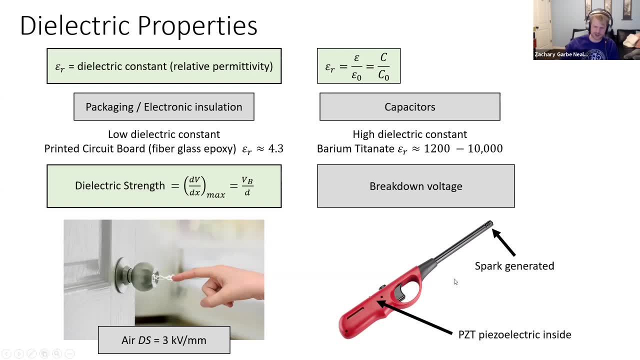 materials, you can generate very high voltages and in this example, high enough voltages to generate a spark, so that's thousands of volts, just by applying a stress on it. So in this device, the clicker, when you click it, there's a striker that strikes. 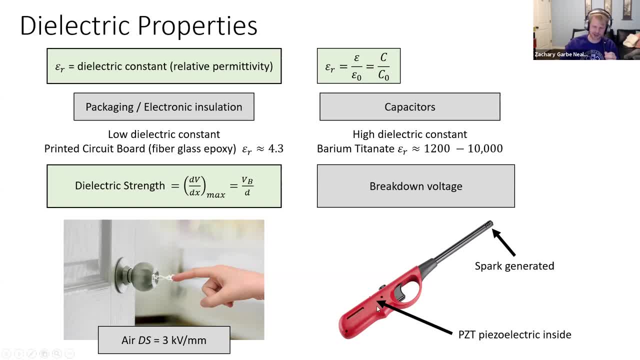 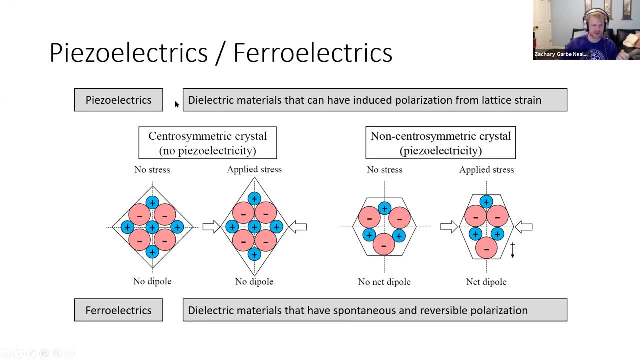 the piezoelectric material, the piezoelectric crystal, inside here, and it strikes it so hard. there's so much strain on the crystal that it generates thousands of volts to make the spark. That's a piezoelectric material, and so this is an example of applying a mechanical stress. 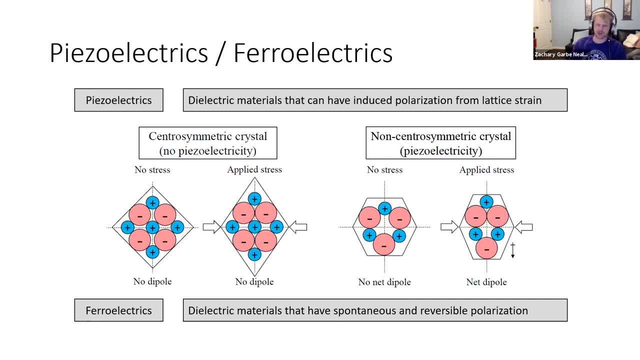 to induce a polarization. You can do the opposite. You can induce or you can give it an electric field. you can polarize the material, put an electric field across, and that will induce a deformation, so it'll distort the lattice and so the dimension of the material will change. 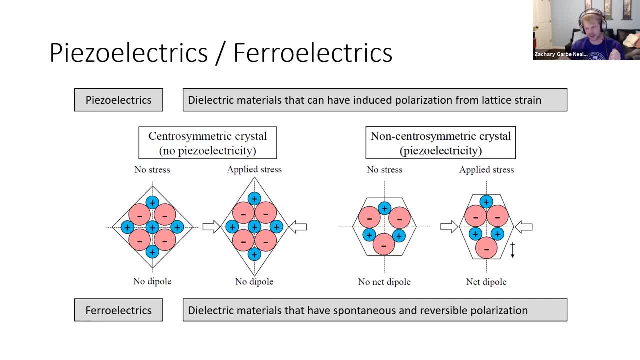 all right. And now let's suppose you have an alternating electric field. so the electric field's going one way and another way and it's switching, and then what happens to the crystal is that it's going to get bigger and smaller, bigger and smaller, right, Because of the 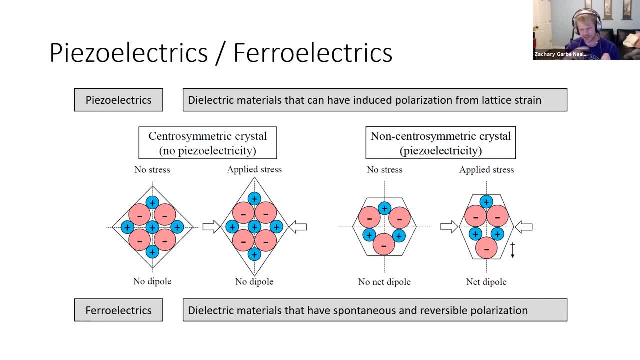 piezoelectric effect and if it vibrates and if the electric field is at a certain frequency and its frequency is at an audible frequency- happens, is that your piezoelectric crystal will generate sound So little tiny buzzers in little. 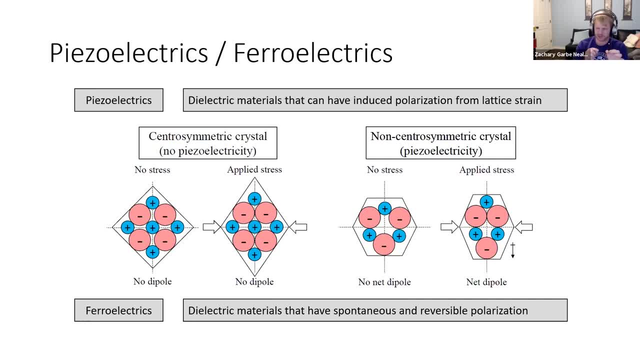 microelectronic devices typically are piezoelectric speakers that will, you know, make it make a noise. Or, for an example, this is: you know, if you, if you ever get one of those birthday cards that make like have a sound or like a noise, usually, sometimes it's a piezoelectric speaker. 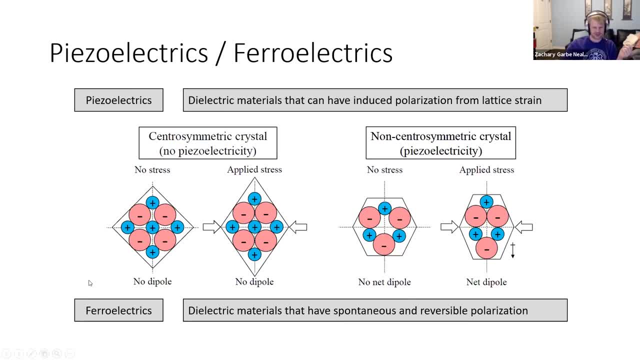 that's making the song or whatever. Okay, And then going back to the original. another example of piezoelectric device is a microphone. So in many microphones there is a piezoelectric crystal and the sound waves that we produce create vibrations on the material and it changes its. 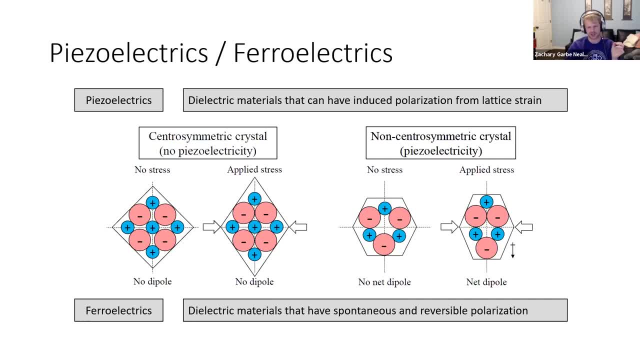 dimension very slightly, And that sends a signal, an electric signal that can be transduced into a digital. So microphones use a piezoelectric material as well. All right, So now let's talk about ferroelectrics, And this will be the last thing we talk about Ferroelectric materials, by definition. 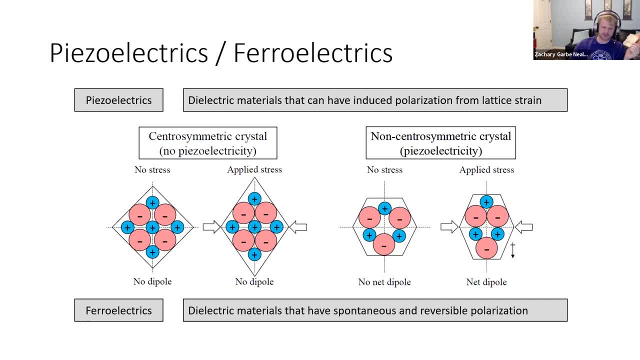 are also piezoelectric materials. Okay, That means that they have to have non-centrosymmetric symmetry, But it's not necessarily that all piezoelectric materials are ferroelectric materials. The definition is that they have spontaneous polarization, So even without, with no stress or 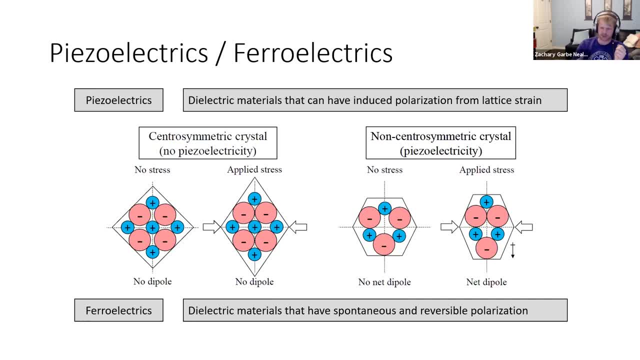 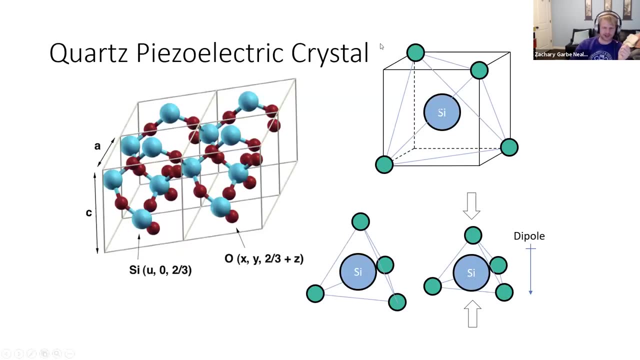 strain on the material, they already exhibit a permanent dipole in the crystal And then also by definition, they can reverse the direction of that dipole. So that's a ferroelectric. Oh, I missed the slide, Sorry. To go back to piezoelectrics, here's an example. 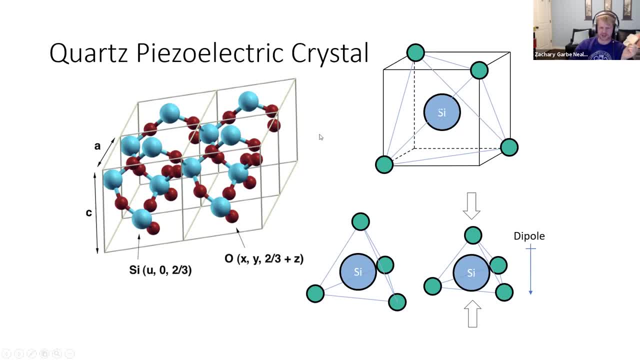 This is a piezoelectric crystal. This is quartz or silicon oxide, SiO2.. So silicon is tetrahedrally coordinated to oxygen. Again, you could argue that silicon and oxygen make covalent bonds, But in reality it's probably 50-50 covalent ionic bonding. So you would say that you know there is. 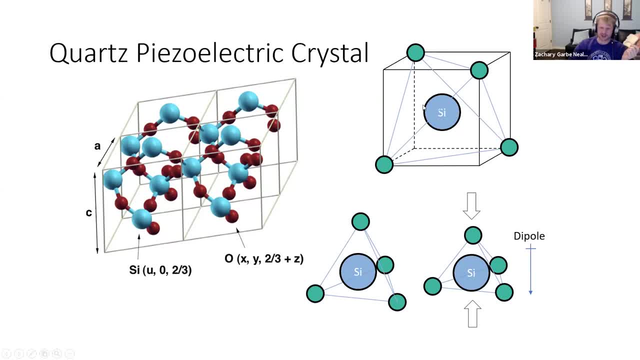 a ionic polarization between these bonds And because it's this has a lot of covalent bonds, it's not always the case. So it's not always the case. So if we look at the piezoelectric crystal, if we look at the piezoelectric crystal, it has this tetrahedral coordination. If we look at the 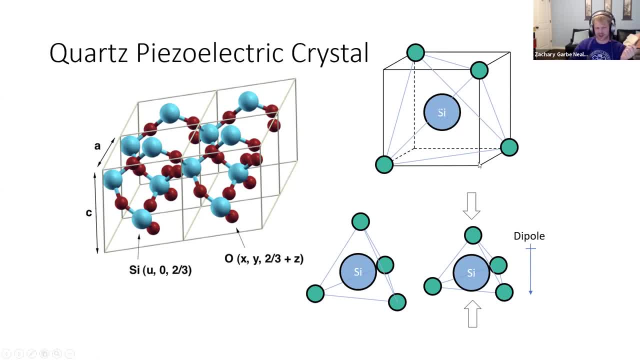 crystal symmetry. there is no inversion center. So if we take this point on the top left here, go through the center into the opposite corner, it's not the same point. So it's noncentrosymmetric, which means it's a piezoelectric material. If we apply a stress on the material, we're going to push the. 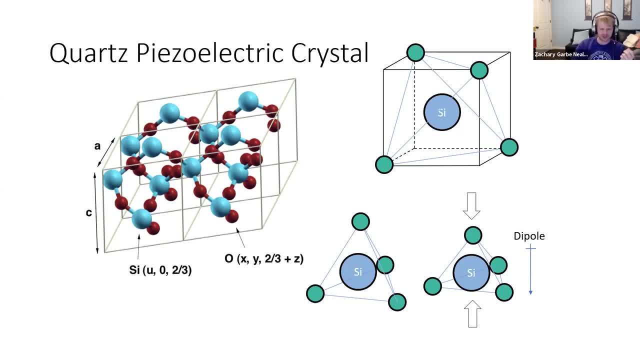 negative charge to one side more than the positive charge and that induces a dipole. So quartz is a piezoelectric crystal And it's used in a bunch of different applications I can't think of. I know it's used like in radio. 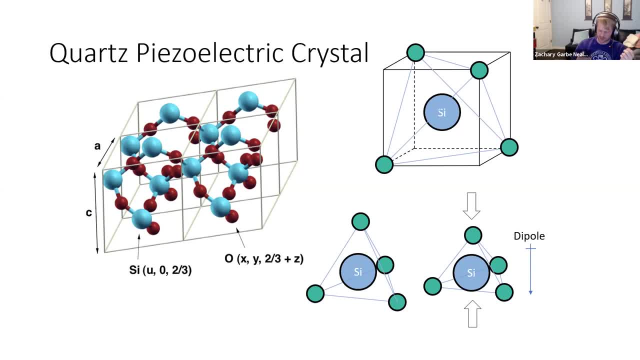 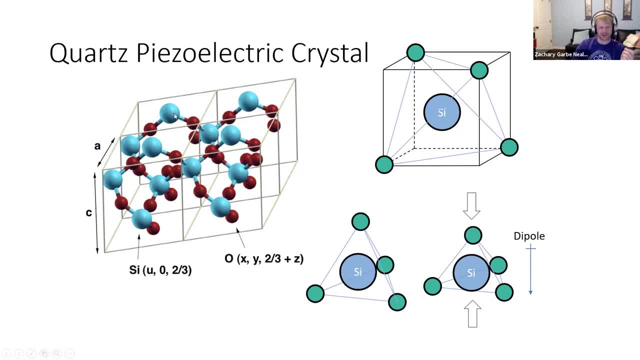 I'm really not sure, but I know it's used in that way. Also related to this, I know that we've used quartz piezoelectrics to measure the mass of something. I've given this example before where, when I was an intern at Toyota Technical Center, I did sputter. 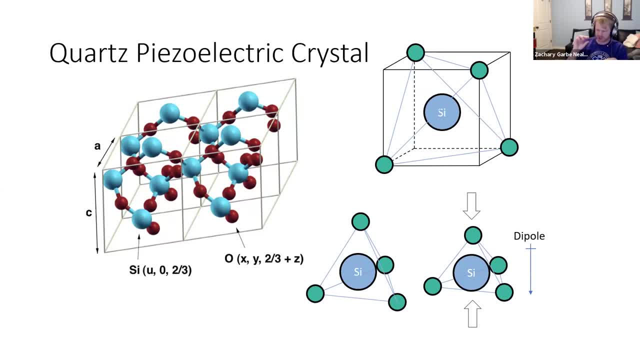 coding and we had a sputter coder that had a quartz piezoelectric which would weigh the mass of whatever target you were sputtering onto. And so, as you were adding, as you were depositing atoms to the surface of your target, the quartz piezoelectric could measure the dimension change. 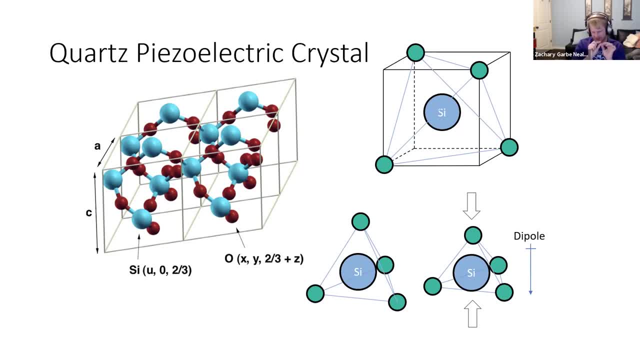 because of the force of the atoms, And we're just, we're talking about, you know, a nanometer thick layer of atoms and it could tell you the thickness of the film based on the weight change because of the piezoelectric signal from the quartz. All right, so back to ferroelectrics. 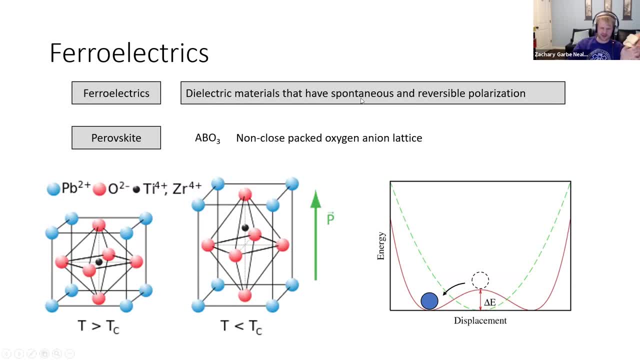 Again, ferroelectrics exhibit by definition a spontaneous polarization, and that spontaneous polarization is reversible. Okay, so a very common example of ferroelectrics is perovskite crystal structure Perovskites. they have the ABO3 chemical formula. A common perovskite is known as PZT. 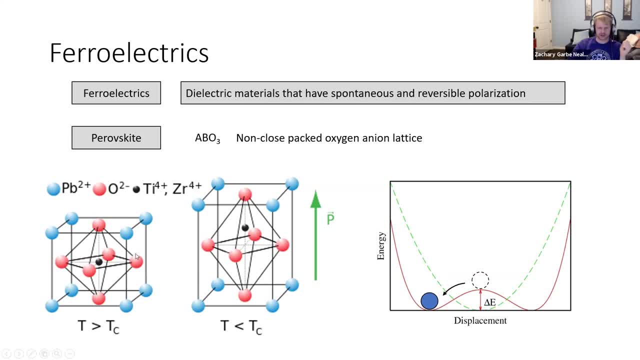 which is lead, zirconate, titanate. All right, so the crystal structure itself has a non-closed packed oxygen lattice. where you have this, this oxygen lattice is in the octahedral configuration and the central ion is either titanium or zirconium, and then on the corners is the lead, two plus. 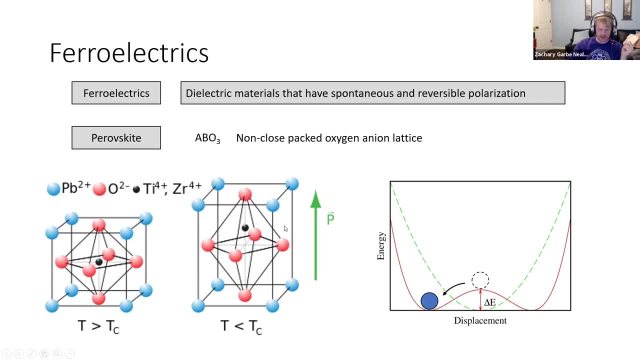 very large ion lead, two plus Okay, and at there's a certain temperature where the phase of the perovskite crystal structure will be cubic and that's above what's called the Curie temperature, And remember, if it's cubic. 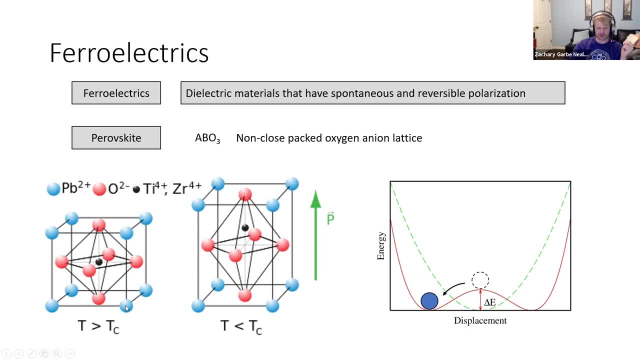 we take a look at the symmetry. this cubic crystal structure has an inversion center and it is centrosymmetric. So at this temperature and this phase this material is not a piezoelectric and is not a ferroelectric. but below that temperature there's a phase transformation into the tetragonal. 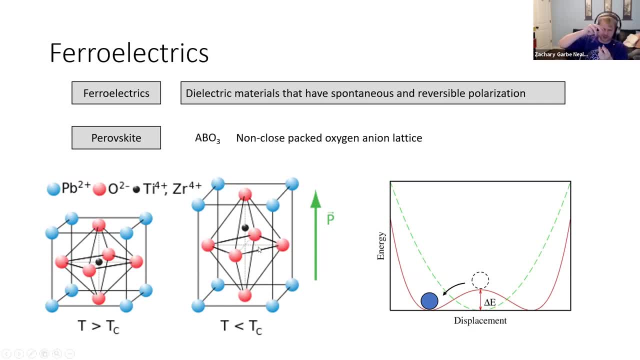 phase, And so tetragonal. you know, you take your cubic, the two phases, and you you pull them apart. You're pulling apart the poles of this octahedral. you're distorting this octahedral, this oxygen. You're pulling apart the poles of this octahedral. you're distorting this octahedral, this oxygen. 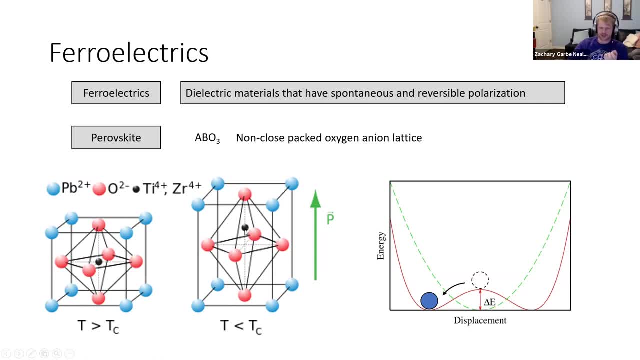 octahedral. All right. and what happens is that the central ion, the titanium or zirconium, is no longer energetically favorable to be right in the center. And here's an energy versus displacement diagram. The dashed line is the cubic phase. so for the ion to be right in the center, 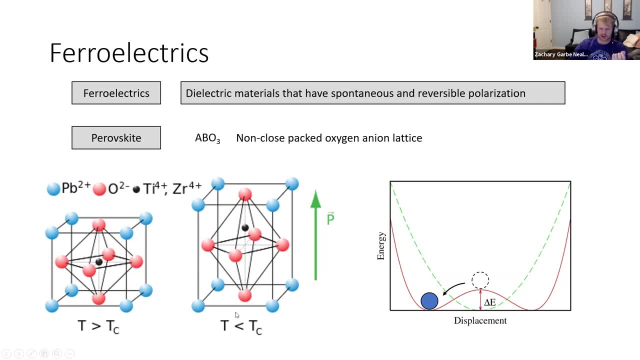 is most energetically favorable. but then the solid line is when it forms into the tetragonal phase and it's no longer energetically favorable to be right in the center of the- you know- the unit cell. So it becomes displaced, it goes offset, either to the top or the bottom, it doesn't matter. 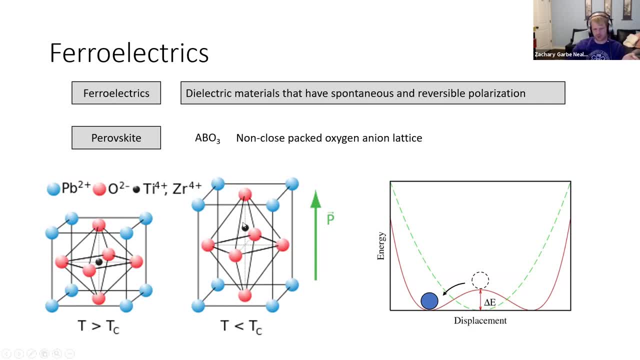 And so when it becomes displaced, then you see that you have more positive ions on the top half of this unit cell than you do have in the bottom half. So you have this induced polarization, this spontaneous polarization, right, and so that fits the definition of the one part of the ferroelectric. 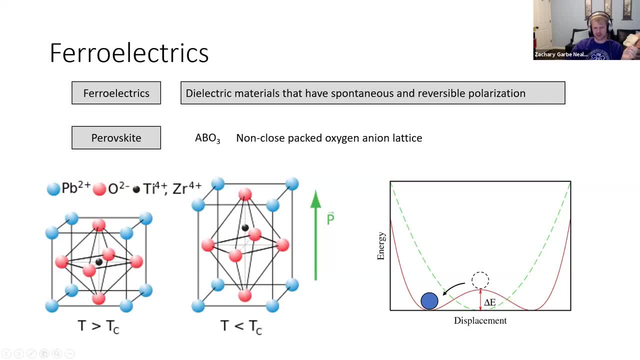 And the other part. the other definition is that it's reversible, So you can apply a strong electric field that will force this ion onto the other side of the unit cell. So you can. you can reverse the polarization direction, but that requires a very strong electric field. So as long as that electric 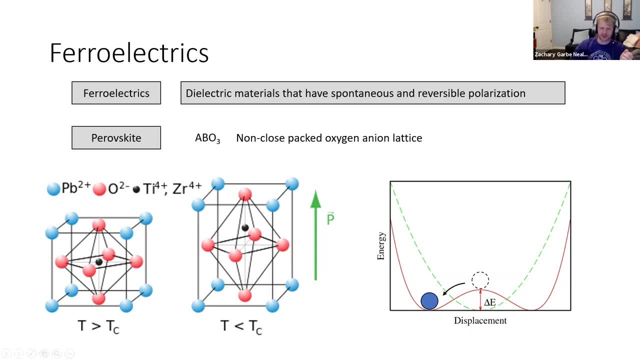 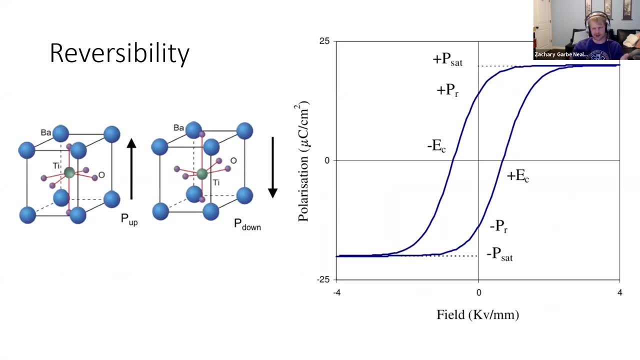 field is lower than the dielectric breakdown of the material, then it could be considered a ferroelectric. If it's not, if it's not lower, if it has dielectric breakdown, then it's called a pyroelectric, but that's. that's more or less the same. So a common characterization of these ferroelectrics is the: 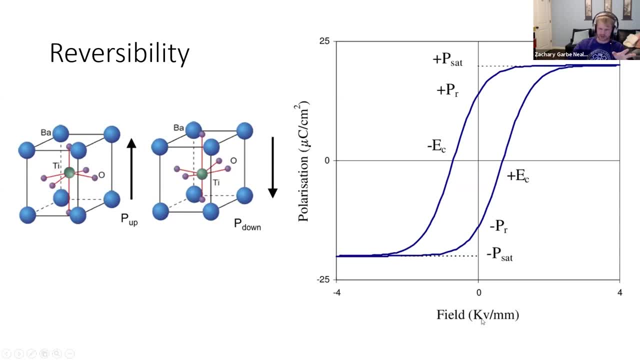 polarization versus electric field. So we're in this characterization: you apply an electric field across the material and you're able to measure the polarization, the spontaneous polarization or induced polarization, of that unit cell. And so you see here, at zero electric field, 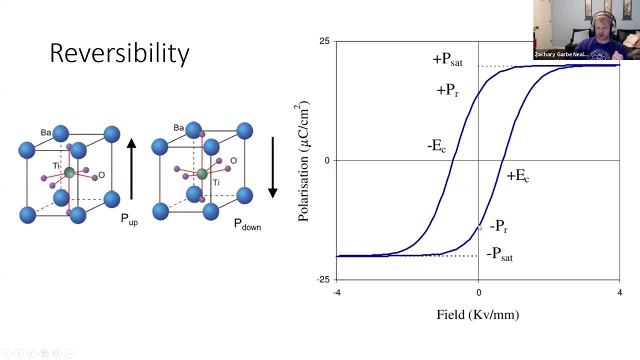 you'll have a non-zero polarization, which is that spontaneous polarization, And it can be either positive or negative. And if you shift the electric field to negative direction past a course of electric field, you'll be able to flip the ion to the other side. And then if you relax it back to zero, then it has the reversed. 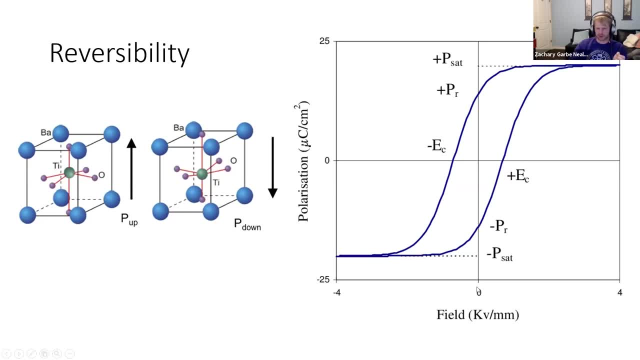 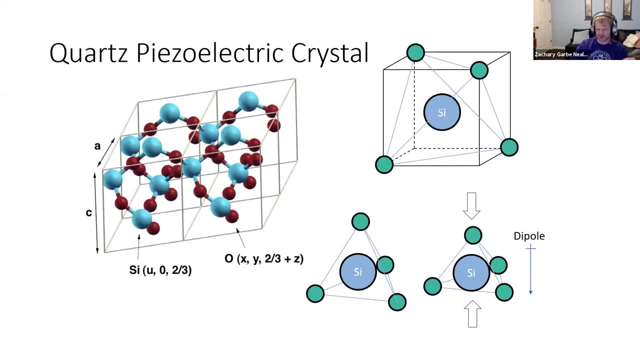 polarization, spontaneous polarization at zero applied electric field, And then of course you can reverse that as well. So that's the definition of the ferroelectric, which is also a piezoelectric, and those have different applications in you know, different engineering applications, So any 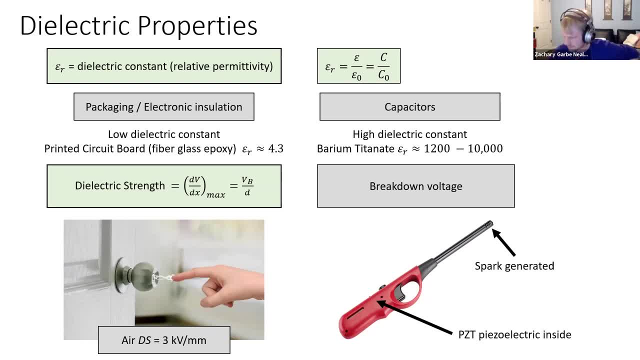 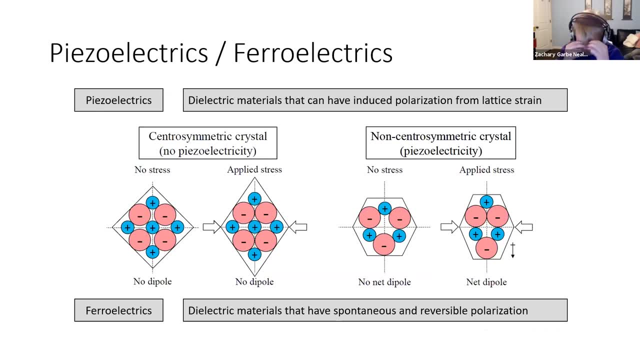 questions about dielectric Dielectrics or piezoelectrics. Oh so so someone mentioned watches. Yeah, Yeah, Quartz, quartz are used in watches. Yeah, Like I said, I think it has to do with the timing. 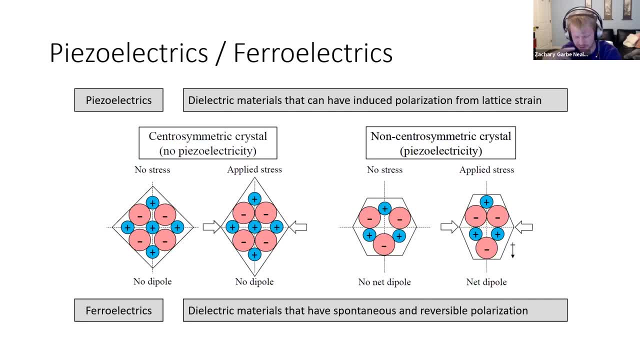 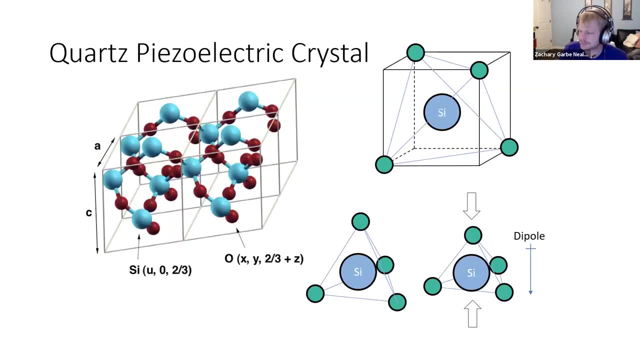 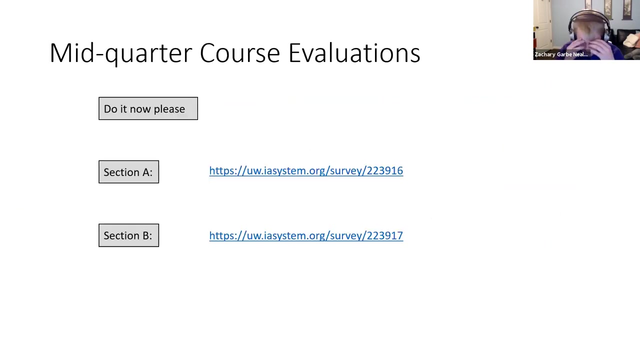 The harmonics, the harmonic symbol signal. if you get the right frequency, something in electronics makes it keep count of the time. I forget. I don't know the specifics. Okay, If there's no questions, what I would like you guys to do, the department has set up some. 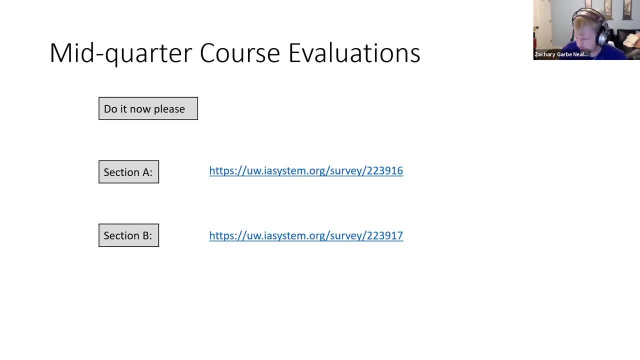 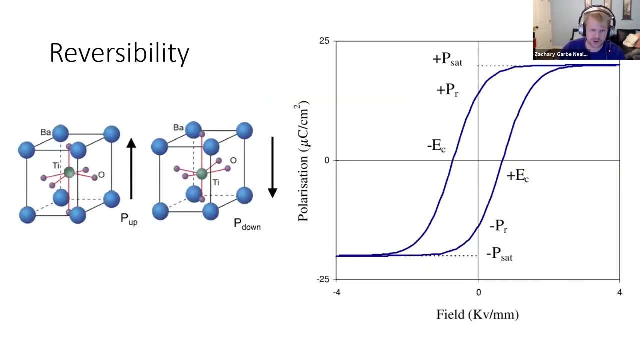 mid-quarter course evaluations. We would like to get some of your feedback. Oh, there's a question: What would be a ferroelectric material at room temperature? Oh well, PZT. most of these are ferroelectric at room temperature, The Curie temperature, and it depends on the material. 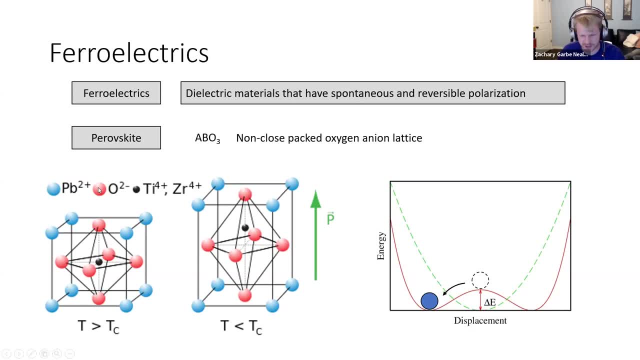 the Curie temperature for a lot of these materials, like lead, zirconinate titanate, I think barium titanate is another one. It's quite high, It's like above 100 degrees, I believe. So most of these are ferroelectric And there's actually more phases than tetragonal. 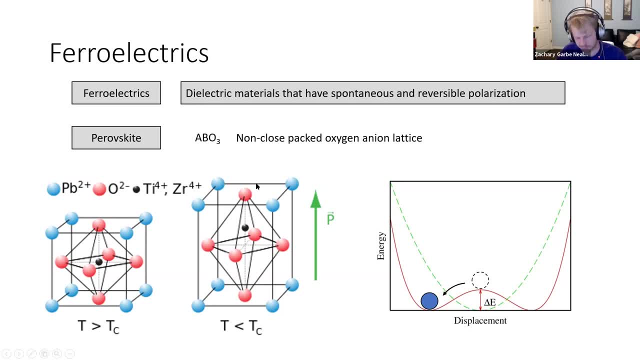 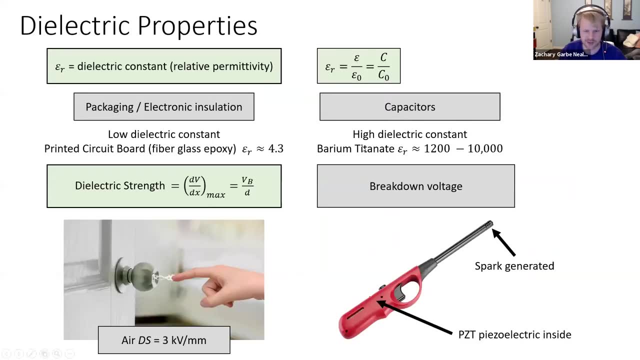 The lower the temperature goes, this distorts even more the orthorhombic and then the monoclinic, And that actually also increases the dielectric constant. I think I had an example. Yeah, Barium titanate has a very high dielectric constant And one of the reasons is because of this, you know. 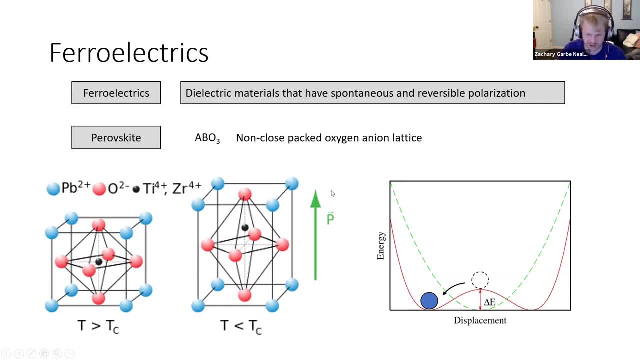 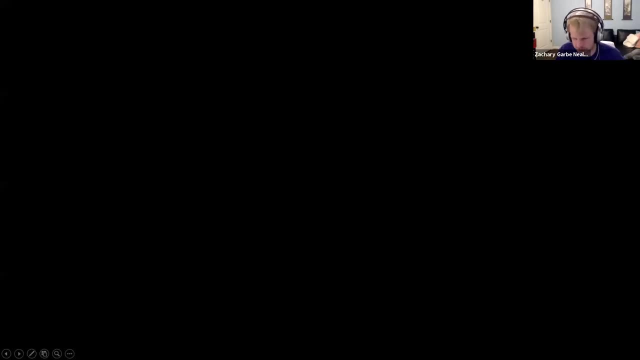 first is the non-closed packed oxygen anion lattice. So it allows this central ion to move around a lot, And if you can move it around, you have higher polarization. Okay, So what I'd like you to do is to- and I will let me put this, I will give you the link: 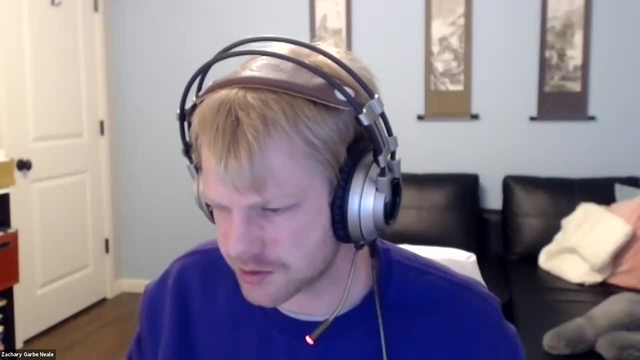 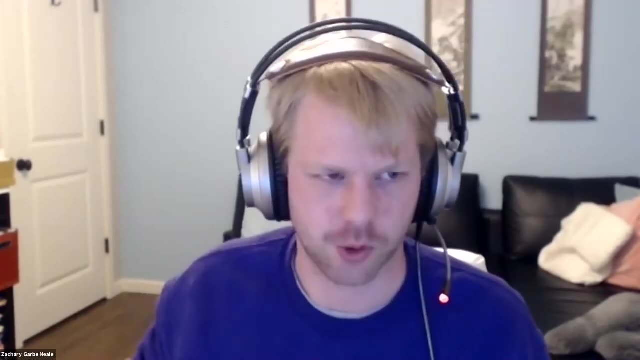 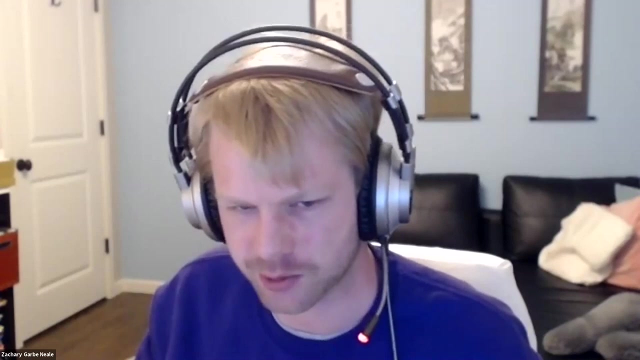 I would like you guys to spend the rest of the class to fill out the course evaluation For your lab summaries. don't worry about making it organized, Just submit your notes, And instead I would like you to spend the time on the course evaluation. midterm course evaluation.